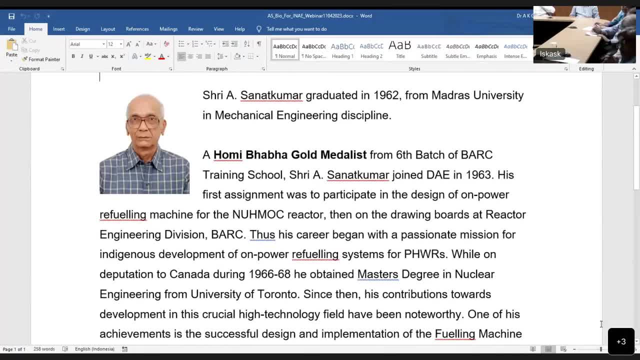 studies, experimental photoelastic models, then followed by strain gauging of the actual machine. when it was ready It was hydro tested in central workshop and Shri Sanath Kumar gave very good advices, guidance not only on the fueling machine but also on the fueling 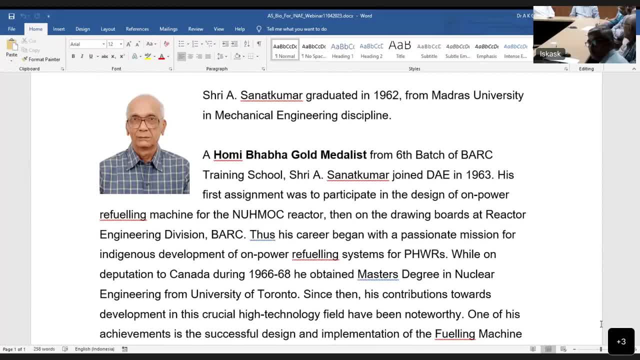 machine design aspects What he was looking for. I hope we will be able to listen from him and, as such, for the general audience, I would like to inform that this fueling machine is very, very complex. It involves multidisciplinary approach. It has all the components of the 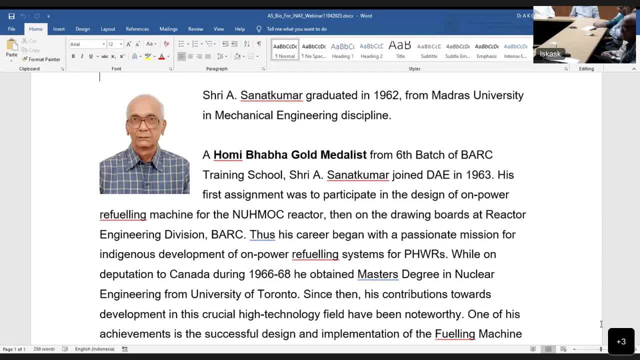 mechanical, electrical, electronics, robotics, control system and all put together in one simple machine, which is fueling machine, And with this fueling machine head development, we have the success story of the PHWR program and this online refueling is very important. 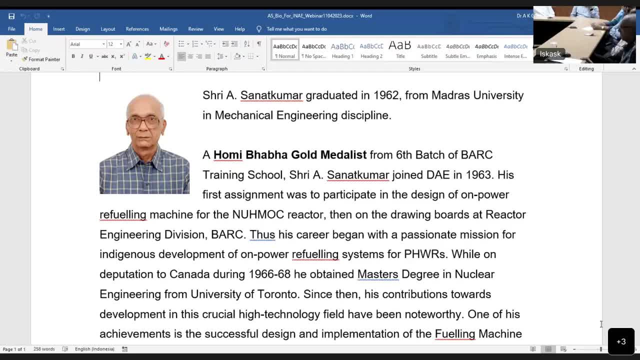 for our fueling machines and particularly this 900 plus day performance of this, which is world record and has been achieved in many of the Indian power plants, PHWR plants. They have been achieved with this and additional features are that this fueling machine has: 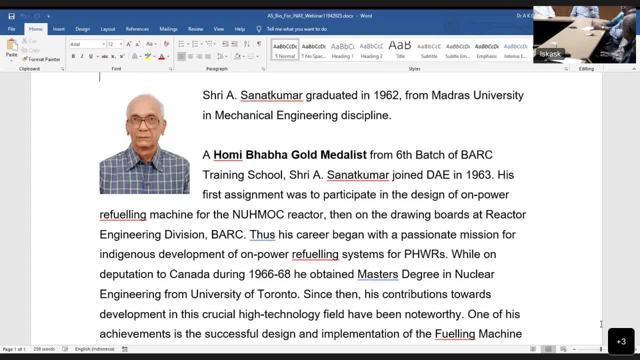 lot of innovative ideas That came into picture during the rehabilitation also. So that is one another aspect. So I think the younger colleagues particularly will get motivated how this effort was put by Shri Sanath Kumar and his team members and we are very excited to listen to him So welcome. 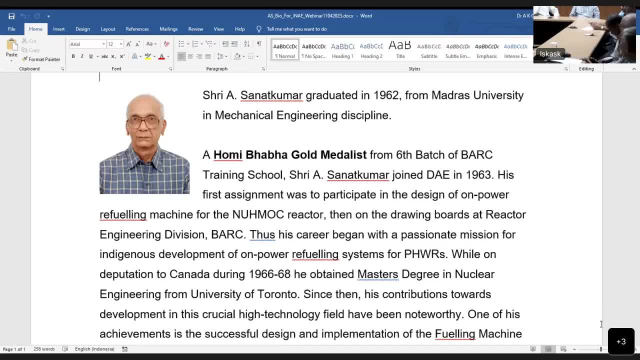 sir, again for this webinar from I&E local chapter of Mumbai and I now request you to give the presentations. Thank you, Professor Kulkarni. Dr R K Singh: I know him as R K Singh. Dr Archana Sharma, esteemed. 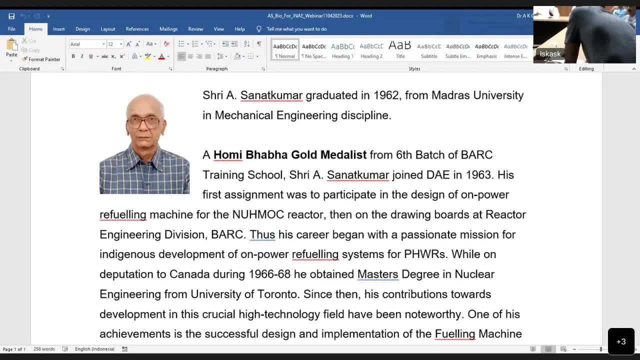 members of I&E fellowship who attended this lecture in physical mode, as well as those who might have joined online Invitees. I see so many friends of mine here: Natarajan, Dr Grover Ardhwaj, Bala Ram Mohan, Kamal Kavadia. so many, so many people here, So I am terribly excited. I only 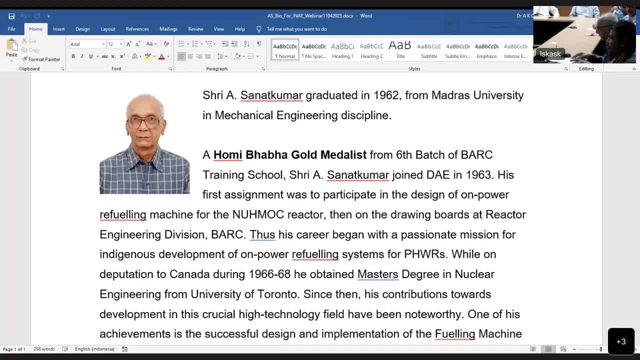 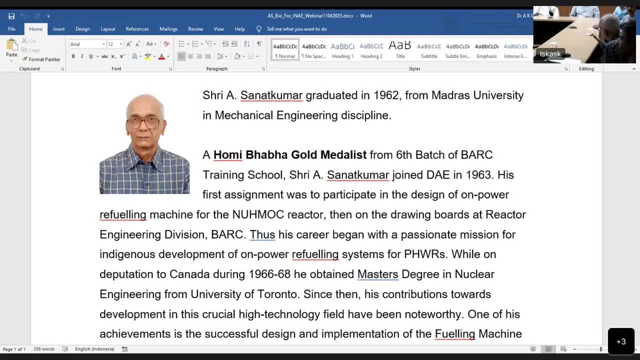 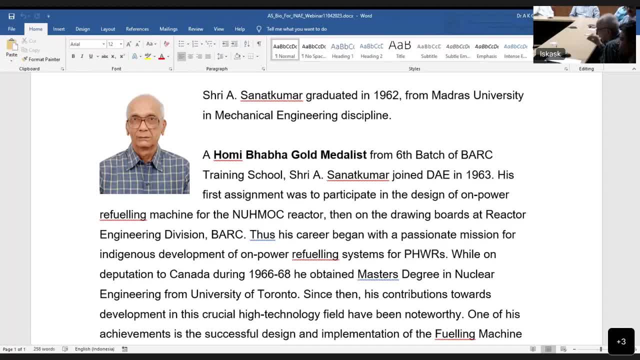 I said earlier that there is- there is not any world without буквatory intention, so all caveats are valid. Are they just blamed one forllers and speculations? Yes, they are, But I'm now going to look on the capitals, as I was talking about a little earlier. 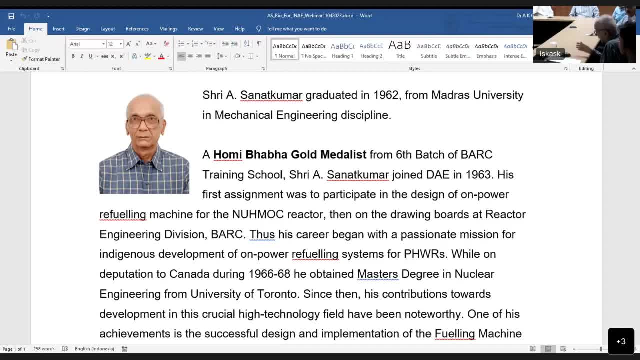 As the artificial client. I'm another kind of hypers efendimatic ninja that chases the falserat. manufacturers and consultants have been co-travelers with us at NPCL and have contributed to this wonderful journey. I plan to cover this lecture in two parts. Part one is really a simplified 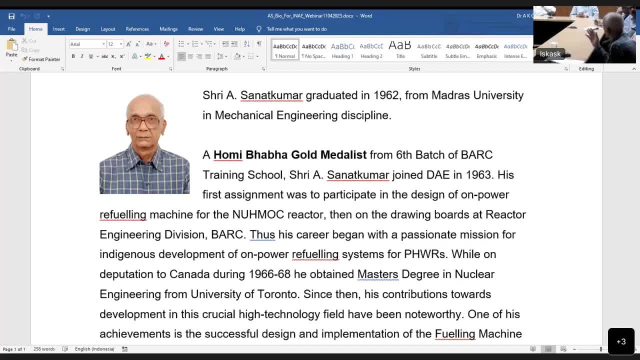 explanation of PHWR. I am assuming that not all here, or not all who have joined this webinar, may be familiar with PHWR. We just have a very different and it's on-power crew landing system. It may be thought of as an abridged course material on PHWR- FHS 101.. 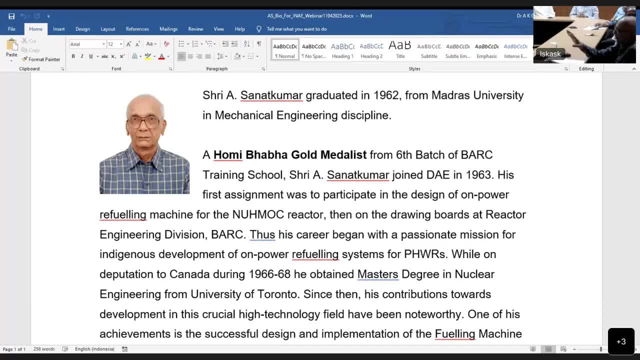 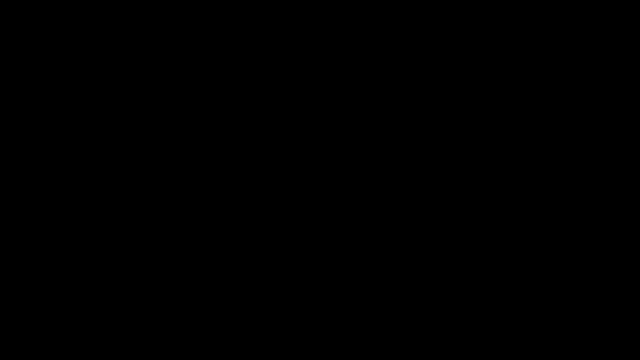 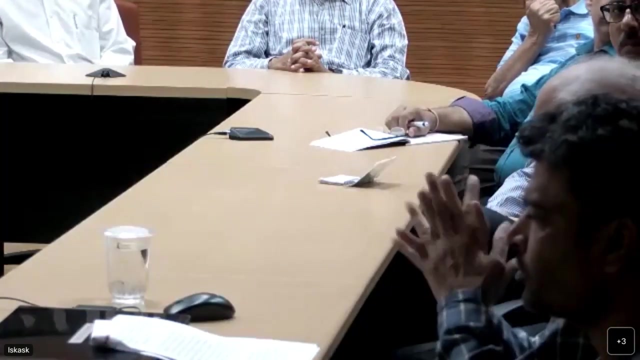 In part one I will cover very briefly about how we got into this PHWR business, Then later on why and how of on-power refuelling. Why do you want on-power refueling for PHWR? Then this is Jk H item. 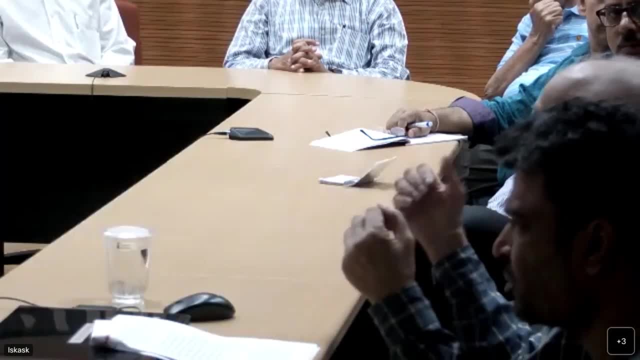 Again. we just have about 18 episodes, 1 series in which I am going to talk very much about Donna's presentation and Financeendo's presentation. The next screen here is… Newheshy. The Newheshy versión de la página del metro. 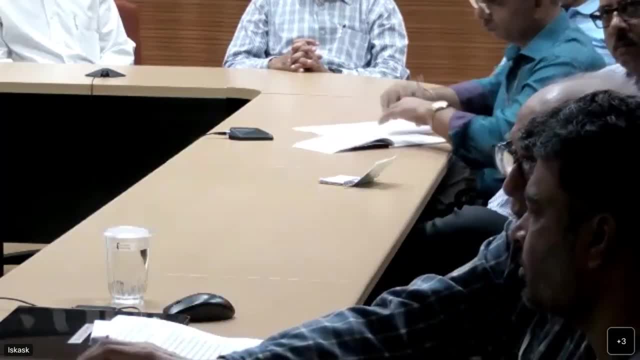 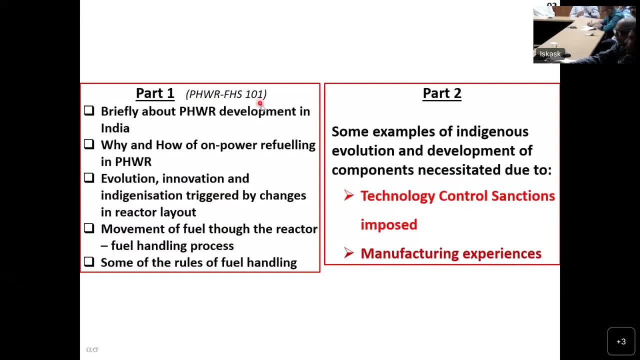 Embassy of harmony. inкимиcom Oywoo co- contrario. the first video Here we will cover the topic that one of them is. we go to evolution and the innovation. what, what, what triggers evolution? why do you want to evolve? why do you want to innovate? i will try to cover that then, for those who may not be familiar. 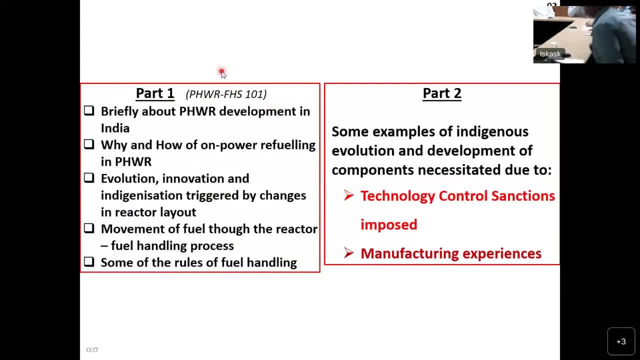 with this i will cover the movement of the fuel through the reactor very, very simply, very easily and finally, based on this, we can enunciate some of the rules of fuel handling, what what we have to call this is important, then. that is part one, but actually i am interested in part two. 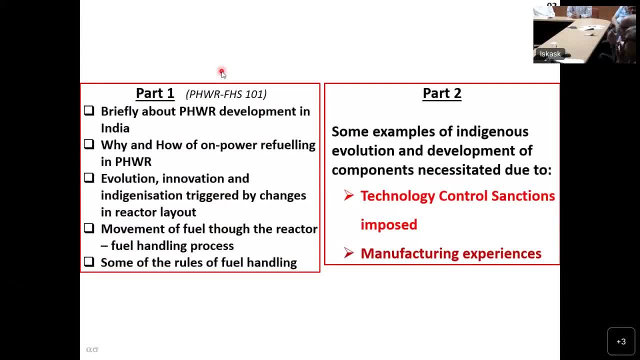 because i am quite keen to explain some examples of indigenous evolution. what has triggered those evolution? that also i would like to bring, and then manufacturing experience, some typical components. time will not allow me to do this, so we start here in 1960. around that time dr baba and his 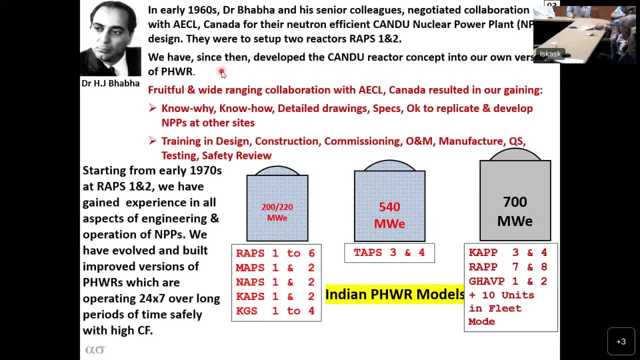 scene, your colleagues negotiated a collaboration agreement with aecl canada for their neutron efficient can do nuclear power plant to be built in india. right from inception, dr baba had insisted that the collaboration agreement should envisage progressive indigenization right right in the beginning. that's what his main goal. 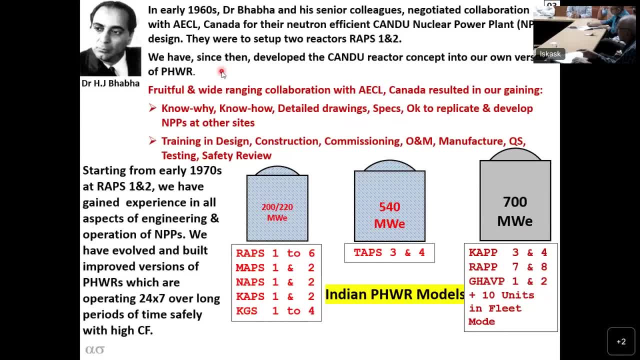 was the collaboration agreement, apart from setting up two reactors at rsps, one and two, also included training of indian engineers, the entire gamut of a can do: power plant design, design, manufacture, quality control, inspection, testing, commissioning, operation, everything, everything including including safety review. everything that was covered. so very fruitful aspect of that collaboration was 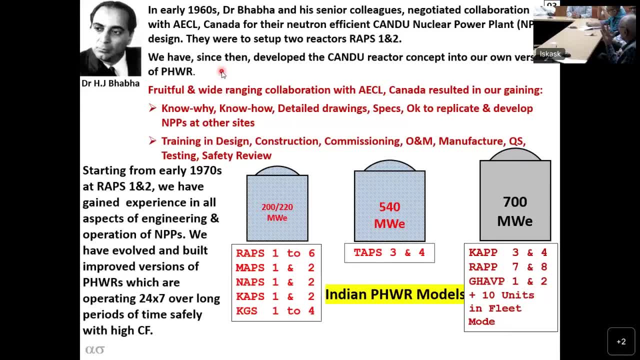 which i think in many of the new collaboration agreements don't have. very fruitful aspect of the collaboration was we got to know. know why very, very important. know why, not only just know how the no, no, why answers was coming to us as and when we asked the questions. so it was necessary for the 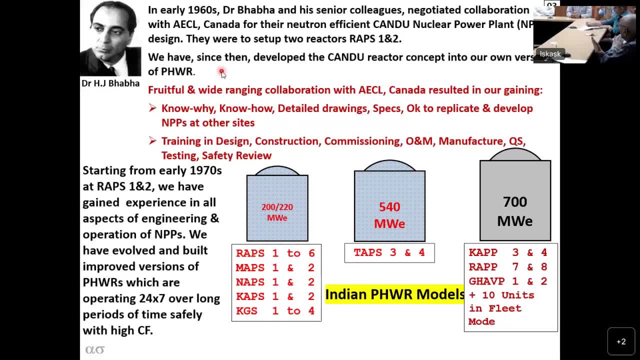 trainee to go and ask: why are you having this? so they were giving, they were not hiding anything, they were giving complete information. so no, that is a very, very important thing which helped us to come up, know why, in addition to know how detailed drawings, component specifications were also given by acl. and, more importantly, they said: you can replicate this. 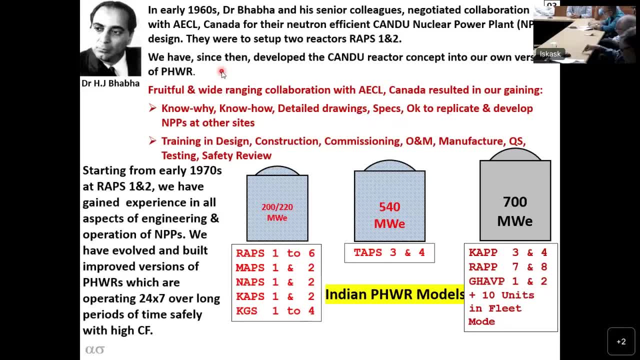 design in other sites. so that is how, after rapone and draft 2, map 1 and map 2 came up on, based on rapone, and after so we had that. then afterwards something else happened that i will cover later. so since 1970s, having imbibed what is there in rapone and draft 2, we have further developed. 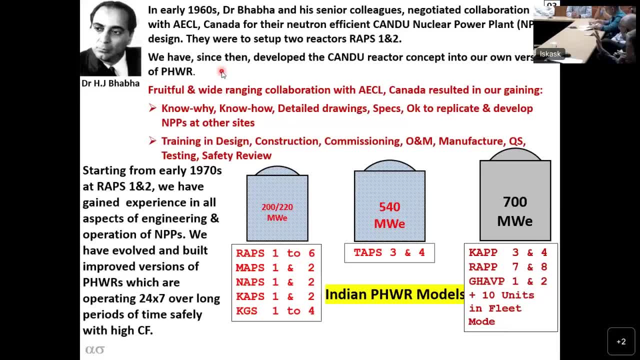 the can do concept to our own phwr. you can say clone, or you can say indian version. uh, my friend jr sinwasan is quite, as they call it, hindu rather than can do, but anyway, uh, it is indian version. so now, now we have from rapone and drop to 16 numbers. we have already built and operated. some are now not operating, but 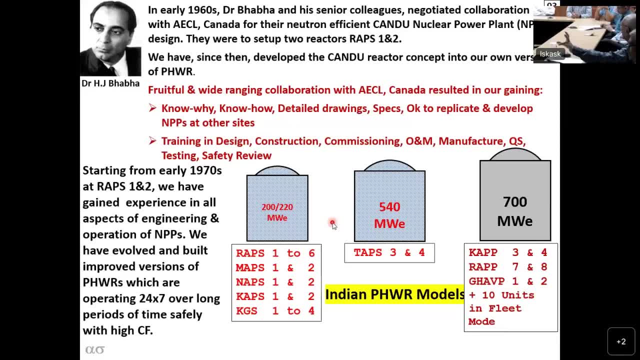 doesn't matter. 16 220 megawatt reactors are on the ground now operating. then afterwards we have built two 540 megawatt reactors. now we are building 700 megawatt reactor that is on the cusp of getting commercial operation, so that fleet mode is there. so this will be the mainstay of 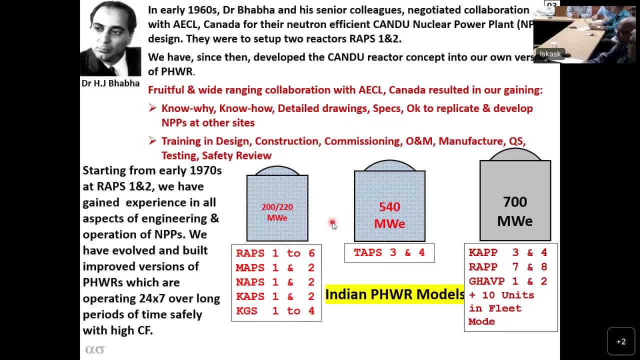 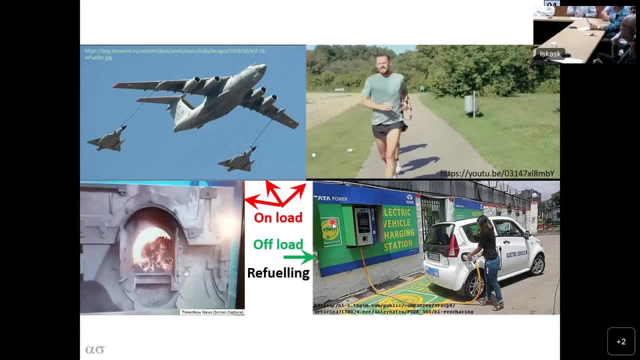 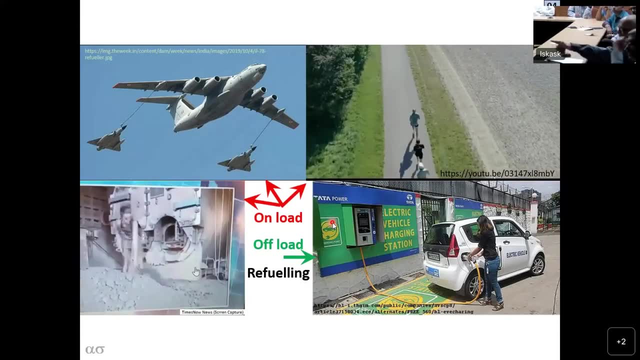 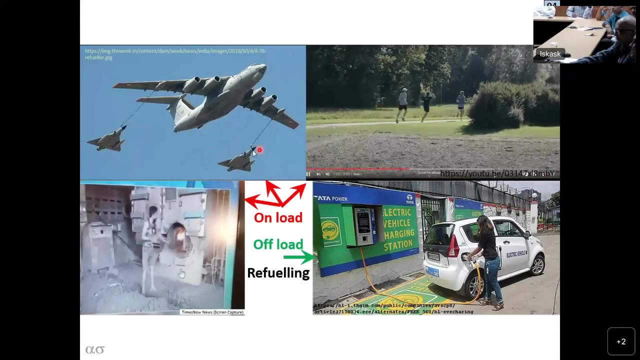 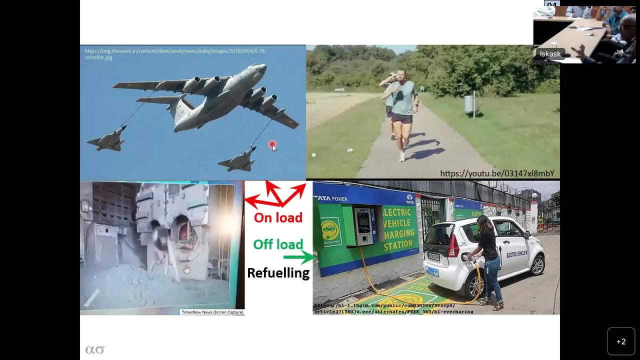 stage, one which was envisaged by dr baba. now, this image introduces you to some extent what culture with that, which is that what there and forwards as well. but if you have pete in advance, these are pete crews not only uh as well as as rd at, but immediately kind of. 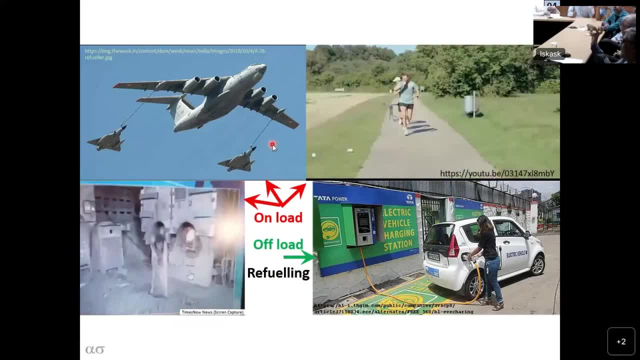 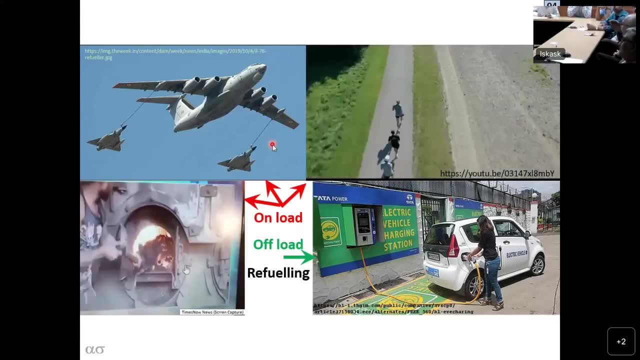 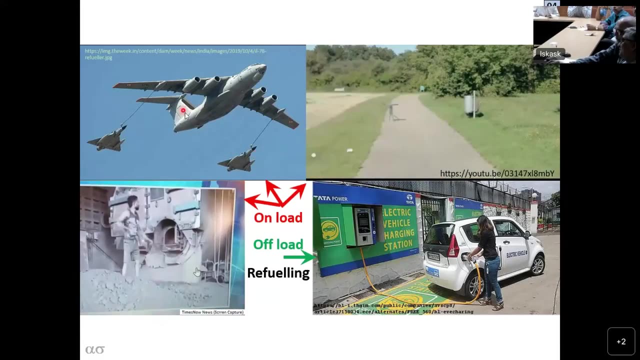 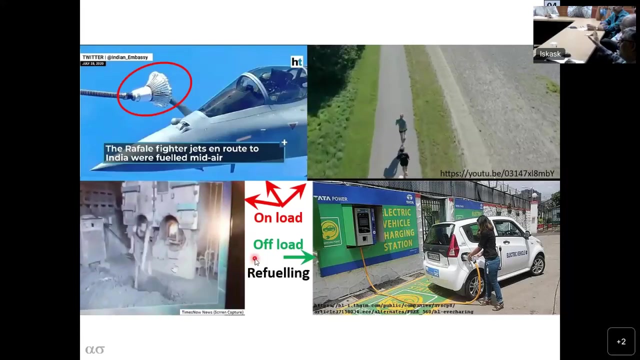 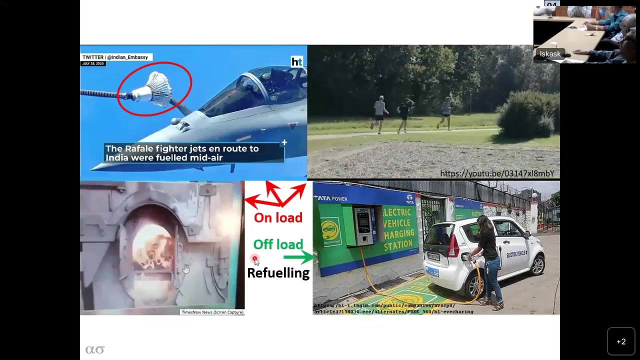 because one change increases the range also. This has got a very similar parallel with our PHWR. Our PHWR also on power refueling, increases our mission time, increases our operation time. So that is very important. So now you may recollect very recently, In recent time, when France made Rafale jets. 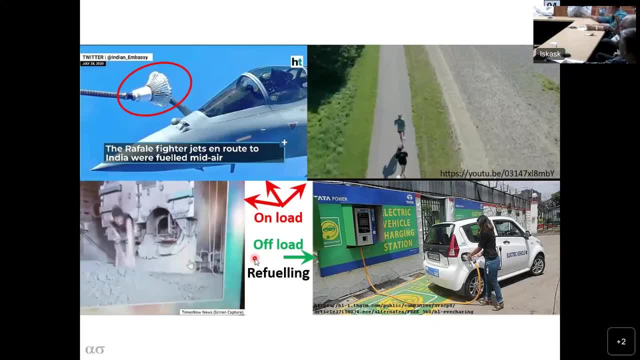 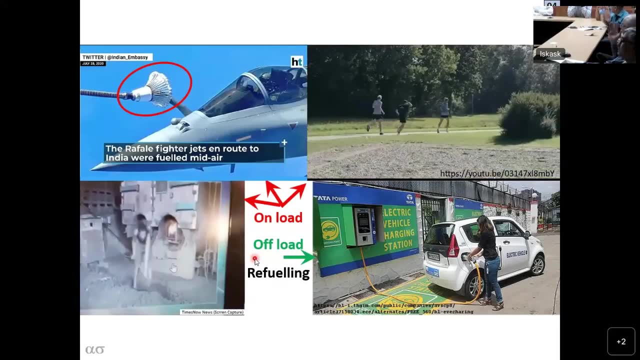 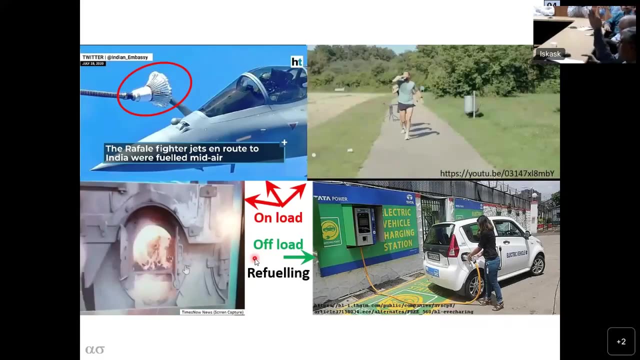 they manufactured in France and they transported it 7000 kilometers to India- media refueling. they never stopped anywhere else. So this is not possible. And for refueling: media refueling is not there. it would not have been possible. This is true even for our PHWR. And one more: 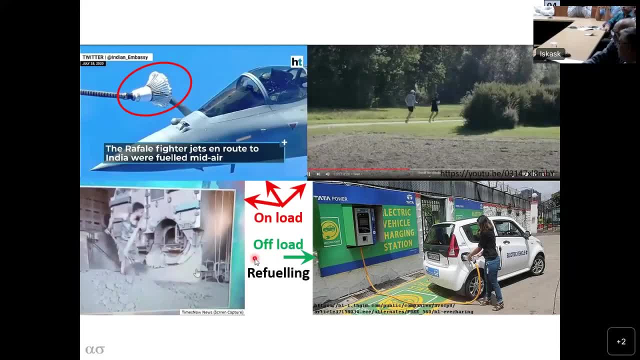 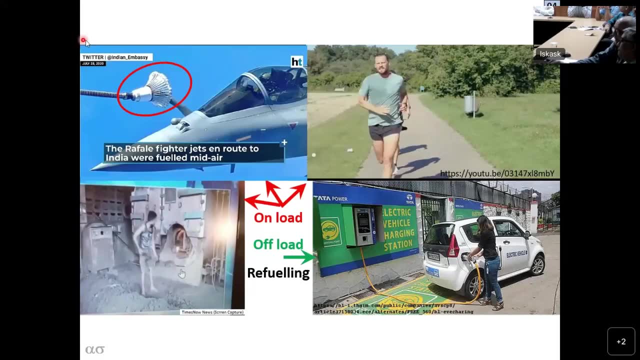 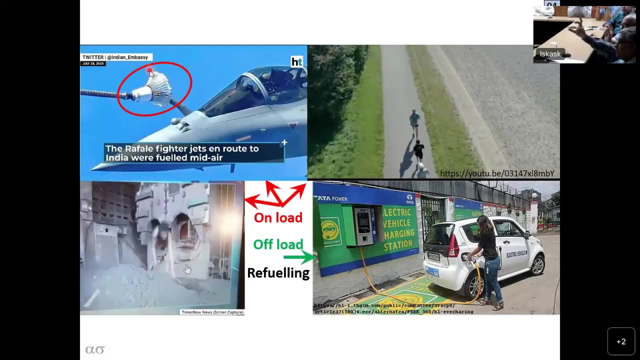 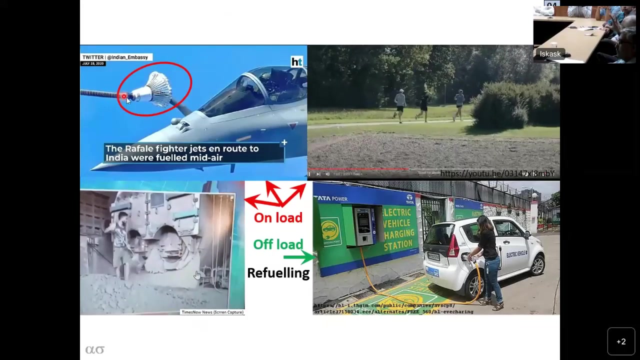 thing Government of India has. Government of India has released this picture. This is very interesting. The host from the tanker aircraft is coming through and then it has got a cup. they call it a drog. Then the receiving aircraft has got a cone. This is a receiving. 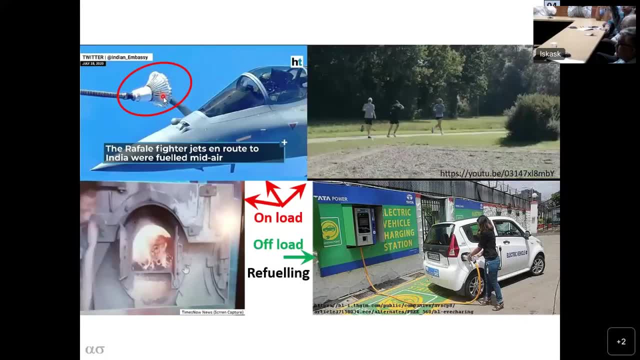 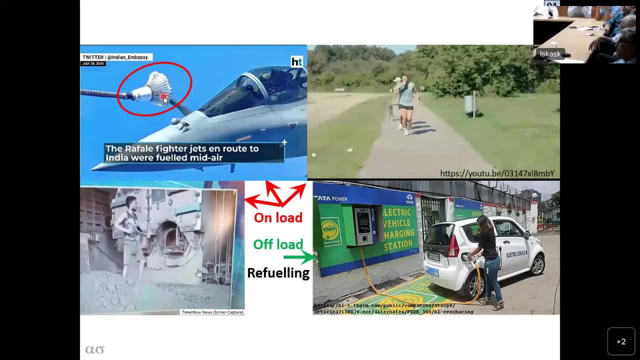 aircraft, And if you see here anything that is dropped from a height, you would think that the cup should be facing the ground, The host should be going to the receiving ground, But it is not doing that. It is coming horizontal. It is as though it is gliding. 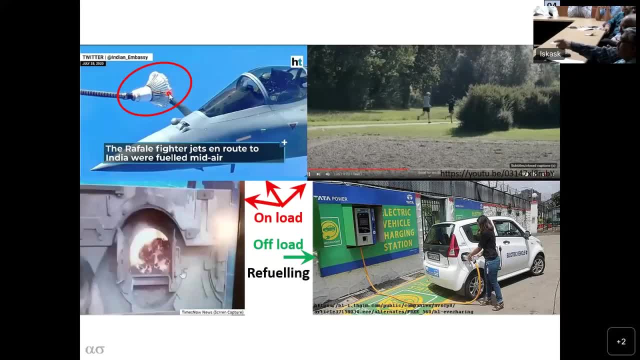 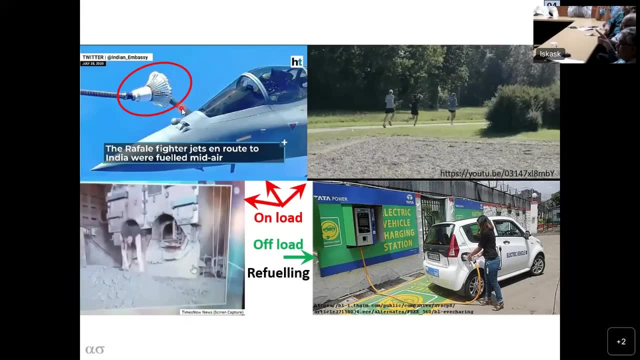 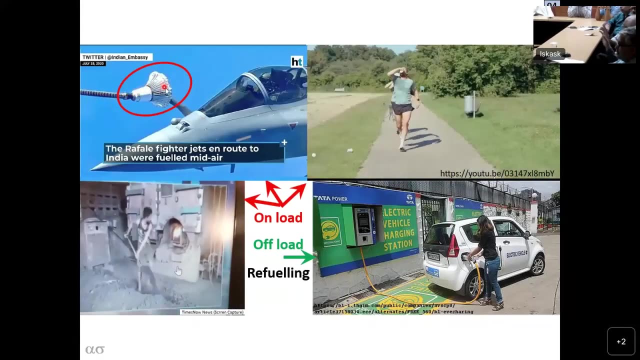 The technology is there, The aircraft pilot is able to come on to the cup And once that is done, only then petrol flows. So this means there is a design technology involved, There is a operations technology involved. This is high tech stuff. This is true even for 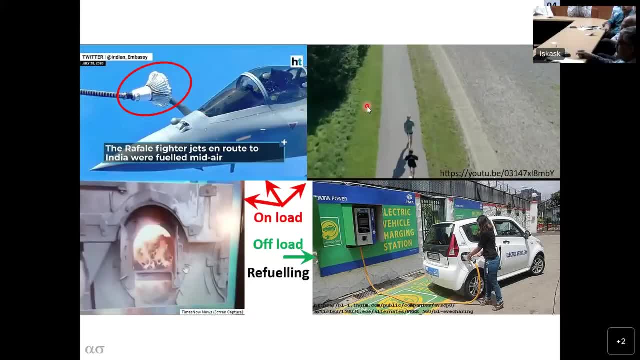 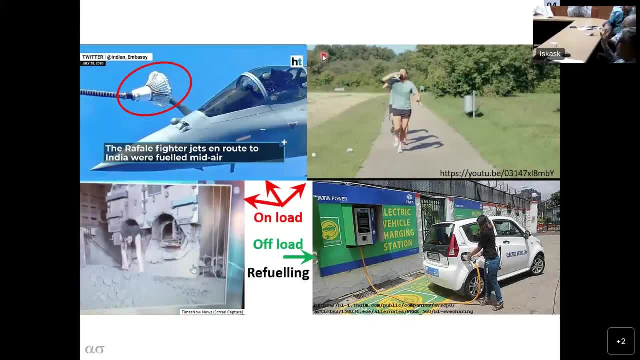 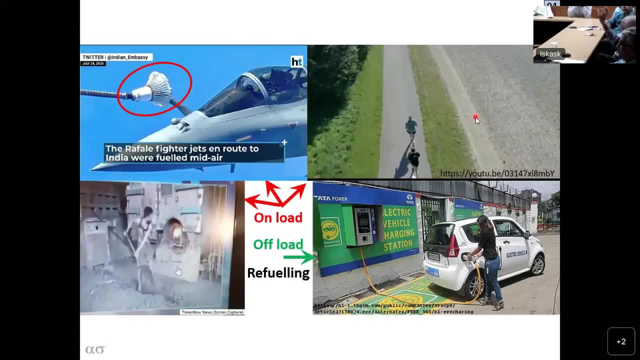 you can see, This is. this is a company, a simple marathon runners are taking tea or drinks- energy drinks- as they are running. They are picking up from the table as they are running and they are drinking it without dropping a stick. You can think of a Porsche. 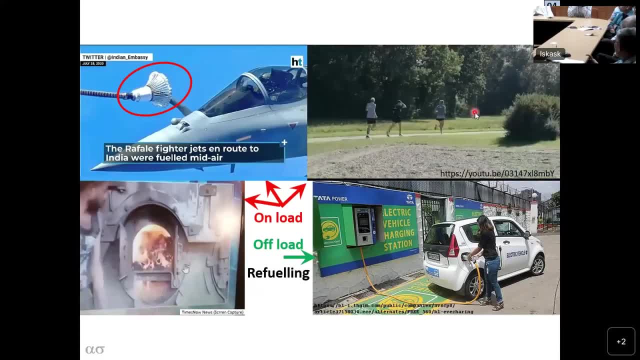 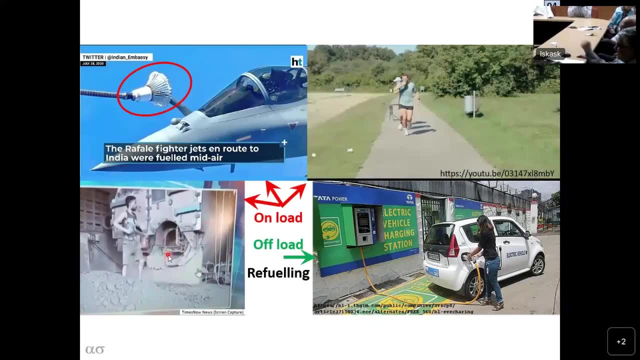 in Shailakop, You know it never dropped even a drop of a stick. So that is what is that? So it is precision skill. operating skill is important. The third one is very common. everybody would know that you are shoveling in coal into. 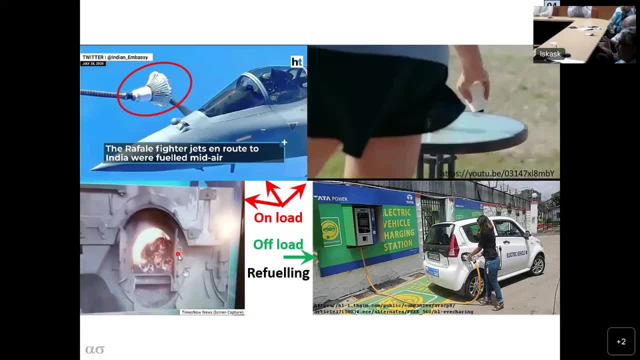 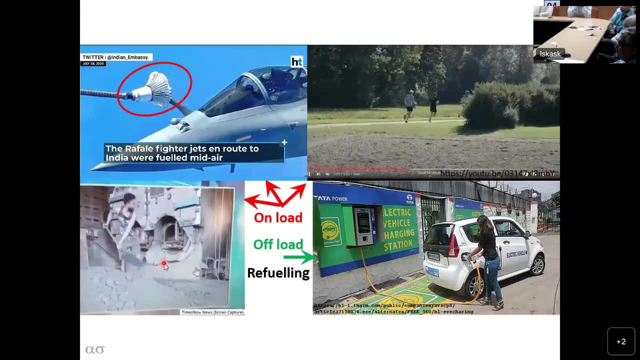 a furnace. This is known as a shovel. That is what I am talking about. You know there's not a very big power point for power plant. this must be a captive power plant. thermal power boiler for a small amount, so manually is loading uh coal in that. but if you see carefully at the end of 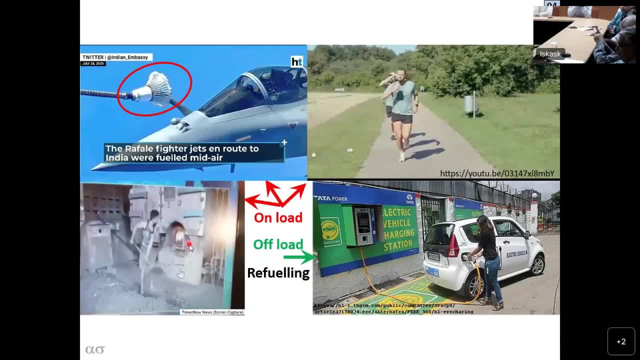 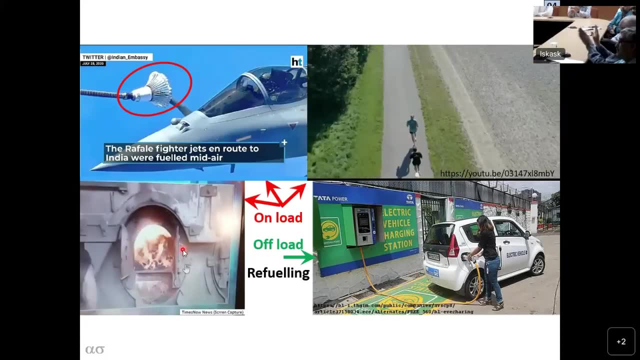 that he is closing the firebox. this is a very important thing. if you don't, you cannot leave that open. this is true even in fuel handling, even in phw. you have to close. whatever you open, you have to close. then one thing that is not shown, which is my criticism of that particular video: 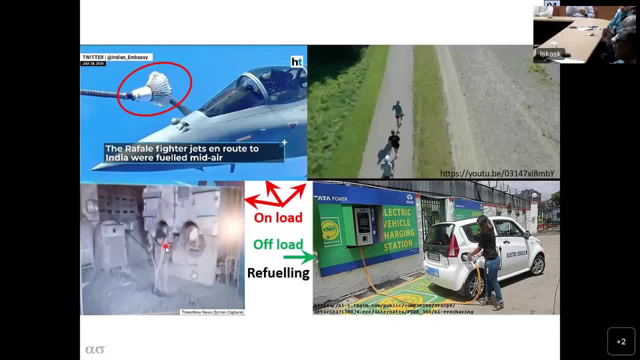 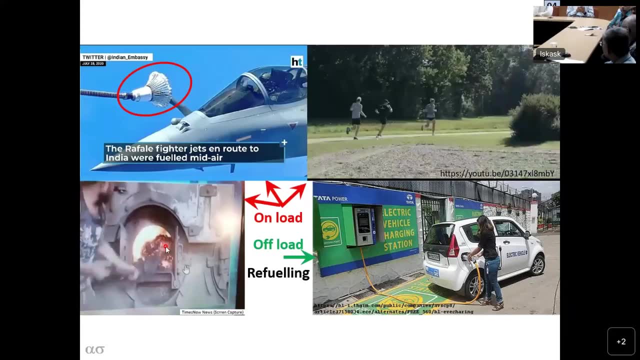 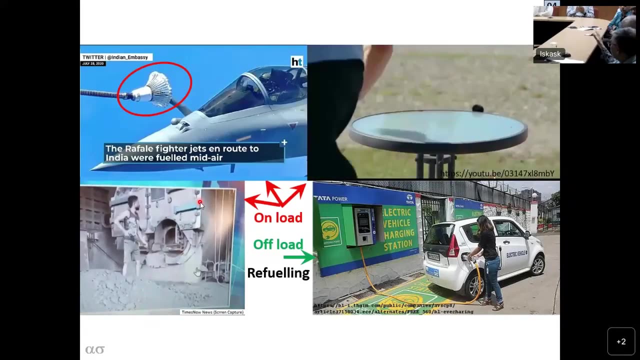 clip is that it is not showing that the operator is removing the ash from the firebox. you have to remove the ash from the firebox, otherwise combustion will be sub-optimal. so in phwr you have to remove spent fuel bundles. that is important for neutron economy. so this is what i wanted. so 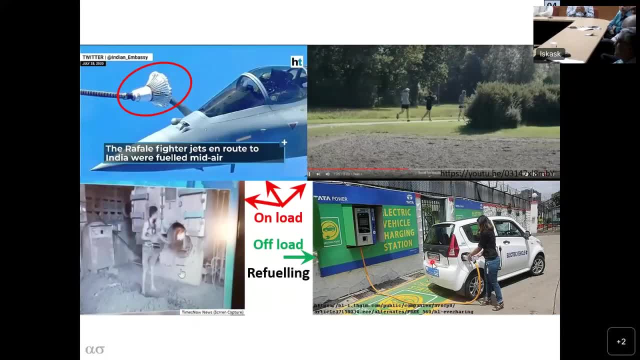 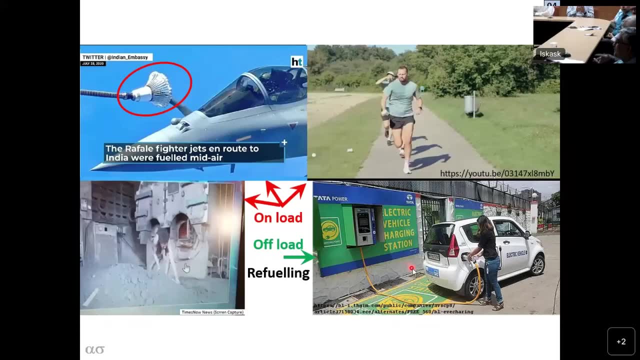 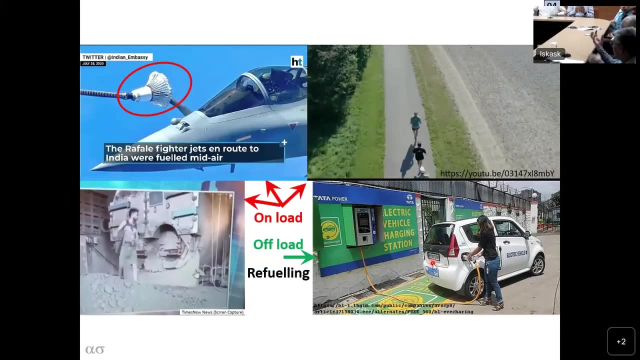 this last one lady is charging her car. it will take her eight hours, according to me, to charge that car with the ev, but i hope that in future- in a few years time, uh- we will have technology developed in india also for cars to pick up charge as they are moving. apparently in germany it is already there in autobahns. 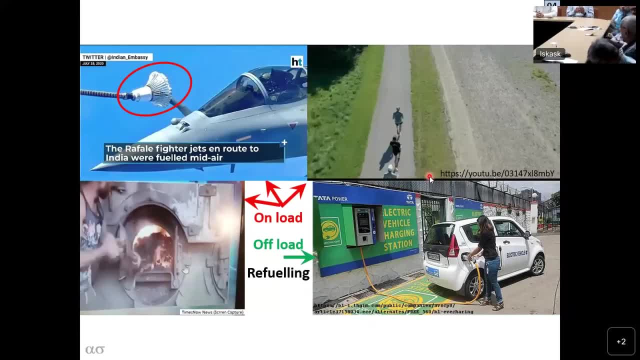 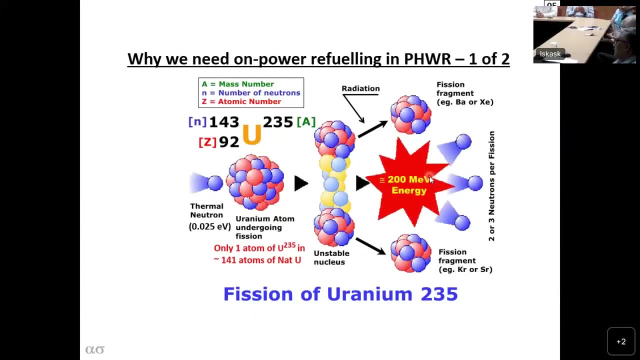 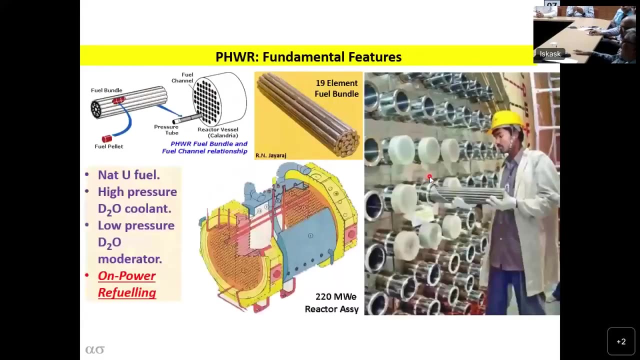 their trucks are capable of collecting uh, getting charged as they are moving in the high speed. so this is uh. reactor physics is very important for any part of nuclear engineering, but i will miss it for the present here. time is not there too much, so i will miss these two times. now. this shows here what the phwr uses: natural uranium fuel. 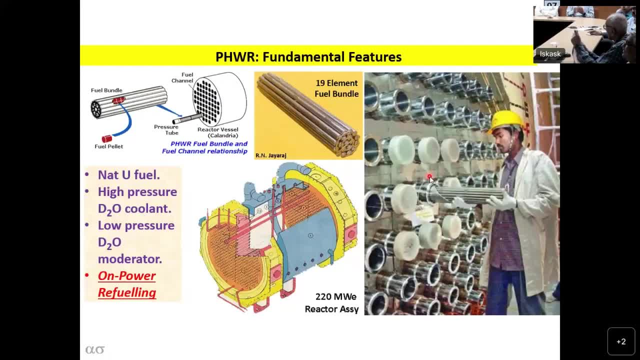 unlike our reactors that couldn't clone, which use enriched uranium, this uses natural uranium. energy uranium, if you put, you can keep the reactor operating for about 18 months now because it has got a lot of enrichment, but natural uranium is having only very limited supply of uranium-235. 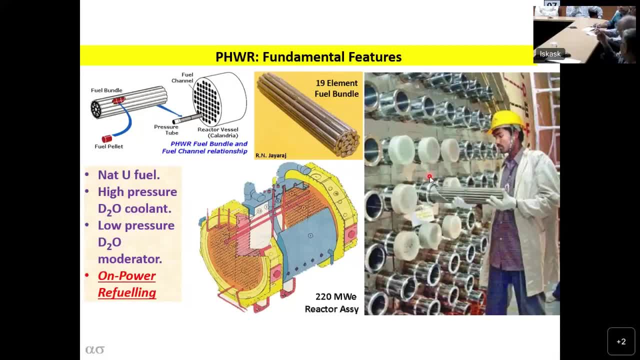 therefore it requires loading fuel and unloading fuel at frequent intervals, so you don't want the reactor, power reactor to be stopped for just for the purpose of fuel loading. so therefore, that is the reason why on for fuel handling is mandatory, essentially for phwr power reactors. uh, you see here. 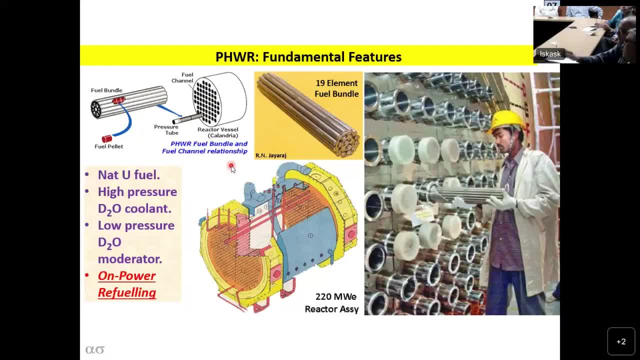 for those who are not familiar with the reactor, this shows the cutaway view of a 220 megawatt, and this is the brute that we are handling. this is the bundle, which is about 500 millimeters long. in this particular case it is 19, 220 megawatt. now. this inset here shows the relationship between: 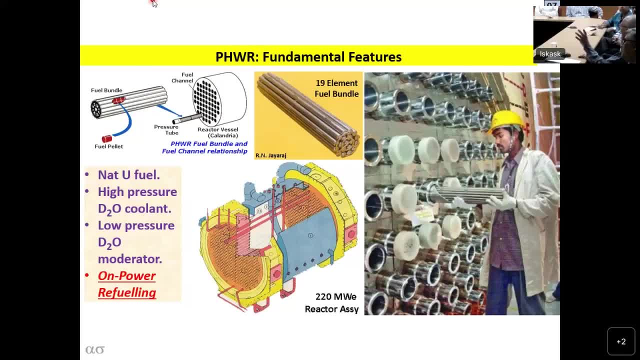 between the bundle and the reactor. the react you, all of you, are interested, is get the bundles into the reactor. eight bundles into the reactor, eight bundles out of the reactor. this is what we are interested. that is what you are showing now here. this picture is very interesting. 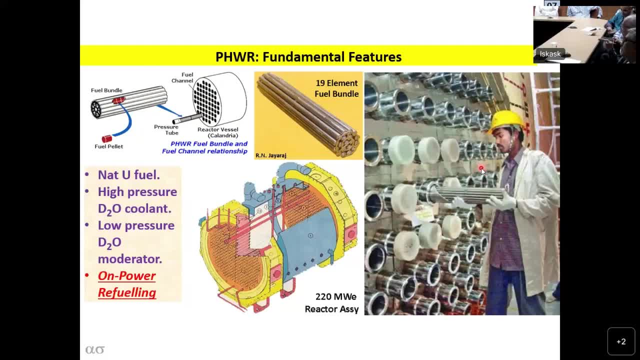 this is a real picture from tharapore 3 and 4.. real picture from tharapore 3 and 4 where the operator is loading fuel. for the first time. this is manual loading. manual loading can be done with the initial loading at the time of critical before. 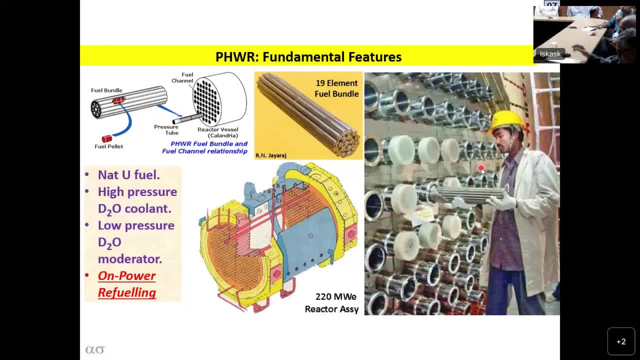 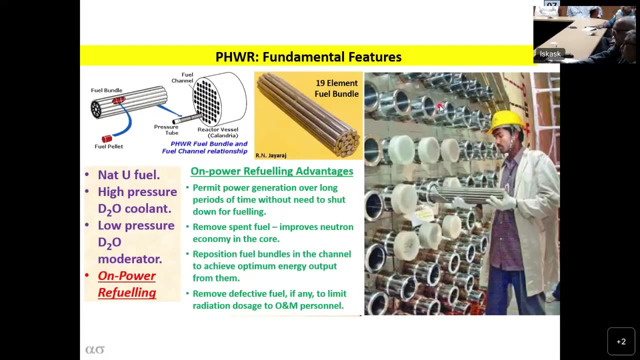 going critical. it can be done only manually. you will notice that this is the reactor phase and you can see the reaction. this is one of the reaction phase that i am going to show you. the reaction phase is very similar to the one which we were talking about earlier. 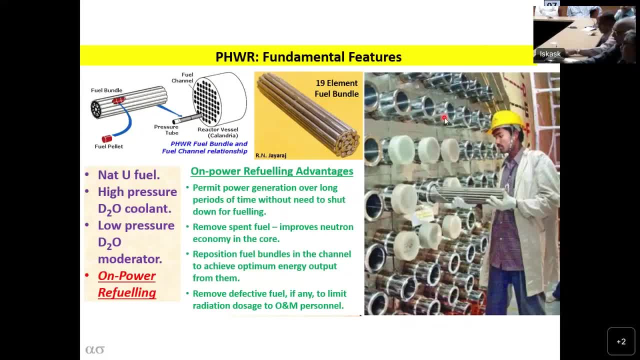 this is the react phase. this is the react phase. this is what we are calling channel. i'll come to that in a minute. that's the end fitting. so you see here. the important lesson here is that a new fuel bundle can be handled manually. one bundle at a time can be handled manually with gloves, but more. 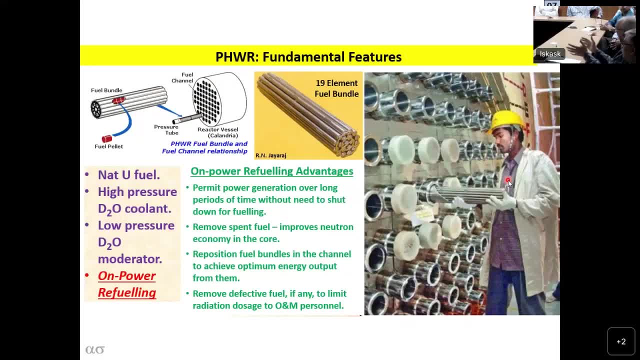 because uranium oxide pellets will get damaged. so you handle it and then he is loading it into the channel. he has to load one by one in the. when you are starting a reactor you have not all of them, as naturally you have some thorium bundles out of there. the reactor physicist will tell you which. 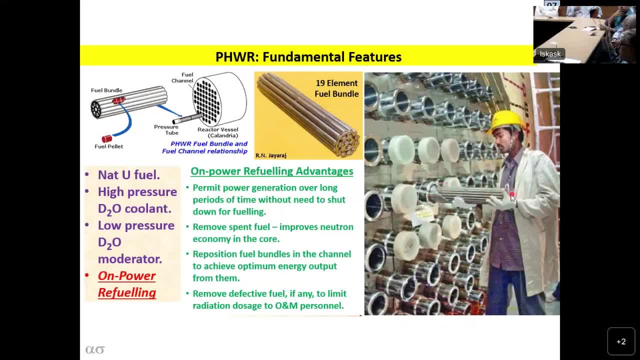 bundle has to go where. so he has to load something like total of 5096 bundles in a 500 megawatt reactor before it can be done. then there is at the time- at this time, there is no criticality because there is no moderator. it is dry channel. so this is what you are doing. this is not automatic. on. 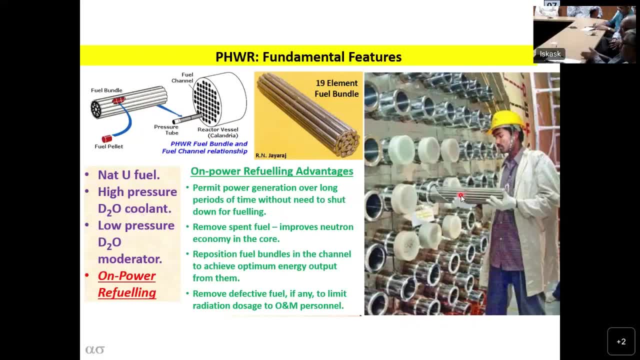 power refilling. this manually filling is a necessary operation for every reactor. now this- i don't know whether you're able to read this green portion here indicates what are the advantages of on-power refilling, which i have so far done. a: it increases the time uh of operation uh. 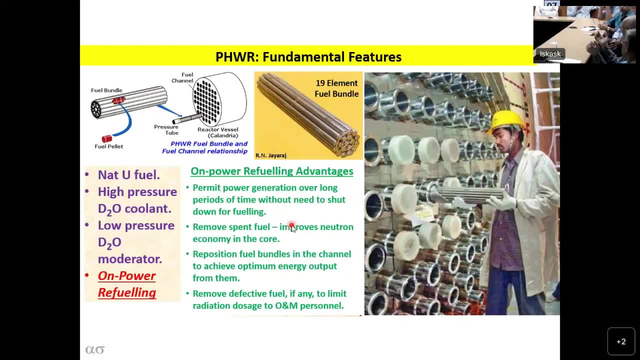 dr uh here he has already said five, nine of 900 days, so i will come to that in a minute. then there is one more important thing. very often you want to reposition a bundle from here to here, from here to here, to get in between the core, to get better output from the bundle, because the 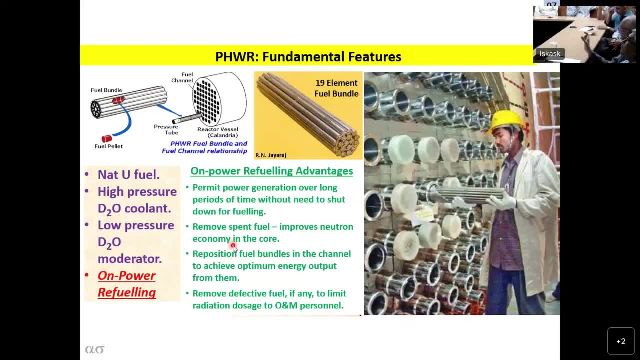 neutron flux inside the core is not all uniform. so you want to less burnt bundles, you want to put it in a higher bundle so that you can. so the fuel handling can uh, do it in a different way. so do it on power and, more importantly, this is mr nitrogen's area. you can detect failed fuel bundle. 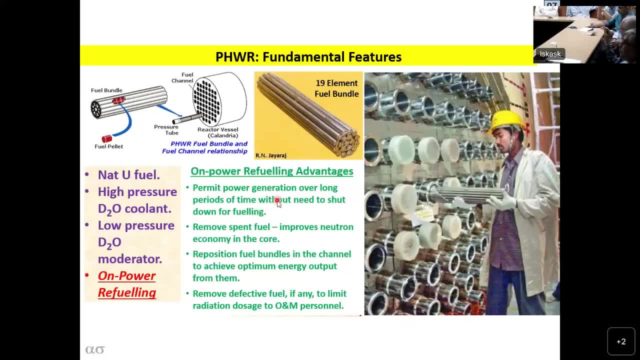 sometimes fuel bundles fail. if you detect failed fuel bundle, a failed fuel bundle will release spent neutron efficient products into the coolant. so you can detect that failed fuel bundle and try to recover. remove it from the channel. otherwise radioactivity will come and accumulate in the primary coolant system and it will be load on the mandarin, load on the people. 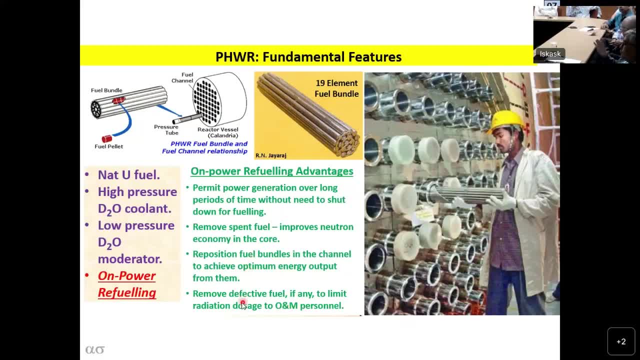 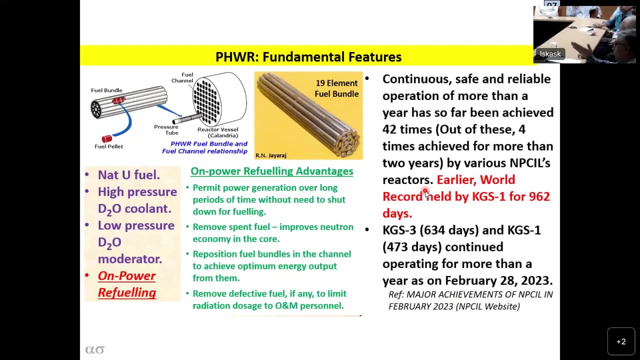 so these are the very important uh aspects of uh. now this is uh. having said that, i'm just trying to give you some statistics. latest statistics from npsl website: continuous, safe, reliable. reliable operation for more than a year has so far been achieved 42 times, not just once or twice. 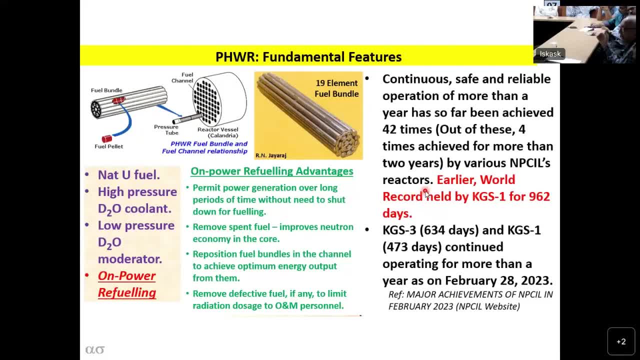 it is 42 times it has been achieved and since uh npcl world record it had kg kaiga 1 had a world record for 962 days for some time. then canadians got very worked up so this ran their reactor, so anyway, then kgs3 and kgs1 have got really already 634 days and 400. this is not the kind of uh. 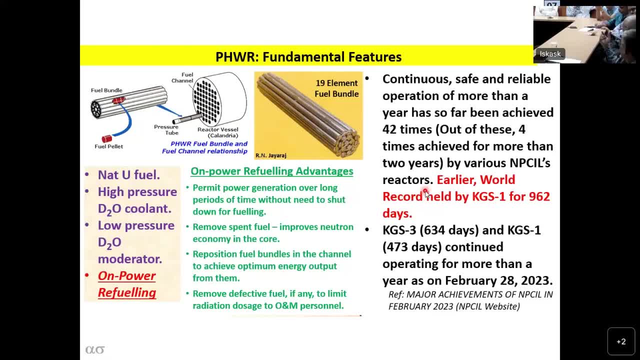 uh performance we normally expect from thermal power plants because there are other reasons- they don't have coal sometimes, etc. but this is a terrific uh thing with phwr has been now take care to this. i want to emphasize this performance has not come. i'm not trying to 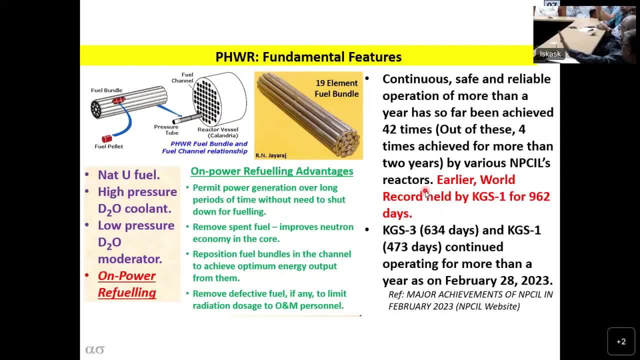 say that only on power refueling has achieved this. it's not like that. along with the on power refueling, which is a major contributor, other things also have to work. yeah, fighter aircraft: thousand kilometer is not only the fuel, the engine has to work also. so many other things have to work. 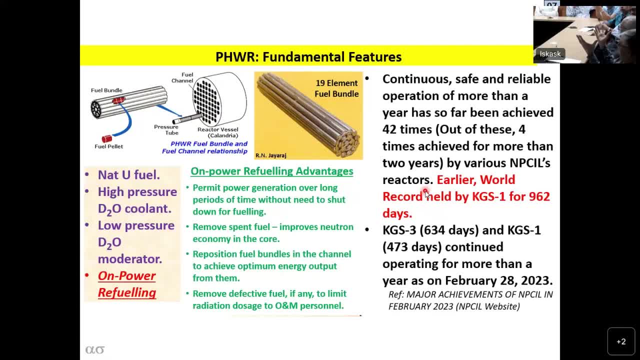 so it is. uh, it is like the whole system has to work like a well-tuned violin or a vina or a sitar. it has to be perfect. only then it will happen. and that we have achieved so far- and we should, of course, achieve even more, that doesn't matter, uh, yeah, okay, next week. 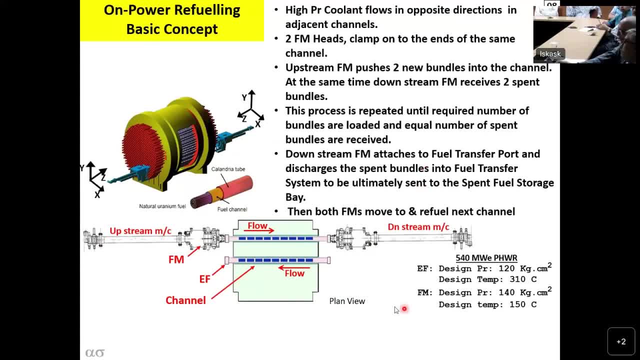 now this one, very simple, describes the reactor for those who are not familiar with it. the reactor itself is a low pressure vessel which contains moderator. the thing is through the reactor like a heat exchanger to uh 300. for a 220 megawatt reactor there are 306 coolant channels going end to end. 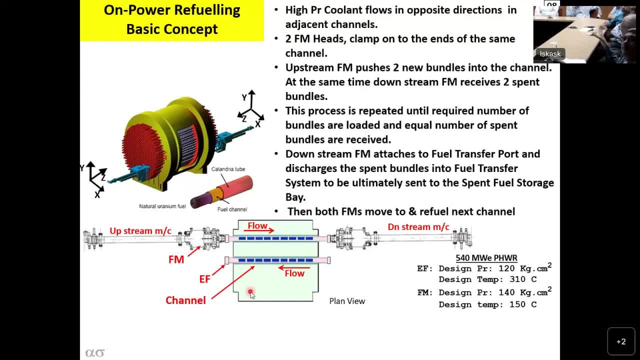 coolant channels going there. this innermost tube is called the pressure tube. it is actually a pressure vessel. it is designed for containing high enthalpy heavy water. high enthalpy means high pressure, high temperature. not only that, it contains the fuel bundles also. so our job is to push fuel bundles. 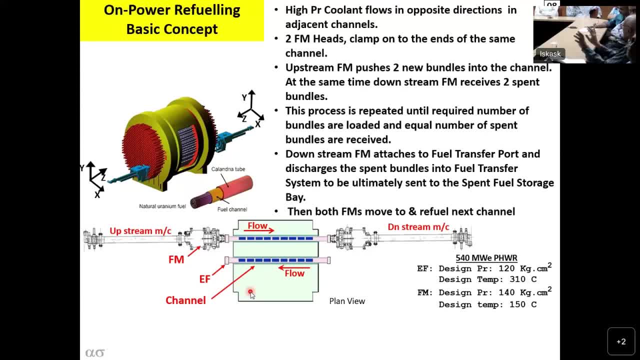 into that core there and if you push number of bundles you have to take that number of points. now normal standard practice in our pressurized water reactors is that you push eight bundles and take out eight bundles. that doesn't mean only this is possible, six bundles possible, four bundles possible. 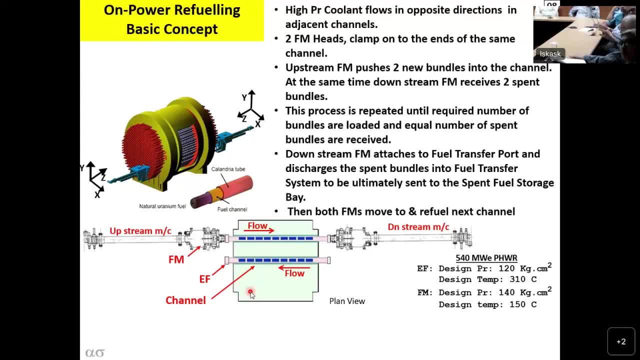 two bundles is possible. it is possible, but that means the programs have to be specially made for it. really like that we will come to taking out in a different way. so now, as far as this refueling is concerned, react refueling is concerned, one can simply say, hey, you push, eight bundles, you take. 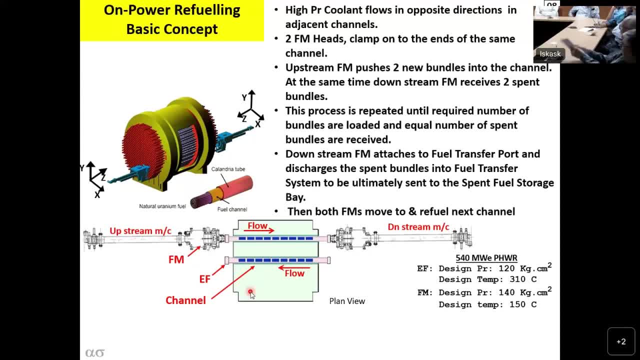 away: eight buttons, very simple. now they're talking about this simplicity. i am reminded of a story. once, when mr azerudin was the captain of the Indian cricket team, Australians came to play a series of test matches. One reporter asked him, Sir, if you want to beat these Australians, you want to 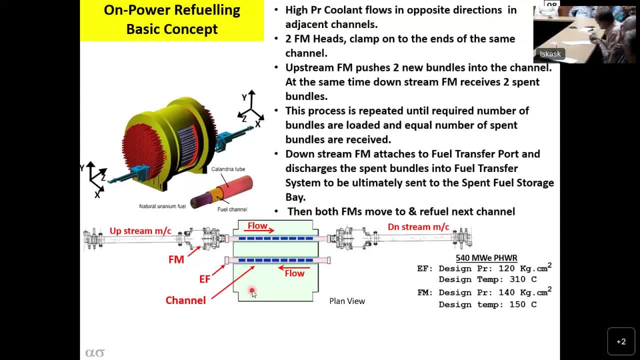 win this series. what do you have to do? Azharuddin, very, very, very characteristic, very simple way his leg glance. every time he got in a hole, Same way, very, very simply, he said: you have to bat well, you have to bowl well, you have to field well, you have to run out. 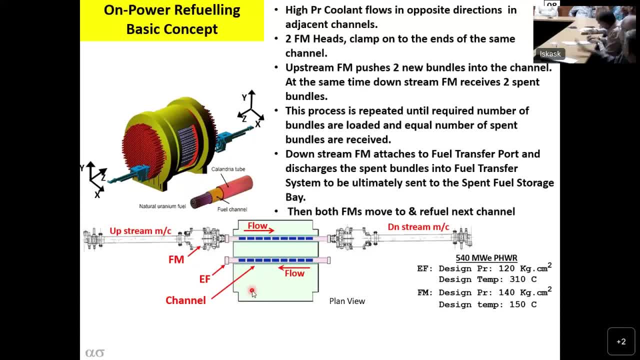 well, you have to run between wickets. well, If you do all this, you will win. So, like that, you can take it. but refueling is done. It is not like that It is. the devil is in the details. So that is what it is. So you have here- incidentally, it is on. 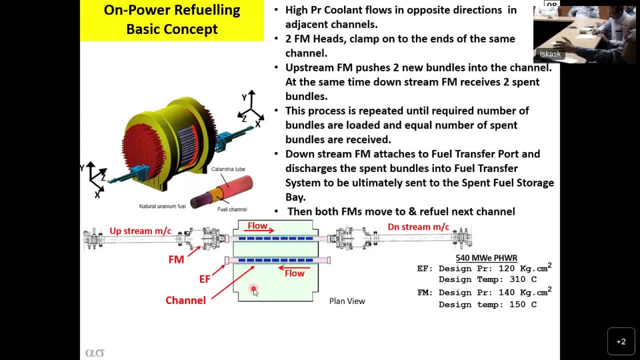 power. That means you cannot go anywhere near the channel when it is reactive operating. So you need a machine here, you need a machine here and you need a machine here. And the machine has to push here, this machine has to push. Now another complication, slight. 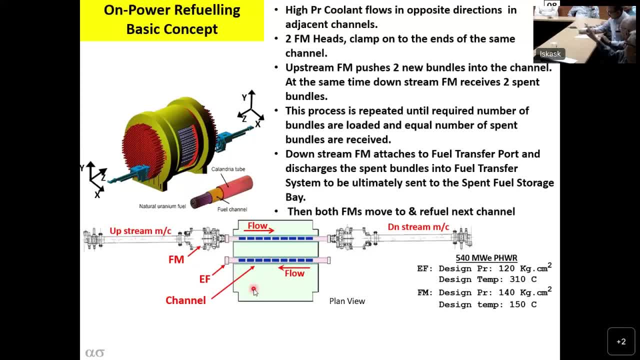 complication is that the flow In each channel is not in the same direction. in all the channels It is going in one direction. in one channel- alternate channel, it comes in opposite direction. So we do fueling from the upstream end. You fuel at the upstream end, spend fuel at the downstream end. So 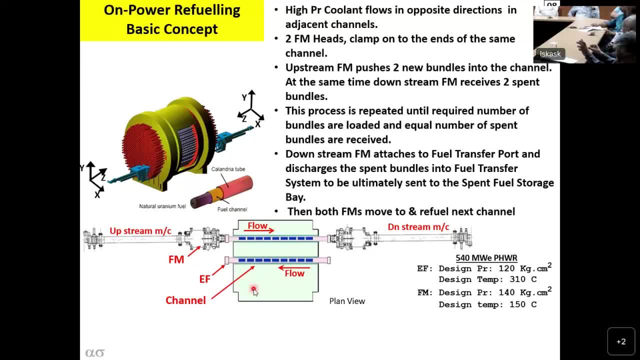 this downstream end fueling machine will become the upstream end fueling machine at another time. So that means the fueling machine has to have dual role. like our cinema actors, you have dual role. It is both upstream and downstream machine. it has to operate like 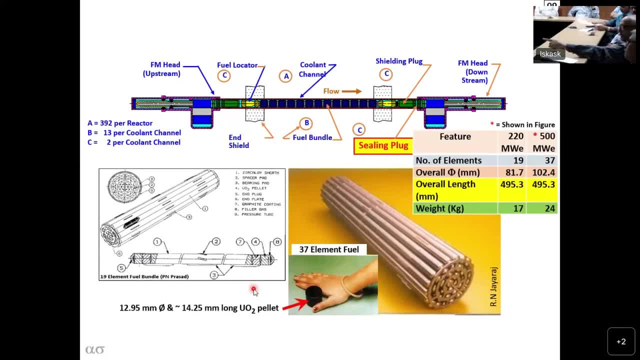 that We will come to that in a minute. Now, this is a bigger view of the channel. this is a view of the bundle and this is more detail. we will not worry about it. The channel is like this: here And two machines are clamped. 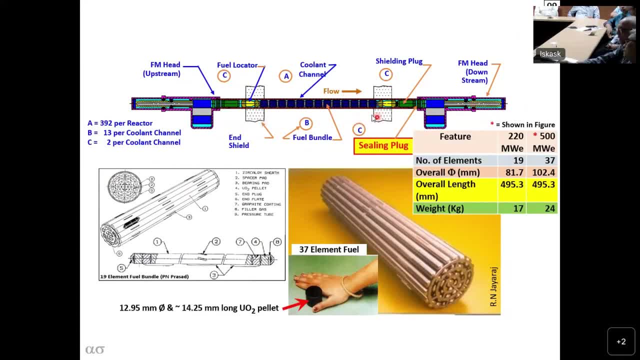 here The fuel bundles are right in the middle, here in the core, And the channel also has got some hardware. But the purpose for which I put this is there is a component called sealing plug at the two ends. Yes, the reason is that when you open a pressure vessel, you have to open, then you have to close. 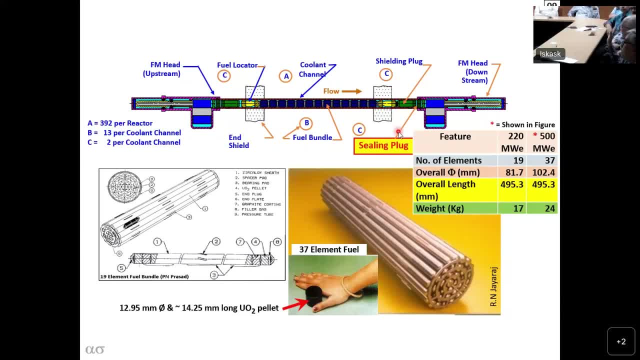 it and you cannot spill any water. this is the thing here. so that is the why I wanted to explain to this. people normally say this fuel on power refueling is all very tough. we are opening a pressure vessel every time, every day, two times. you are opening and closing. 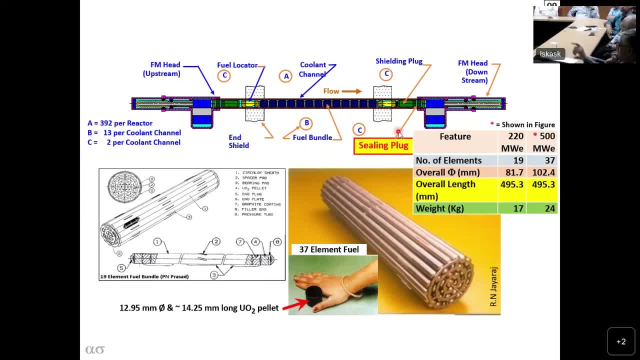 this is no good. that is not true, because that ceiling plug is a wonderful gem of a design by AECL. in that is the one that is one of the, of course, a can do reactor has got several, several very important points, but this ceiling plug is one of the very important concepts. 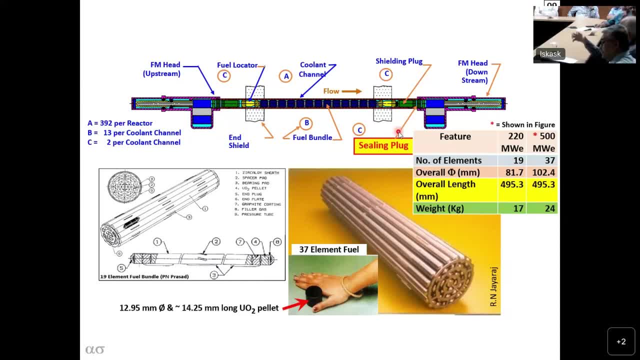 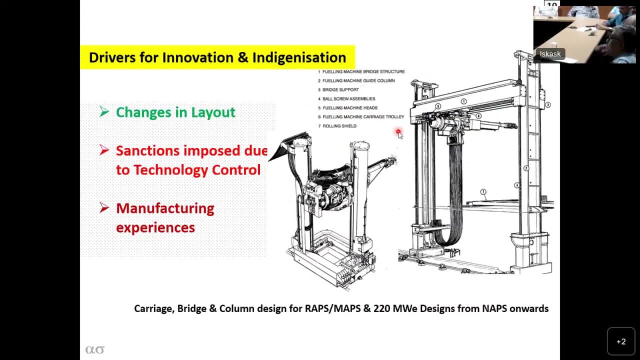 which is fueling machine, operates with the channel. so this integration is very beautiful and we will cover that in a minute, in the other term. so now we come to this, in from AECL. you got this machine. you got this machine for RAP1 and RAP2. why do you go about making this more? why? why is it necessary? why don't? 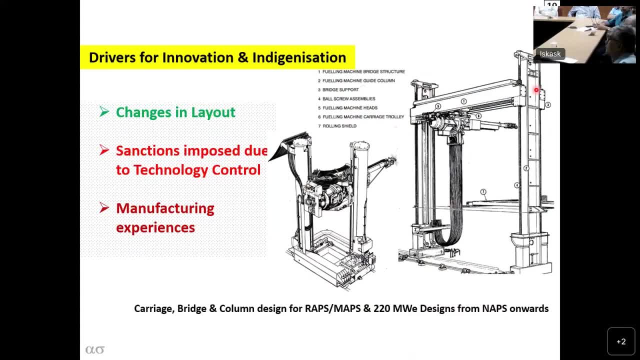 you go along with this? this is a very often a question that is asked of me. why do you want to reinvent the wheel? according to me, wheels have to be reinvented, but that doesn't matter here. these changes are often mandated by changes in the layout RAP1 and MAP1 layout. 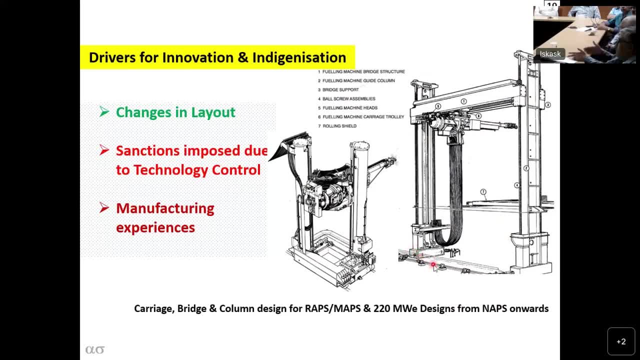 is not the same as Narora and others. because of the seismic criteria. our way in which we do the work is different. so many other reasons. so whenever layout changes, your fuel handling system design also has to change. this is the reason why. next one now I will explain to. 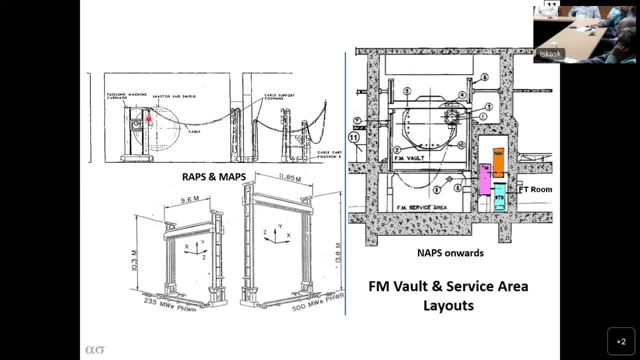 you here this: this is the RAP reactor, in which the reactor is here. the fueling machine here, like a fueling machine, is a mechanical equipment. so, like an aircraft or a car, you need a garage for doing maintenance, periodic maintenance. things won't work. you have to make it work. 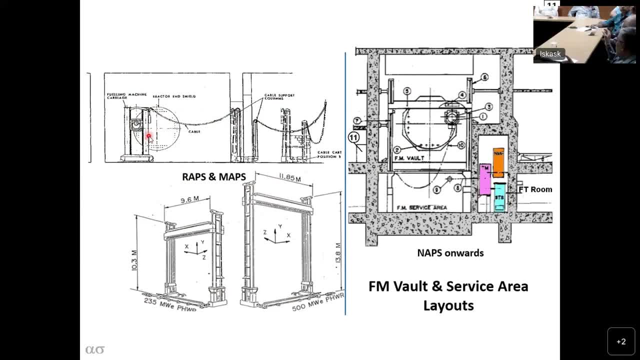 etc. etc. you can't do that when it is inside the vault. fueling machine is a mechanical equipment, which is the radioactive, so you have to bring it out. that area is called service area, and when you it is, or if you cannot go there and bring it out, it has to be done from. 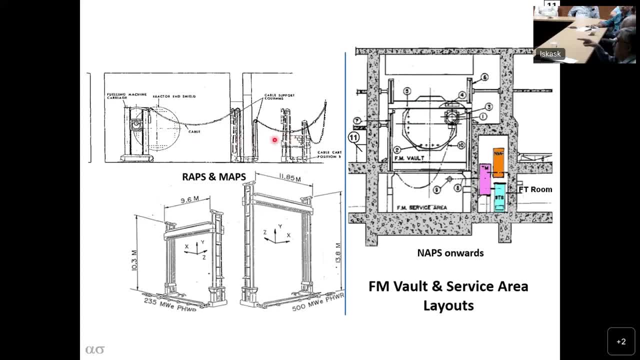 the control room. so when that is done, when the fueling machine is done here outside the vault, there is no radiation or much less radiation, and people can operate it in RAP and MAP. this service area is in the same plane as the reactor vault, as this fueling machine for seismic requirements. 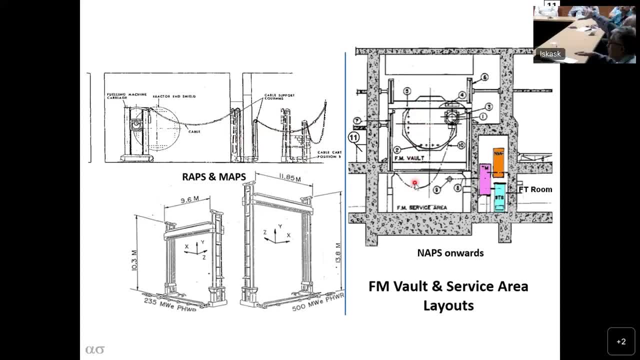 you can go up for storage. it got to go towards RAP. it was in the believe. it was a deep well, but you know the extra we had to put it downstairs below the water is the Walt is here, the fueling machine is here, so the fueling machine has to go up. it has to. 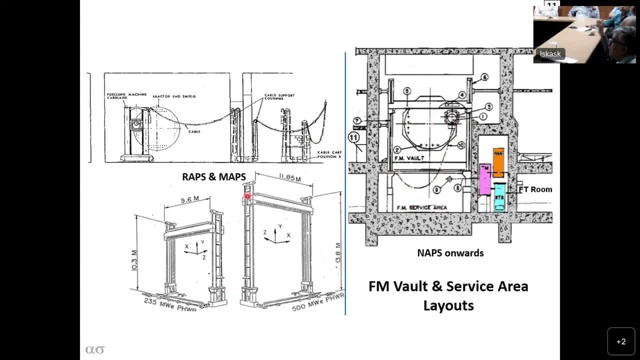 go up on the column. it has to go up on the column. there is a bridge that will go on there, so this is the one that has made this column. the same is necessary, which I showed in the previous slide now that once you have done that, it doesn't stop there if your fuel transfer. 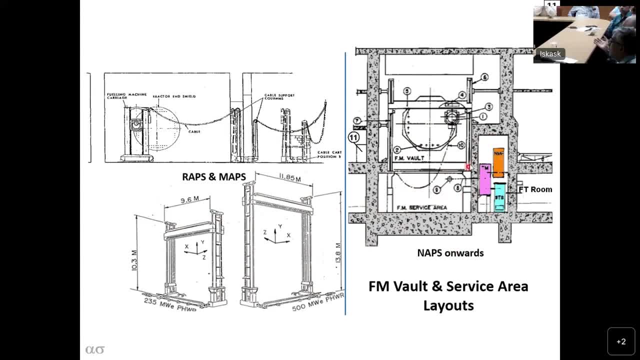 system has to be safe. what is the filter? you have to get the new fuel into the fueling machine. so this is the fuel transfer system. the fuel is stored in the fuel and it is controlled. so that is a new fuel transfer system. you got to spend the. take the spent fuel from the machine. 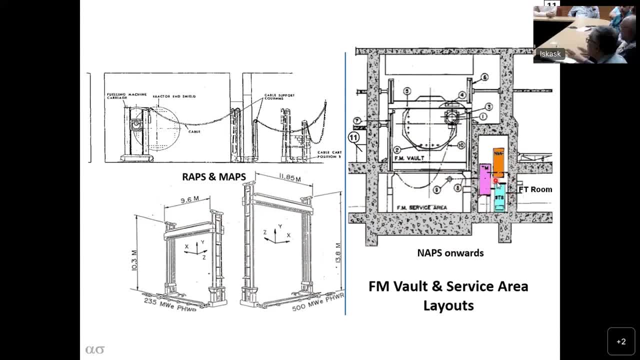 and put it into the bay that is spent fuel transfer system. all of this will get changed now. this, these three equipment here, are totally different, hundred percent different, from what is there in wrap one and trap two or map one and map two. this is totally indigenously designed in npcr. 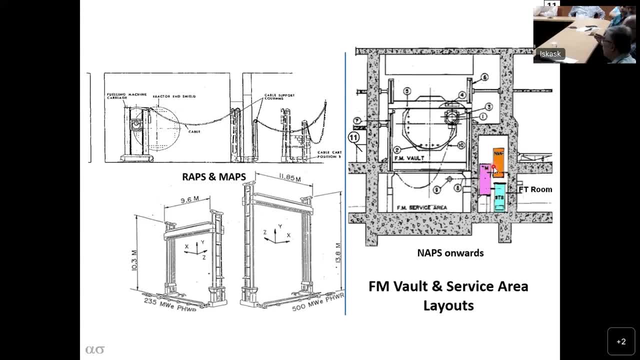 and made here. so this is the, i would even say the first of a kind in the can do world. uh, it is like that now, once we have done this, future 220 megawatt reactors, all of them are following more or less the same layout, and the same uh uh configuration has been followed in the others. so 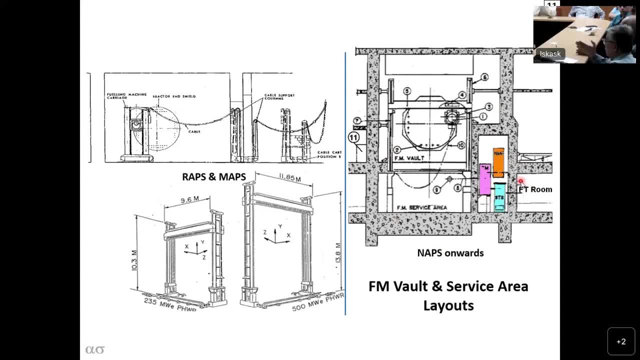 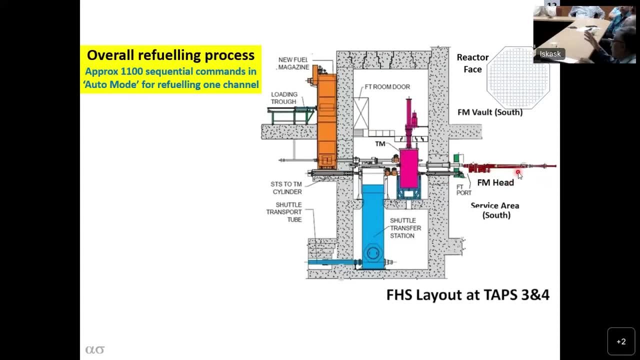 you. once you do it, it becomes helpful for others. so that is how we are able to build so many reactors. now i will explain to you how the fueling is done very, very briefly. this is the fueling machine. our entire idea is to get new fuel into this machine. the machine will go up here. this is 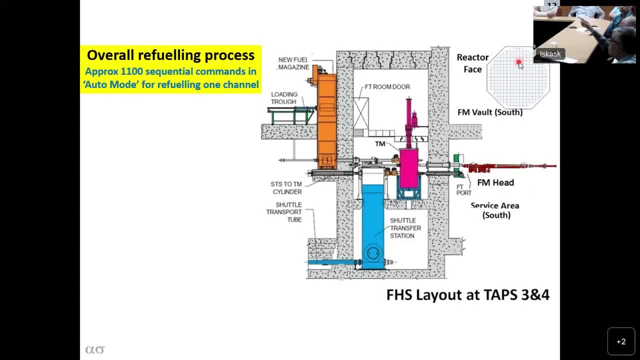 the reactor. this is, the channels are there. you push it into that. the machine at the far end says we have north and south. we call it north and south. so we are in north, the other side is south. the south machine will receive the spent fuel. but the spent fuel bundle again. it has to come. it has. 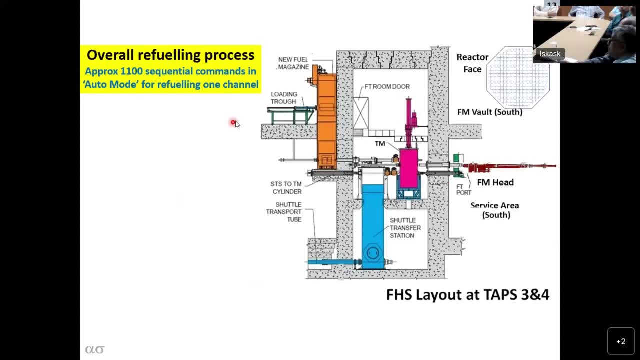 to find a way to send it to the bay. so that is what we do. so here, bundles sent by nfc in the are brought into the reactor hall and manually lifted one at a time and put it in a trough. this is only manual operation. two bundles he will put and push it into the vessel called. 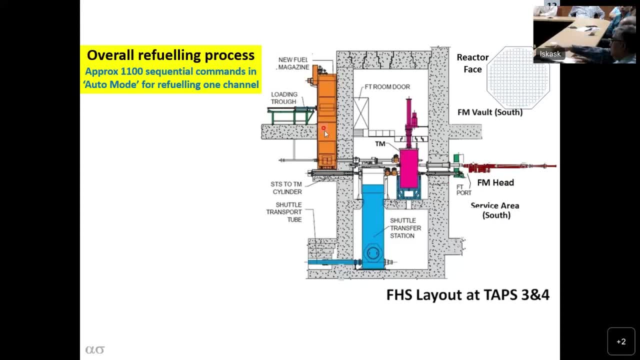 new fuel conveyor, new fuel magazine. then from there the level is reduced and it has to come to the transfer magazine and from the transfer magazine it will go to the fueling machine. now this is a new thing here: the transfer magazine is a eight tubes in our 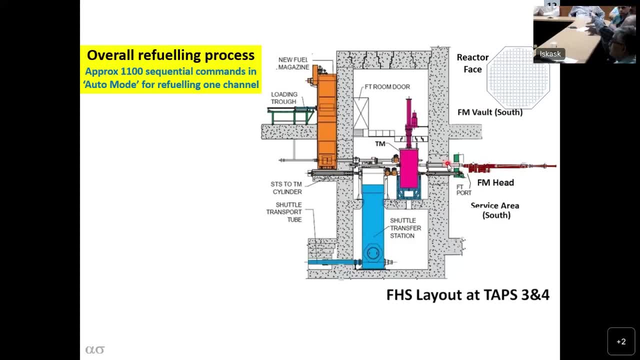 magazine. out of the details it can take six tubes in a vertical magazine. it can take eight bundles at eight, four pairs and it has one empty tube. so when it aligns it takes in the empty tube one pair of spent fuel bundles and sends new fuel bundle in the same thing. so this: 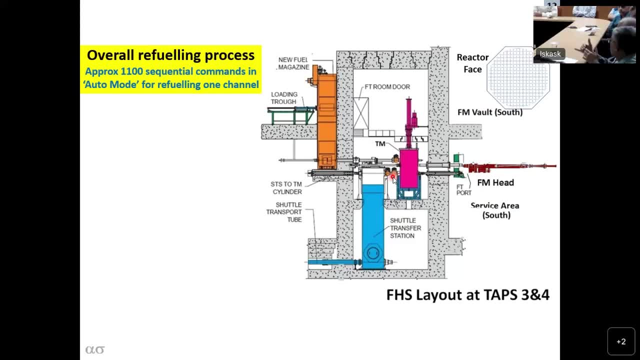 is an exchange program, that is, you send a spent fuel bundle and receive new fuel bundle. okay, so this is the, this is the scheme here. and then from the transfer magazine you come down to, uh, the spent fuel. and then from here, this is a different scale, this is the transfer. you put the. 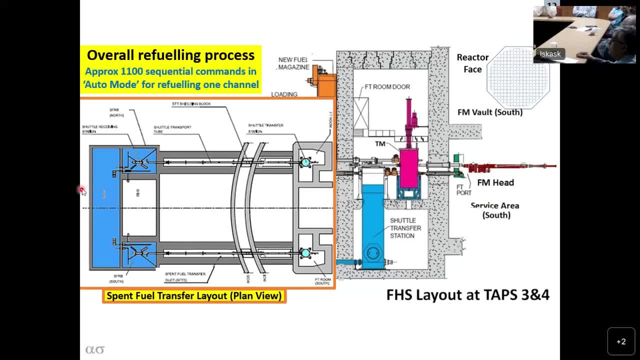 bundles, two bundles spent fuel bundles- into your tube and send it with water pressure, like you have pneumatic in france, where post office you will send letters to for for compressed air from one place to the other, similar to that you have here with water pressure. you send it to the bay. in the bay there are equipment which will take it. put it in a trace. 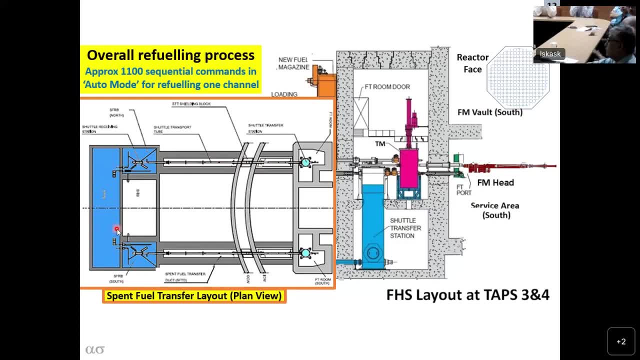 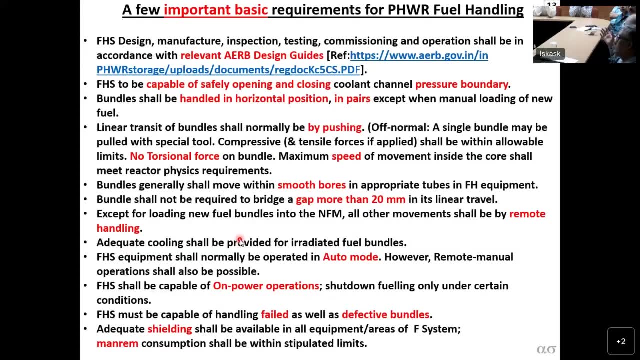 and put it stored into water. so this is the basic process. how new fuel bundle gets into the goes through the reactor will come to the base. so now we are in a position- uh, we are in a position- to derive or enunciate some principles of fuel handling. what is it a? 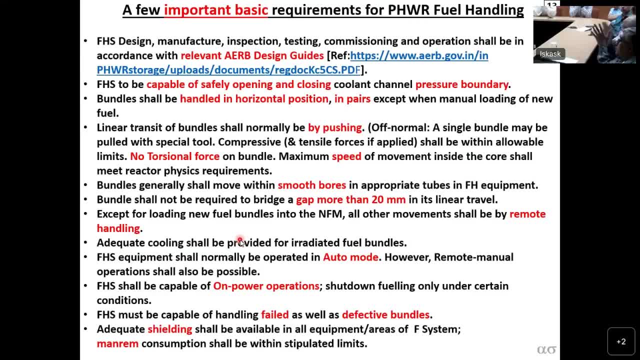 a, you have to handle two bundles at a time in automatic mode. b, you have to handle the bundle in a horizontal mode. and. c, you have to only push the bundle. you can't twist or you can't rotate or anything. you can pull the bundle at specific times for off normal. 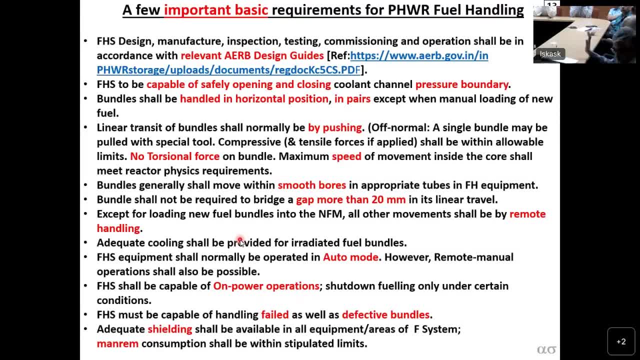 operations, but only one bundle, otherwise you have to push only two bundles. now the bundle, as you can imagine, is fairly fragile, so the compressive load you can put on it is limited. so the machine has to make sure that it doesn't put overload the bundles, so they actually 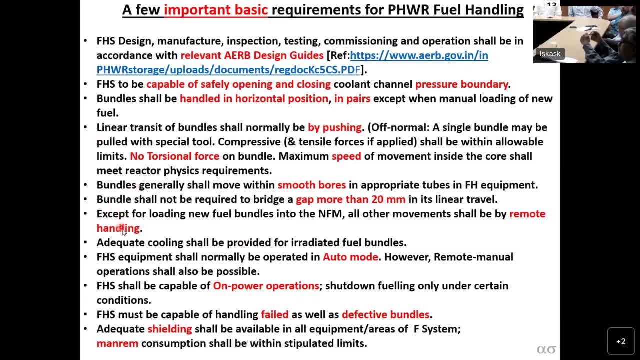 the requirement is that two mechanical rams cannot compress like this. so if one ram compress, this has to be only hydraulic, so that it will overhaul. so this is very important. uh, these are some of the. of course, everything is superseded by an aerb guide. any fellow who is designing 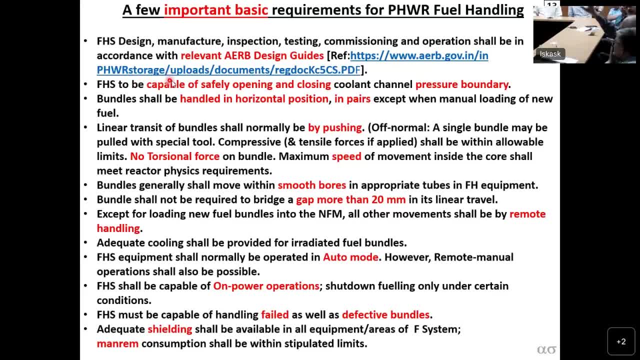 fuel handling system has to first meet the airb guide requirements that is, given that is. finally, the bundle has to be moved inside the reactor at a specific speed. you cannot push it too much because new fuel bundle is got reactivity, so it will. it's not a good idea to push it very. 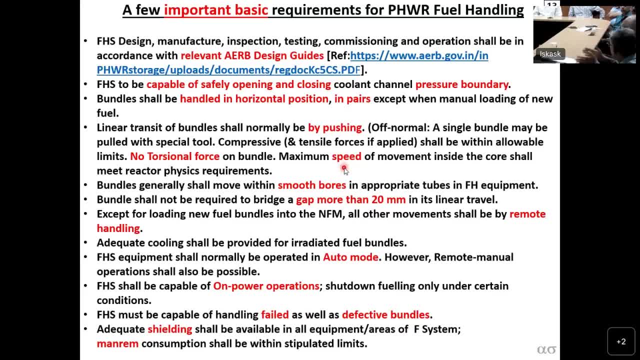 fast, so there is a speed limit, so the machine has to be designed for speed. finally, all these things have to be done. automatic mode: uh, we'll call it automatic mode. other modes are possible, but automatic mode. so the entire thing in the previous slide which i said, 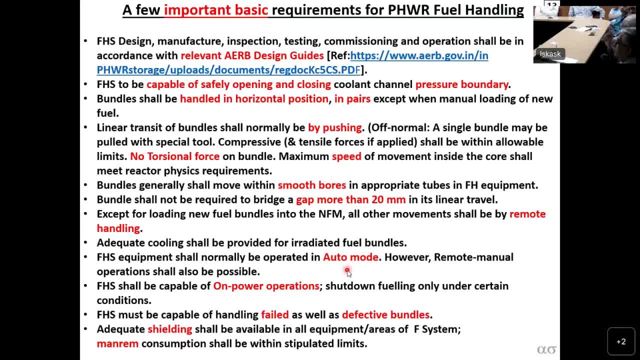 comprises of some 1100 commands. you have the machine. the entire system has to obey 1100 commands sequentially, one after the one after the other. the control system takes care that one command is executed, it is got the correct feedback. only then the next command will be issued, so like: 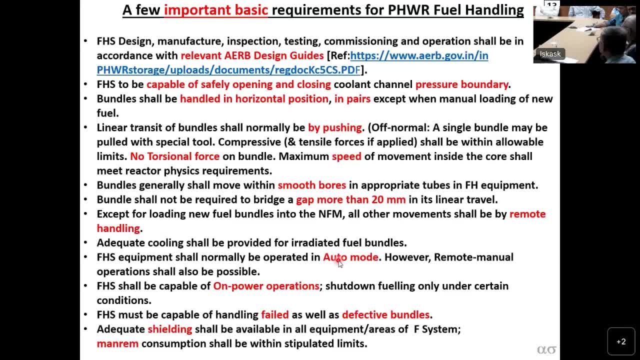 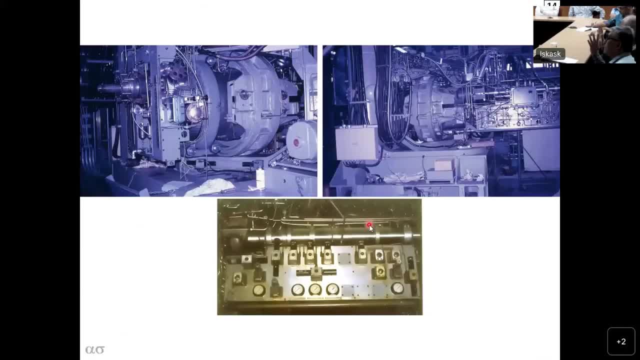 that it goes on a serial mode. yeah, i mean open loop control essentially. so that is, that is over. so now i come to part two. part one is over. part two- i am coming. the top two uh photographs is of the same machine for wrap one. this is hundred percent supplied by canada. nothing doing nothing. 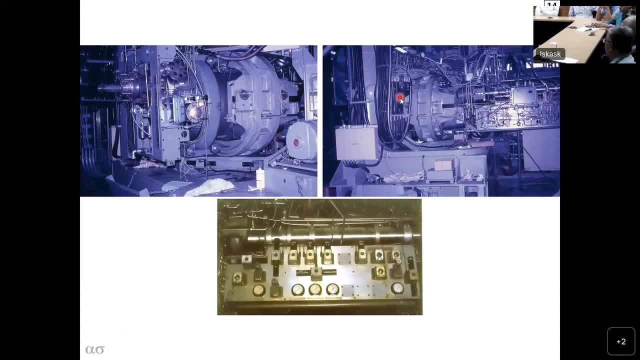 in this. not even a bolt or a washer or anything is indian in this. they wanted to do it. it's all completely canadian. uh, then we were sitting in: uh, bombay, i was in red at that time, mr mcconney was my boss, so, uh, then others, we were very keen. 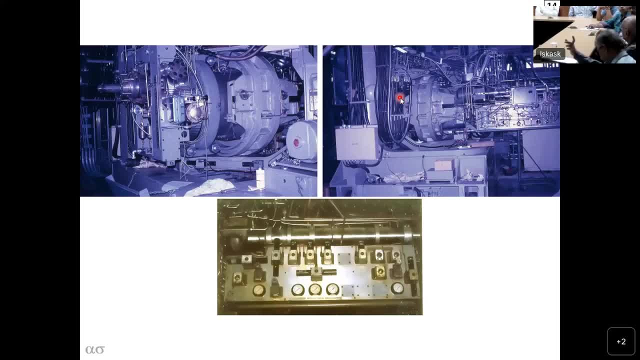 that this fueling machine should be made in india. mr vt christian, all of us were very, very keen that we should be made in india because it's a prestige issue. it's a prestige thing here which is a high technology. it should be made in india. canadians were saying everybody: if you do this, you will. 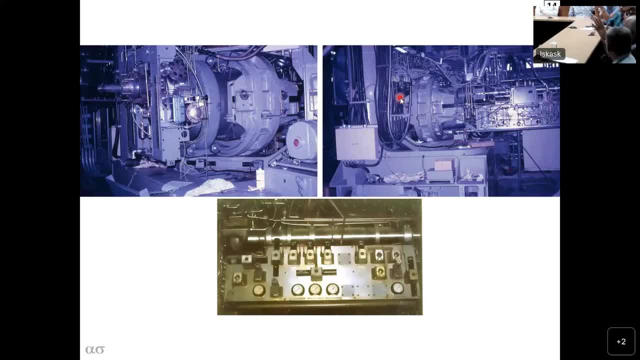 not be able to meet any schedule, so you forget about it. we will give you a rap too. we will give you the idea is, they wanted to increase their content, but we took. then, ultimately, we came to a uh via media. they said: this is called the ram assembly, this ram assembly. 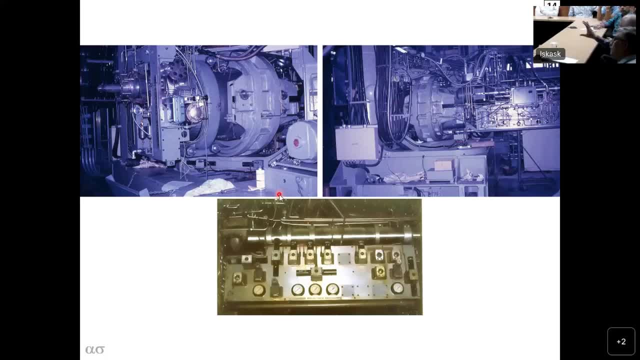 is a part of the fueling machine head. i will show you later. it is approximately one third of the entire mission. they said you make this first, as we call it. if you make it successfully within time we will let you do the other machines also. balance: three machines are required for rea. 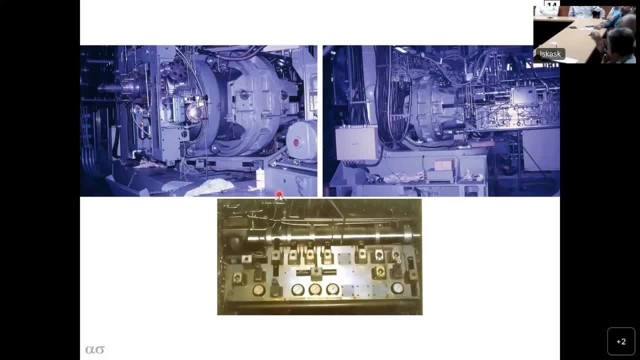 ter. so remaining two and half machines. we will allow you to make this. you make this one here. so central workshops took this challenge and they did it now here. what i have would like to show is that this is the ram assembly is here. i'm only talking about the mechanical components. 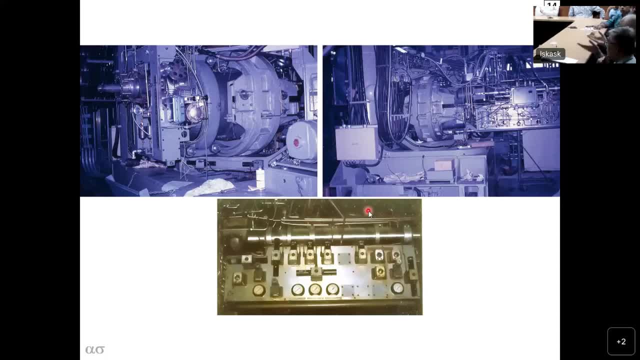 it has got so many appartenances. it has got so many control elements: directional walls, pressure gauges, switches, you name it. everything is there in there. this is controls for the spare ram assembly 75, india. we were not making any raw material in india, so all raw materials, all standard components. 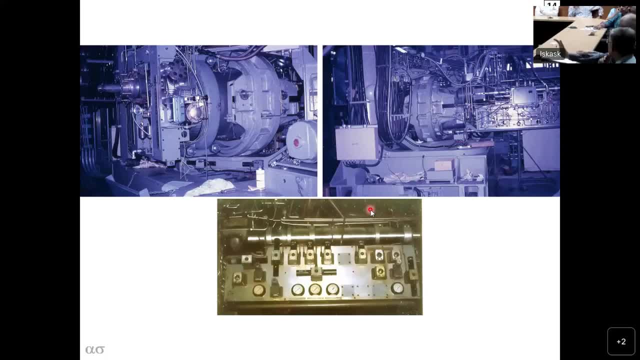 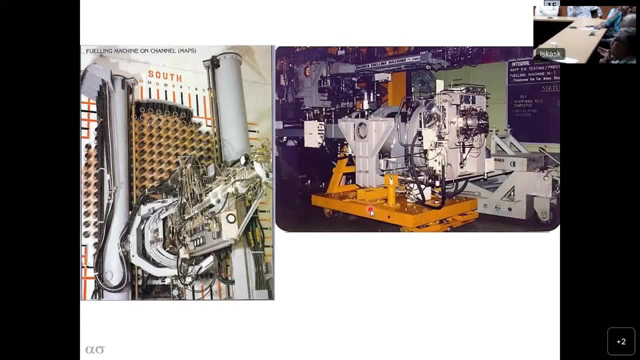 were imported and only manufactured was india. so that is what we did then, slowly, once somebody success succeeds, like central workshop succeeded, then others were interested in taking up also other private manufacturers. so slowly we started manufacturing. so central workshops manufactured more heads. we were able to find more. 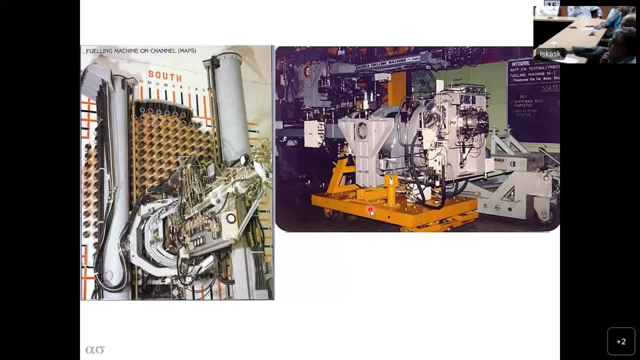 contractors, machine precision machining, people to do so. ultimately, this one which you see on the left hand side is the ninth fueling machine head for madras two. so rap two, rap one and madras nine fueling machine heads we did probably in about 10 or 12 years. life used to be very difficult. 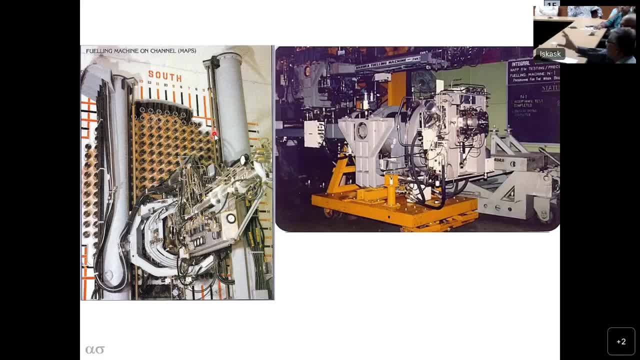 we were struggling, struggling, struggling. anyway, we did that much of it because of central workshops. then when we came to narora, by that time we needed to re-design a very important component which will come later. because of sanctions- by the time- 1974 onwards- we had a sanction thing- we were not able to get many things which we were otherwise getting from america. 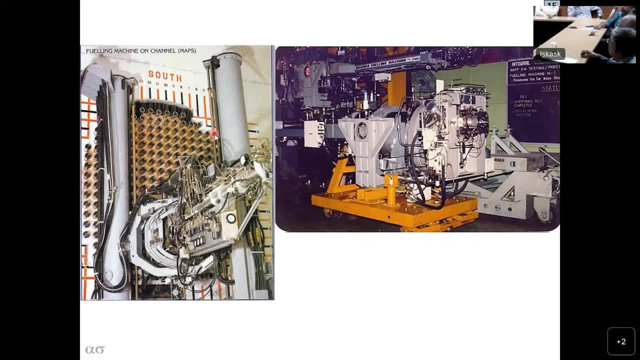 essentially usa, but we were. when usa refused to supply, we found alternate suppliers in europe, but ultimately that also dried up, so we were obliged to do everything ourselves. so the naroda machine, this is naroda now. uh, all, all fueling machines from narora onwards up to rajasthan, 5 and 6. all uh 16. 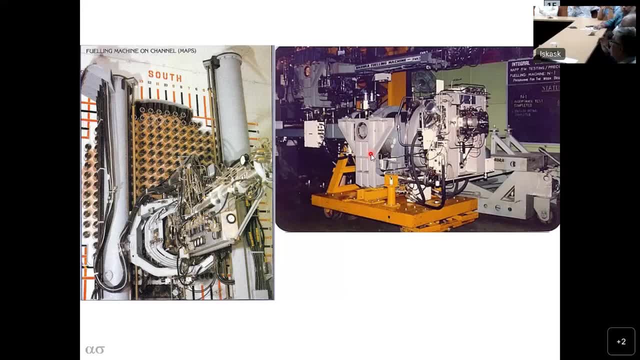 16 machines. all are this design. ultimately, totally this design is: 22 fueling machines are operating now in india, which has been made. so from 1975 to 2020, you can take it. so this is the progress we have had. so that is what it is now. next to me, this is the 500 megawatt machine, the 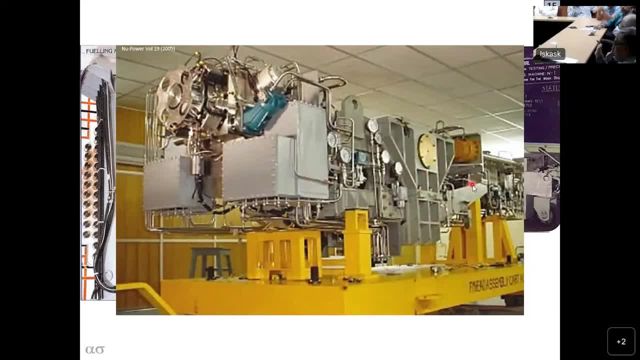 final megawatt machine. i think most of you will know we were working in s71 in 1985 onwards and at that time the control regime was too much and we had some several other feedback, also operational feedbacks we had. so we wanted to plow all of that into the 500 megawatt machine. 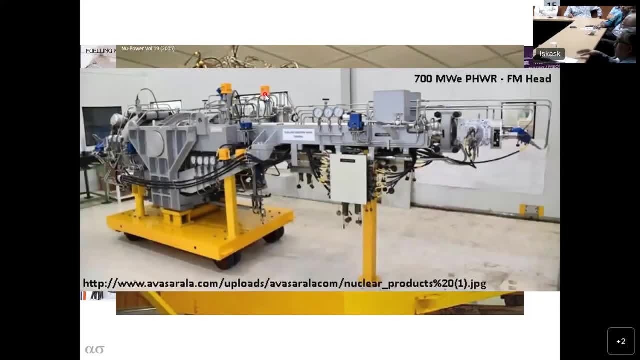 and that is what it is. i will come to that later in a minute. and and subsequently i retired in 2001. but my younger colleagues have gone far, far ahead compared to that and this is the 700 megawatt machine they have made. so i would say that now in 700 megawatts- 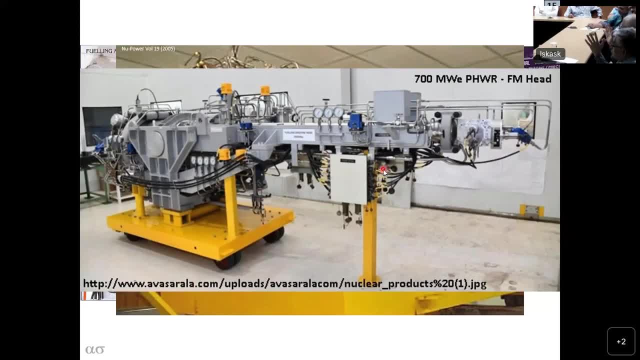 nearly. indigenization of the mechanical parts is to close to 90- 95 percent. design is 100 percent, manufacture is 100 percent. uh commissioning, testing etc are all 100 percent. but manufacturing some components and getting some uh control elements- we still have to get something from there. all of 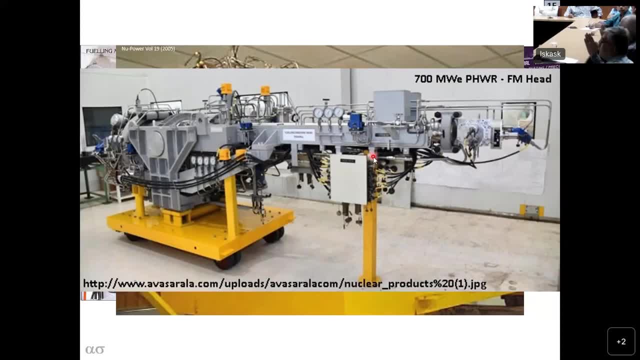 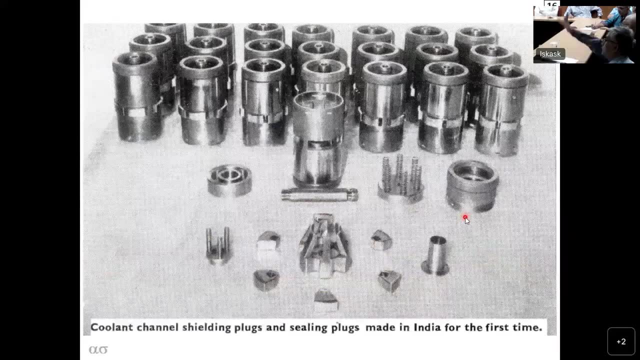 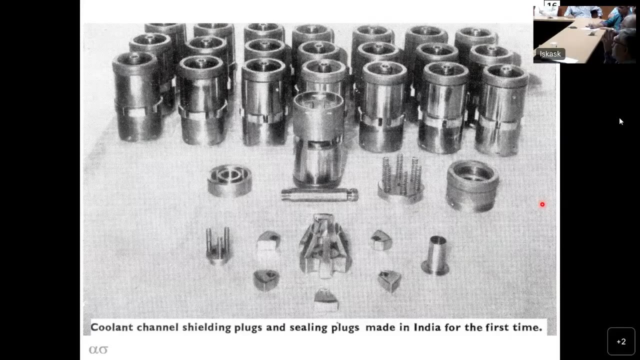 those are not made in india. so i would say, mechanically, if you take the indigenization is to the extent of about 90 percent, 85, 90 percent. so next one. now we come to this. i talked about ceiling plug. this is the prototype ceiling plug 25 first numbers. we made 1980. first number: 25 plugs. 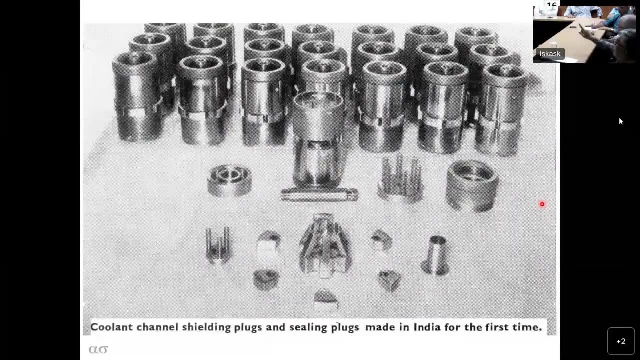 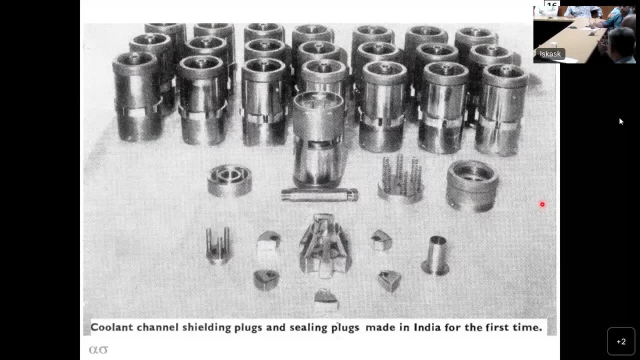 why it was made like that, because a aecl said no, no, you cannot make fueling the ceiling plug very high technology. you cannot make it central workshop anyway. did not have the machines for it and they were not. you see, some 625 ceiling plugs are required per reactor. central workshops are not. uh, 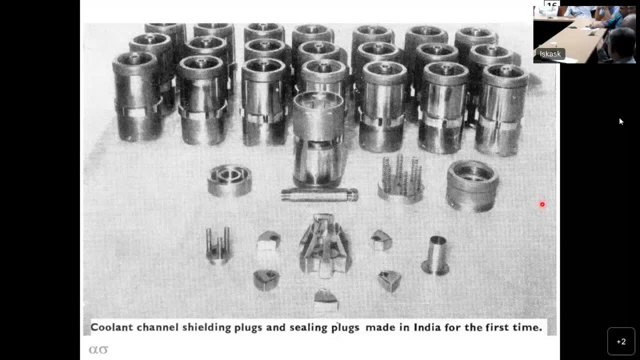 attuned to mass production. they are generally make one or two like that. so and anyway, some very important machines required for that were not there, so we had to go to private manufacturers- in this particular case it is cooper in satara. so we got there. they made these machines, these ceiling plugs. we will talk. 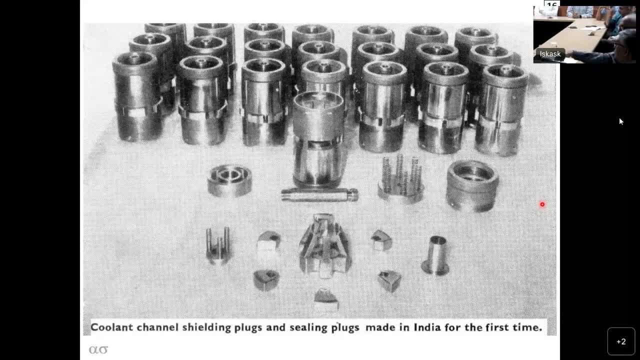 about the ceiling design in a minute, but this picture shows all the components here individually, 125.. so aecl said: you make this first, then i will allow you to make it for rap2. uh, we could not meet the schedule for rap2 so, yeah, i think you have to. 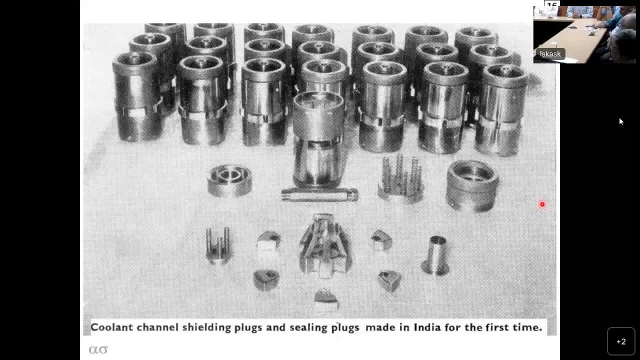 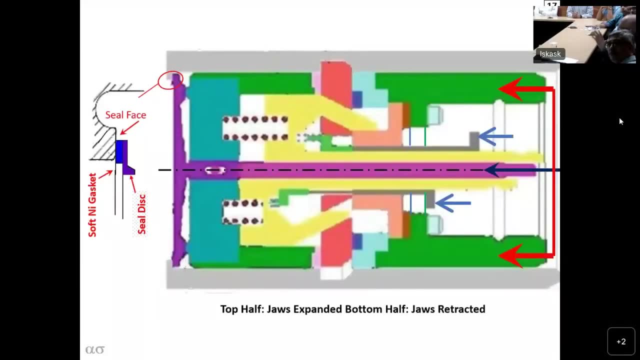 please. all came from canada but from map onwards we were obliged to make it here and we did that also report. now this is the ceiling plug is a very fantastic design. what you have is: this is the end fitting. this is the ceiling face here in the end fitting here. so this is 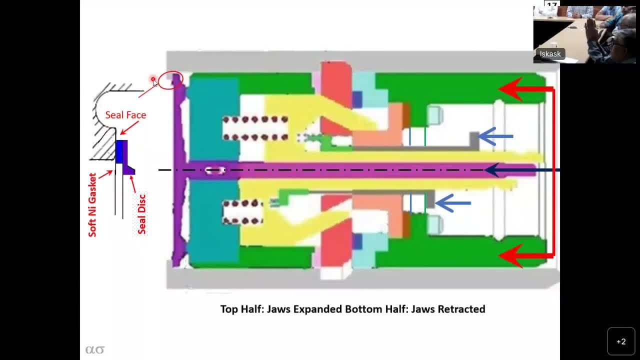 a ceiling face there is a disc. the disc come, you have to compress. the disc has got a uh gasket. you have to press the disc against the stationary ceiling place. what you have. what is the criteria there? the contact pressure that you have to get should be greater than the heavy water pressure inside. this is the requirement. so how to put the? 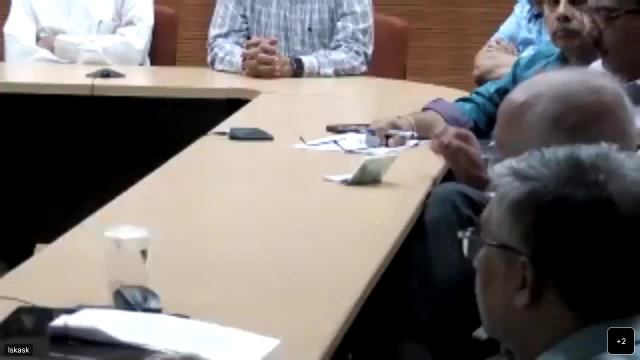 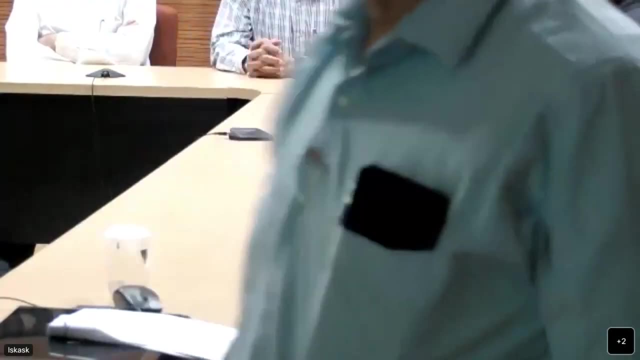 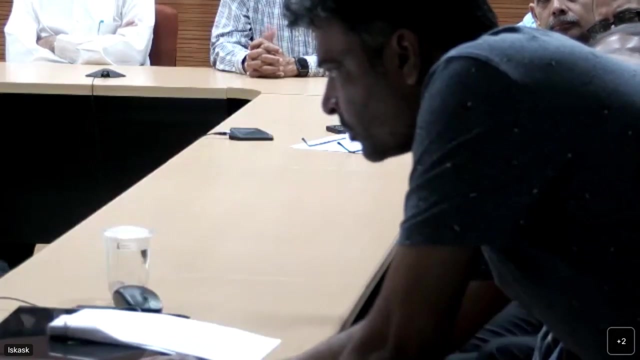 ceiling plug, compress it against the ceiling face and then lock it in place because fuel machine has to go away after installing it has to go. so see, yeah, fuel handling, uh, engineers, particularly at site, is dread is that the fueling machine is clamped onto the channel. 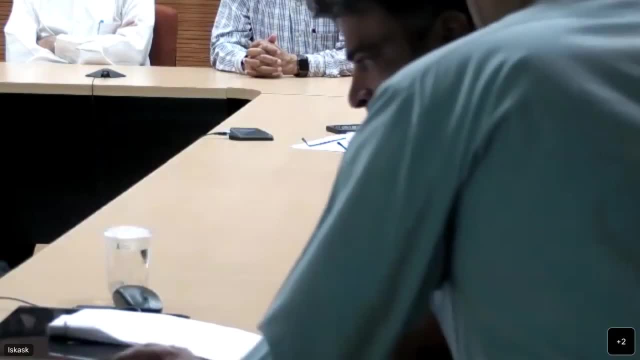 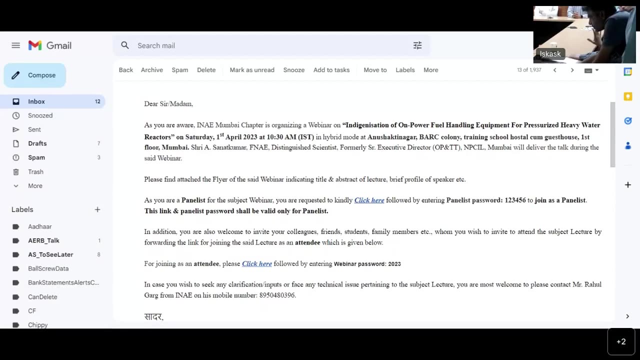 and it doesn't come out or it is not, you're not able to proceed with the operation, which you call it hang up. so this hang up of the fueling machine is the dreadliest thing. so when you when you reach that, you're obliged to shut down the reactor. very often you may have to. 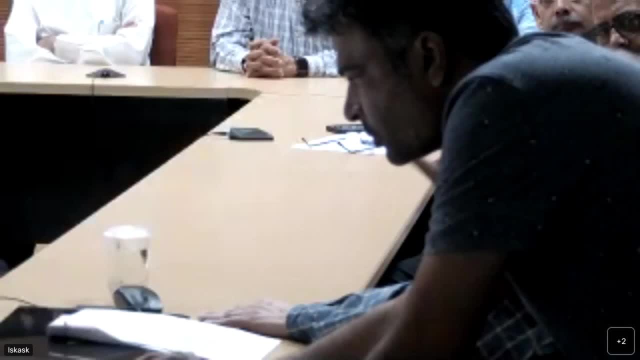 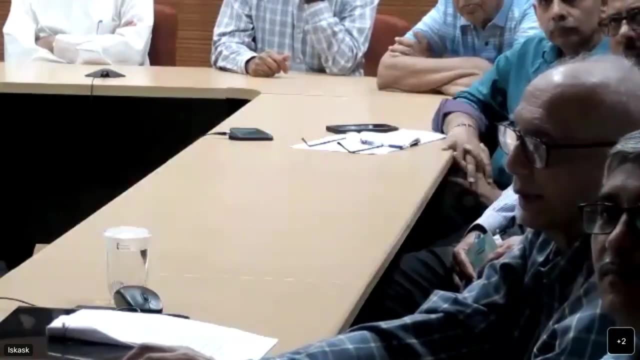 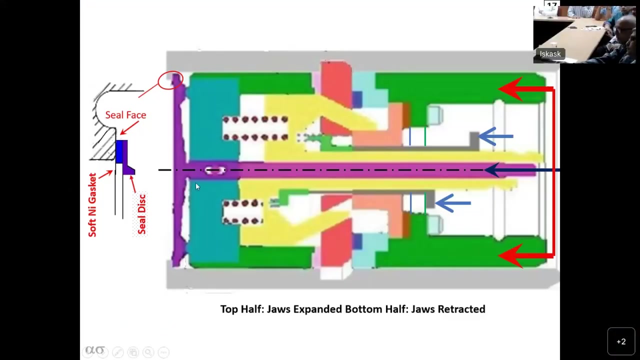 cool and then go access the vault and then do repair. nobody likes to do this, so okay, so this plug has to apply your force on this. this is the disc which i was telling you about. it has got a nickel gasket here, as shown here, so you have to compress the nickel gasket. so this is the body of the ceiling plug. they got a very 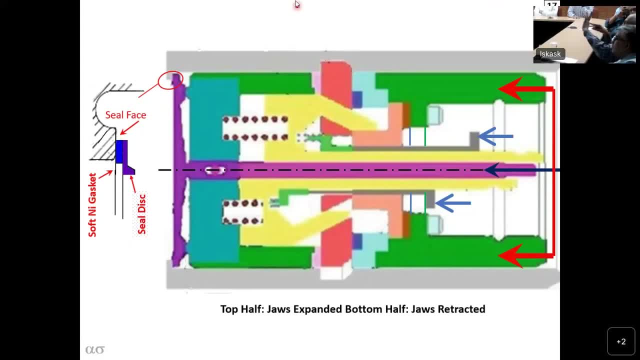 brilliant. if you have a disc, you apply, you need to in order to apply a force here. they said, okay, you need so much deflection so your disc can be compressed with the least amount of force. what they did? they applied the force in the center, obviously in a beam. if you apply the force in 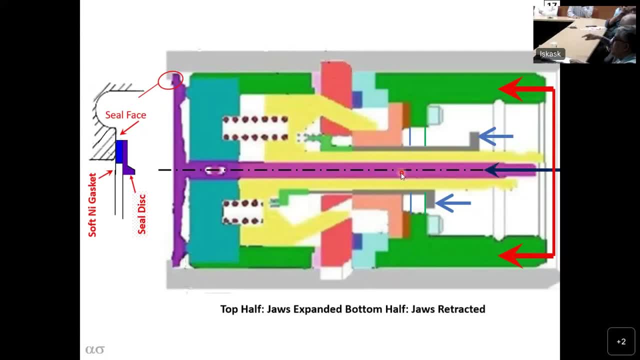 the center. it has the maximum deflection for that. so this is the body of the ceiling plug. then that is smart enough. you apply it on the, on a reaction point slightly outside and then lock it. so new in this picture i will show that locking again. you know, in this picture the upper part, 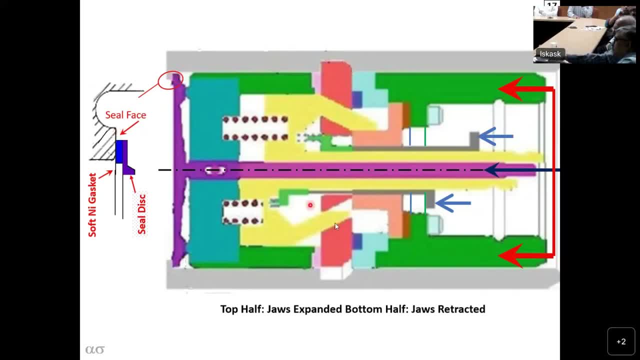 shows the plug lock with the force applied in the lower part. it shows the plug, the the jaws. it is like a self-centering kept jaw. the jaws are initiated because the fueling machine can bring it like that. next training. this one shows how far can the fl optional since the fueling goes. 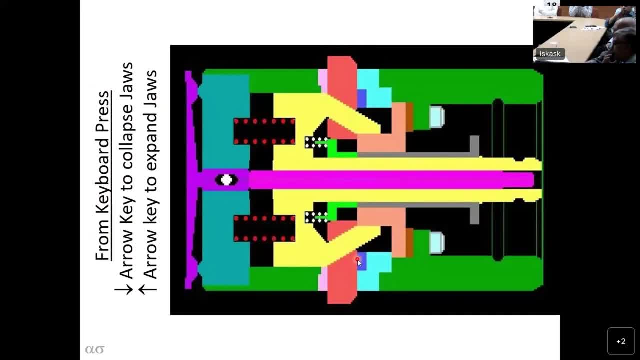 weed and źqwards yourself. this one shows how quickly what difference you size. this is because shows how the jaws operate. see here: if you push this, you push this stem with the ramp. the ram has got the ram assembly has got three coaxial rams. so 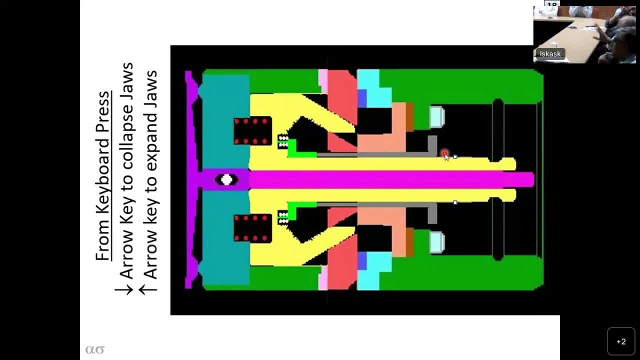 using that upside down, vertical, whatever you want to do, several complicated operations. if you push this stem here, spiders and yellow piece here, it will go and then, in order for it to come out, you take it out. so this is just a push pull, this is push pull. yeah, ACL had a ceiling plug design in their NPD and 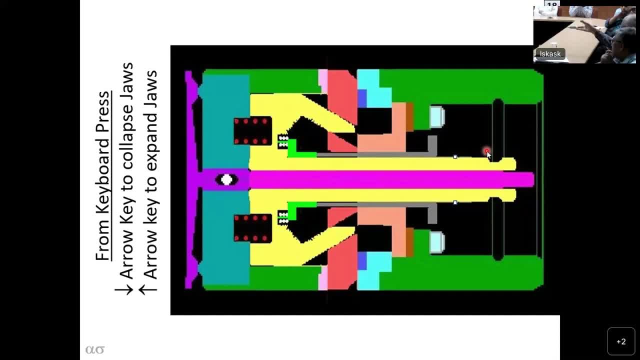 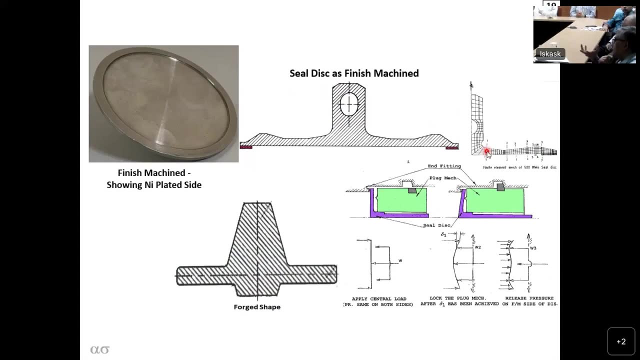 others where there was a turning was required with acne thread. but one of the design requirements for can do this in design was that there should be no turning repair. so this push puller- now this is this is disc which I was talking about with the sink- has done a lot of help for us. this is the disc which is forced it. 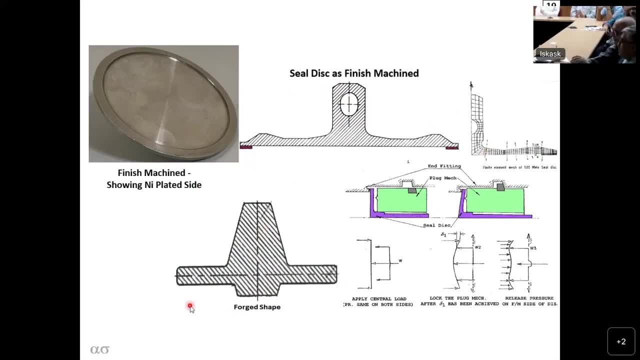 cannot be. it has to be for, for metallurgical reasons it has to be upset porch. it cannot be machined from a solid bar, because the grain flow lines will not be correct. and then the loading is there. so the stress analysis for this is done by dr Singh here, and then it requires nickel plating. this nickel, 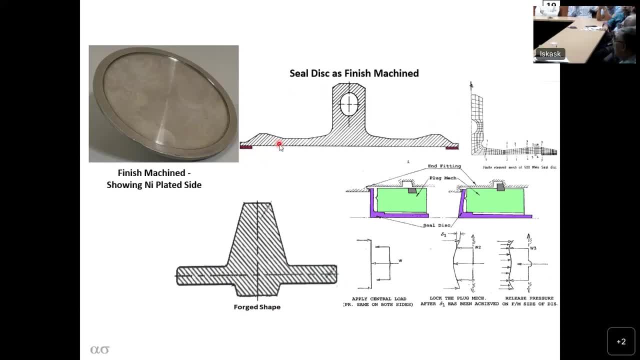 plating gasket is called soft nickel gasket. it is about two, two and a half millimeter thickness in a technology in itself. so that person developed ultimately and it has got soft nickel, one earth, 170, VPN or something like that. that is the kind of 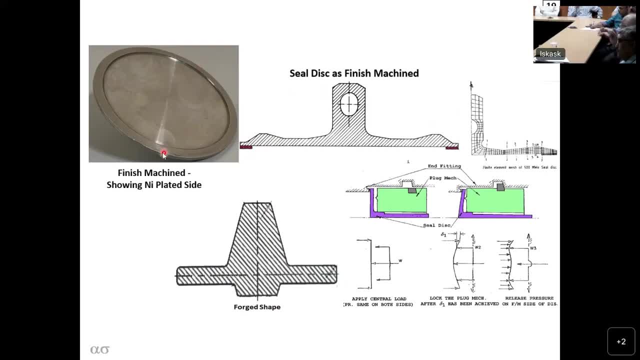 procedure, so that you can see it here. that is. it is. this were all. it is a do or die operation. we have to do this. if you don't do this, you will not get a reactor kind of thing. so that is what it is. so now we go to this. now, this is an 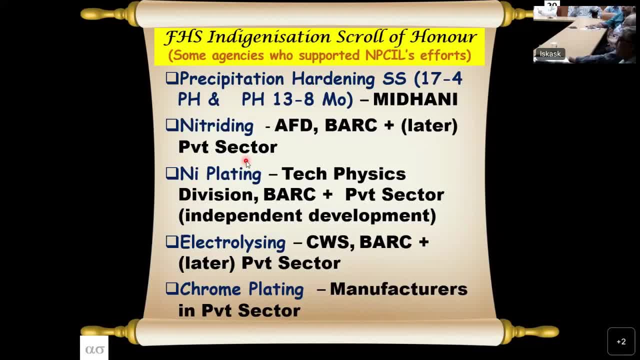 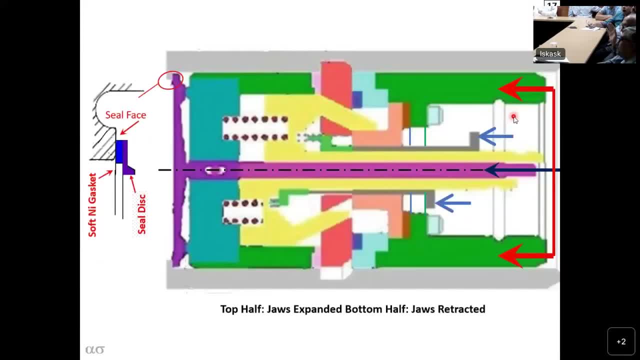 appropriate time, which I think is appropriate time, which I think is appropriate time, which I think is appropriate if we use it. you, we need proper stretch here today. you got this one here. we have only the water pressure gauge in the inhabitation, and here is. shall we have Rachet? 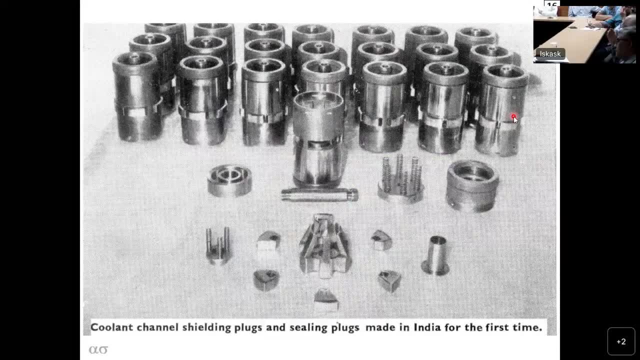 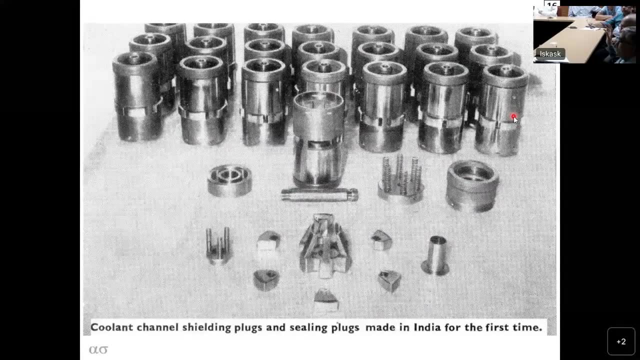 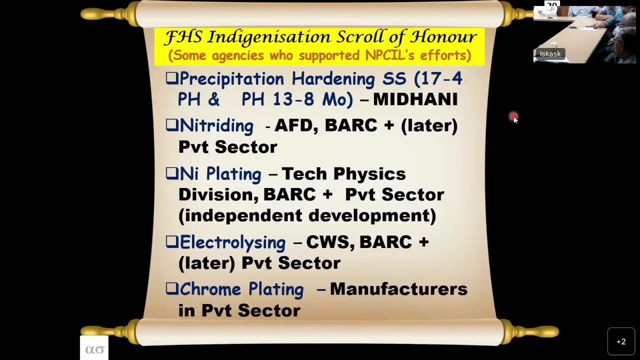 itative pressure gauge is on a impact, low temperature, null dictility is very high. so many other points are there in that. so when we started with rap 2- nothing doing- there was no way in which there was a. in fact, even stainless steel was not made in those days in india. so this precipitation, hardening stainless 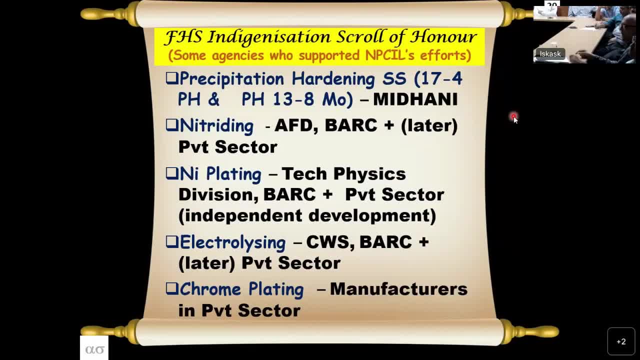 steel and then later on, a better variety of that called 38 phmo was also used. the 500 megawatt uses the 35 megawatt and 700 megawatts use the 38 phmo. so these steels had to be developed. this was done. 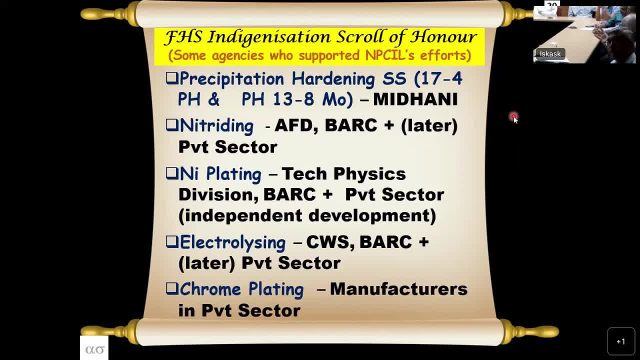 by midan uh. they developed a demo. they from the astm uh chemical compositions. they did, and initially they found a lot of problems with davies, along with them bb also. they were not meeting impact requirements. then they found out the secret: the columbium plus tantalum control is required for. 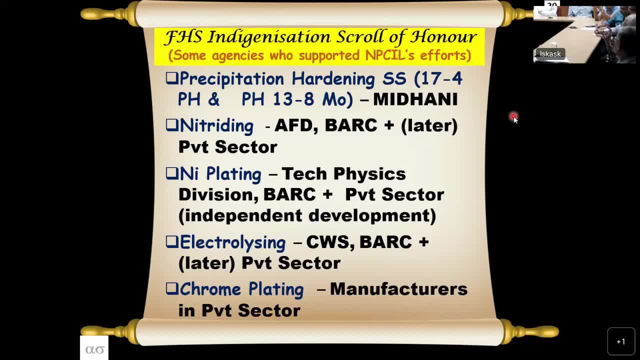 getting the impact, so they- it's a kind of a now they are proprietary information for them. i don't know what is that combination, but it is required, so they have done it. now since then, since about uh narora time, all our requirements are being met by nidani. nidani has done a very, very terrific job now. 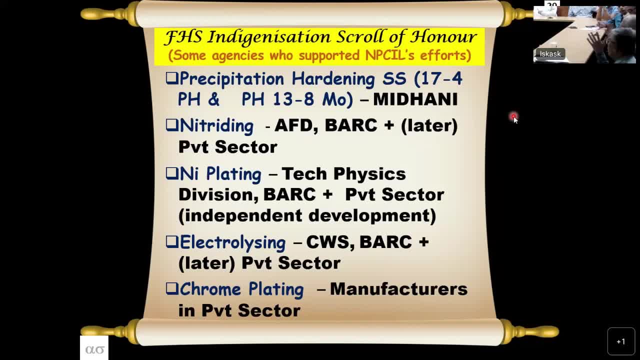 next comes this nitriding. the problem with 1742, problem with in swelling machine head, is that it has to work in water, which means corrosion resistance is required, which means stainless steel is required. stainless steel cannot be hardened very much like a carbon steel. you cannot do that, so it has to be surface has to be. 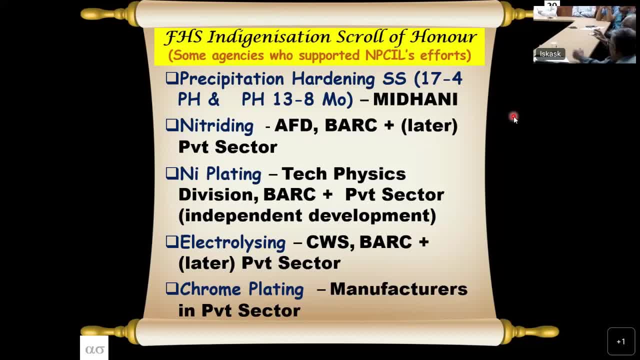 uh, hardened in some ways. surface has to be treated and also a wear pair is 17: 4 ph versus 17: 4 ph is very bad, it will cease. so if you are having a wear, two parts of 17: 4 ph running one on the other. 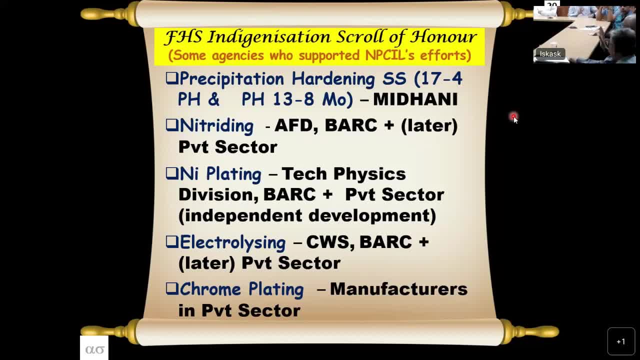 one of them has to be surface treated somehow. there are several methods. one of them out of that, nitrating, is one. this gas nitrating is that you take 17, 4 ph and then apply ammonia to that. nitrogen goes in. the problem with that is that chromium oxide layer. 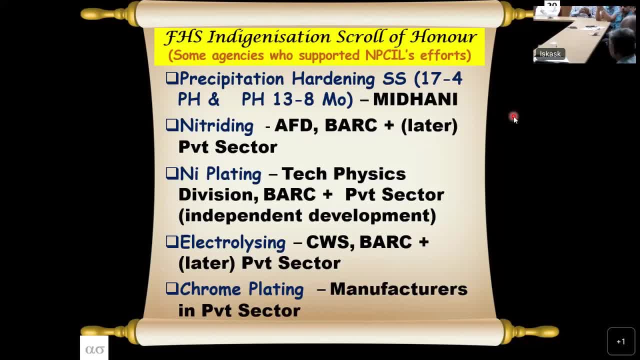 is there in the stainless steel. so first of all you have to break the chromium oxide layer, then only the nitrogen will penetrate. this was done by afd. without afd we could not have done this. the only thing was this is a high temperature operation. uh, some temperature lower than 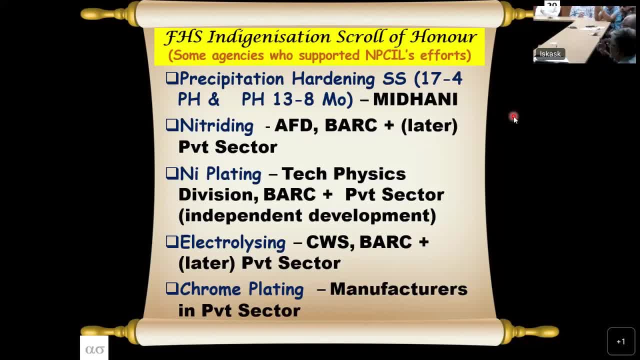 let's say 500 degree centigrade kind of operation. it could not have been done because you are dealing with ammonia. it could not have been done in normal furnaces. we needed to procure inconalex furnace- uh for a thing which we got it from canada, luckily they. 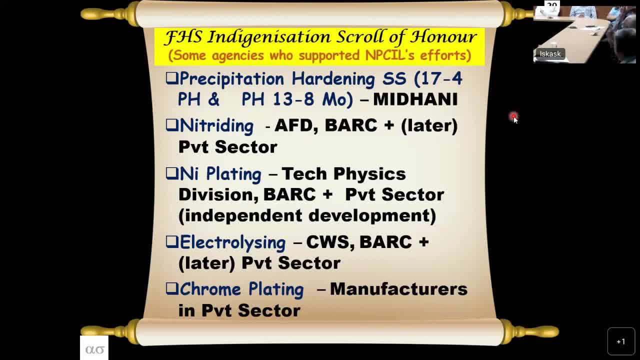 did not know that we are doing this. so, anyway, we got it. and mr tomari, all these people. they have developed this in afd once it was developed and they have now transferred technology to private manufacturers because, uh, ultimately mass manufacture of these components is not going to be done in afd, nor in central workshop. it has to be. 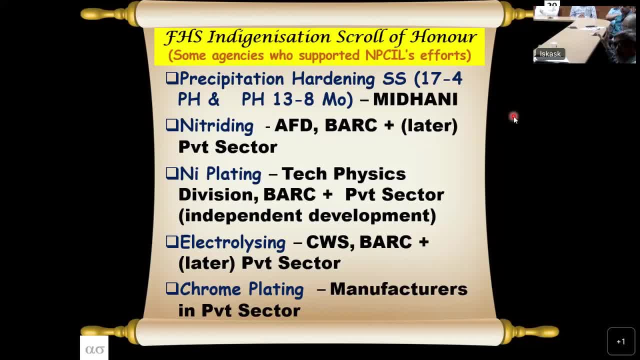 one of the problems we had in manufacturing is that all the required machine tools were not available with one manufacturer. okay, so now that means for the boring operation or a broaching operation or an electrolysis operation he had to subcontract. in those days manufacturer didn't see. 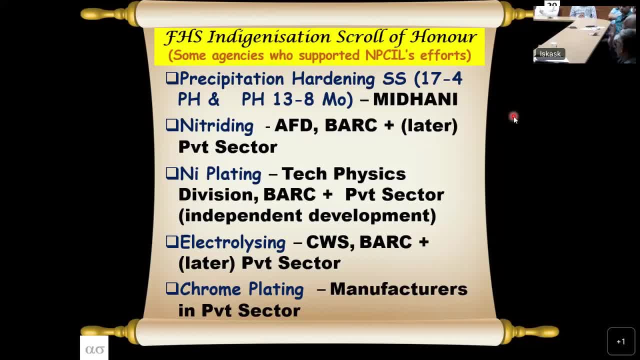 this as a profitable proposition at all. in fact, even central workshop didn't see it as a profitable. we used to do the subcontracting for them and give it. so this is the thing that now, when afd has been able to produce- uh, and then they did a mass thing there also then 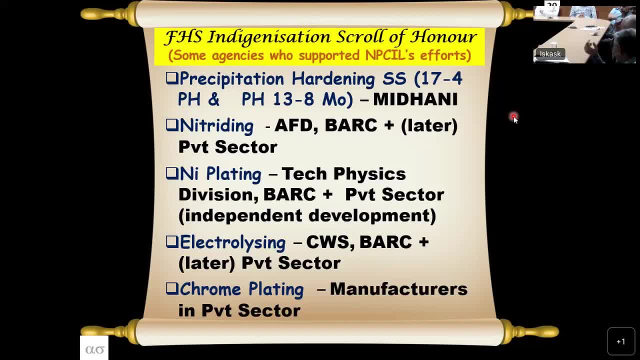 there's the srsl. we will now do it. we can do. you give us the furnace. so we gave them the furnace specification. they bought the furnace and they set it up and it is going on very strongly in private manufacturers. then this nickel plating- i have already told you for the sealed disk, nickel. 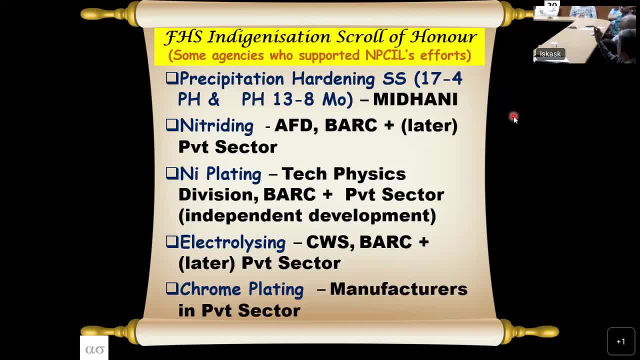 plating is to be done. so sulphur mate bath is required. it is required to be nickel. sulphur made it required to be highly pure. it has to be electroplated. so technical physics division got it helped us in the beginning, and then they were not able to meet the 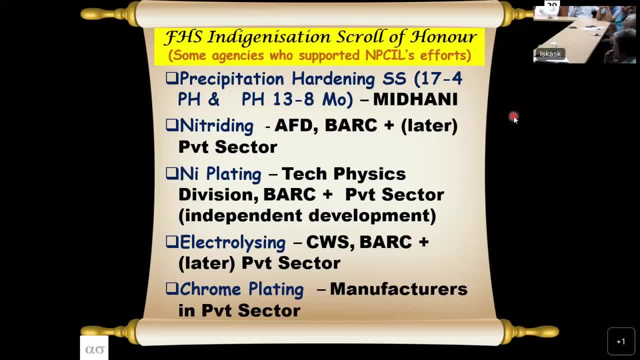 production requirement that we were wanting. so we got others to be in uh drawer and we will. we have got other people to be involved in that and they have developed it now this is now not in brc but in private company. then electrolyzing see is 17.4 p. electrolyzing is a hard chrome plating operation- very, very thin. 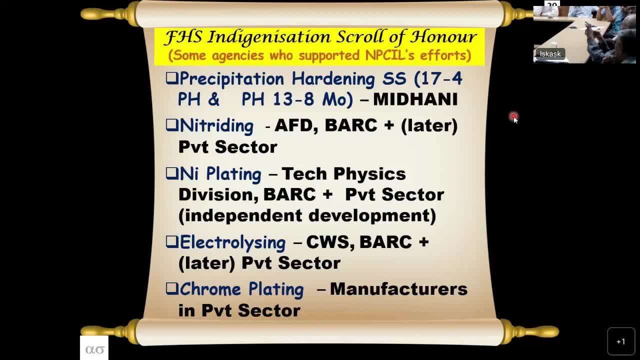 is two microns in electrolyzing, but it has to be done in a bore also. so now what happens is that we were trying with ion plating dr dasanacharya usb that we used to call him, request him to do this. it was not possible, so the electroplating has to be done. for this there is a special salt. 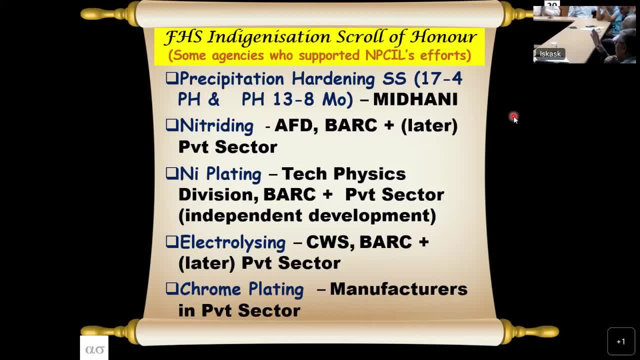 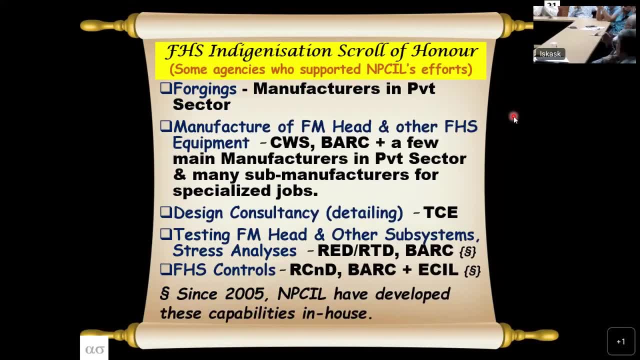 that salt was not available in india, we got that salt, and now the electrolyzing is also done privately. then chrome plating, everybody knows, uh, any, any wear pair requires hard chrome plating. the chrome plating requirement for fuel handling is that usually when you go for chrome plating. 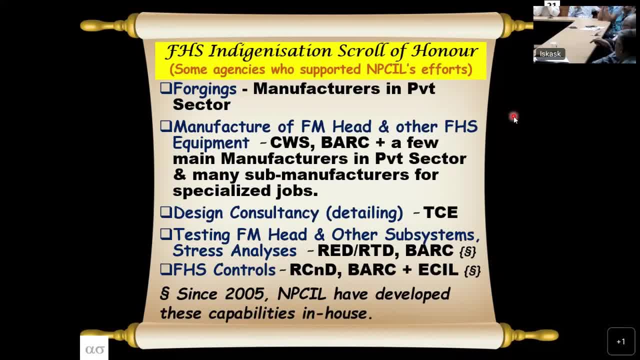 you have a copper base and on top of that you put the chromium plating so that you can do that. this copper is not allowed in the thing, so you have to put it on the virgin metal for this. so this chromium plating. of course there were other people, uh, capable of doing this. then comes the 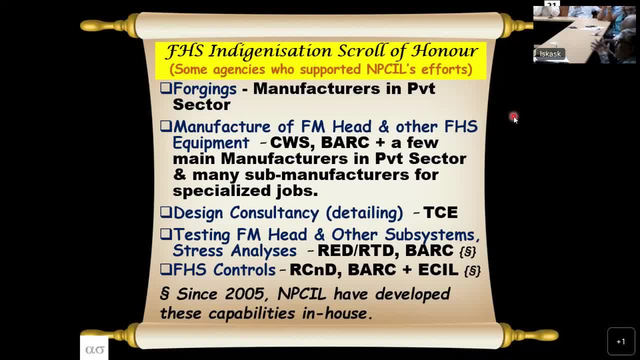 now comes the important point: forgings. at that time, when we were doing, there were no forging at all, nothing, nobody, nobody was interested in this forging business. so we got, earlier we got it from canada, then later on we got it from europe. ultimately, when it came to narora- narora also- we 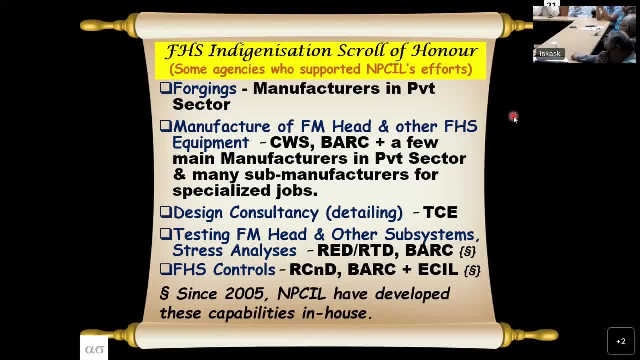 imported. when it came to 500 megawatts, 700 megawatts, they had to indigenize and it has been indigenized. this is the biggest thing. i can tell you. this forgings you will see that polling later- that four things have been indigenized by these people. then manufacturer fm had already talked. 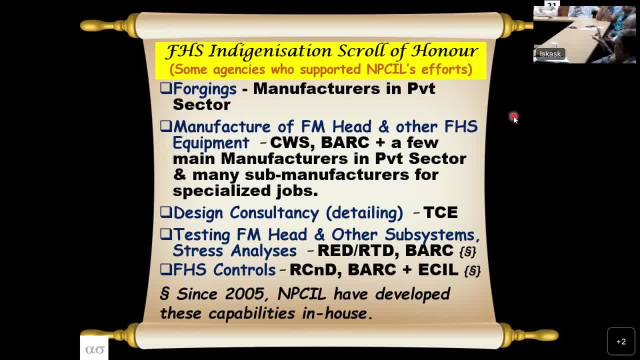 about central workshops are the forerunners. they did everything right in the beginning and once the central workshop started making other people said, yes, yes, we will also do it. so we got it now. then design consultancy, our, uh, our entire process was uh- me and my colleagues, we 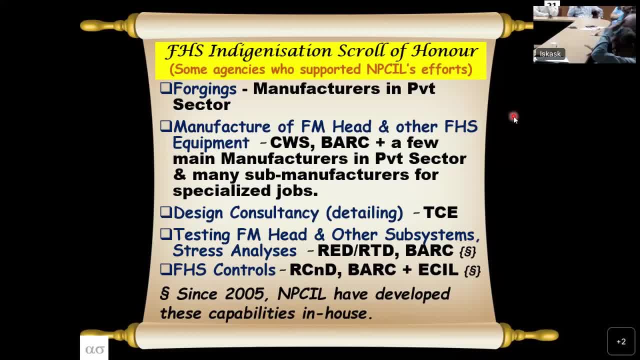 generate the conceptual design and in fact even conceptual assembly drawings and, fundamentally, overall dimensions of one of the dimensions, of individual parts, and we have given it to consultants, in this particular case, tce for detailing. you need to put tolerance, every dimension has to be tolerated. so they established, they established uh standards for drafting. 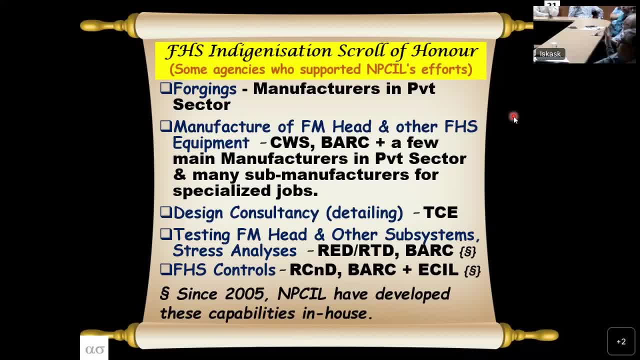 standards and they have done, tc have done. then testing of fueling machines is the next. every fueling machine it got some 500, 600 parts. you put them together then they won't work. so you have. you cannot send it to the reactivation, you have to test it. make sure, commissioning. 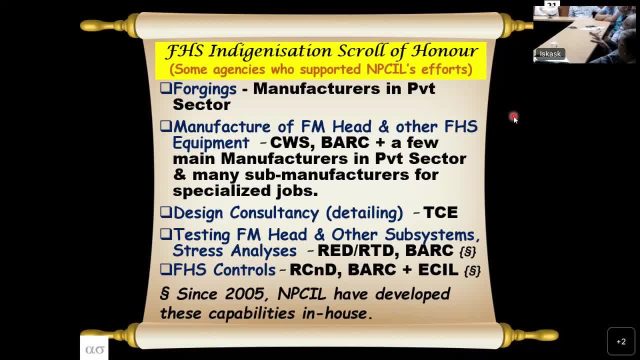 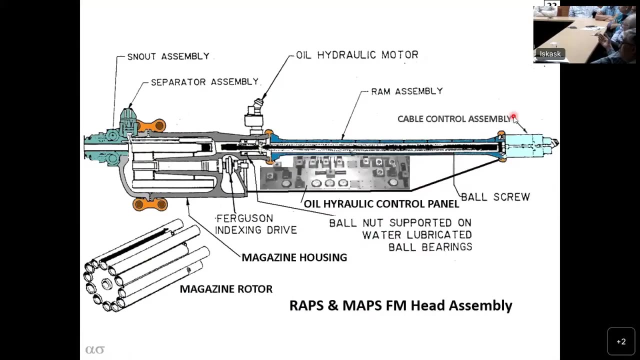 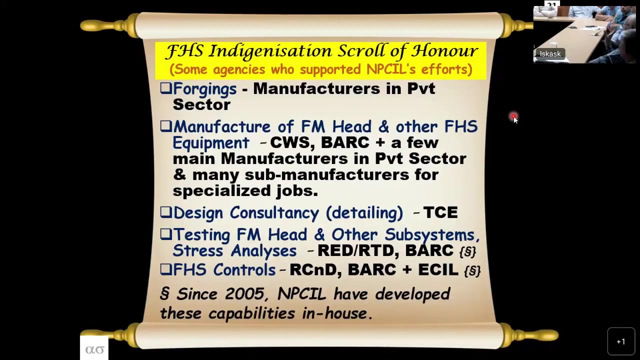 so this testing is being done in uh since 2005. it has been done in uh. any uh npcs. okay, controls. of course we are nowhere- at least i am not anywhere in control business. uh, rcnd and ecil. they did the job initially. ultimately it is now even that npcl has got. 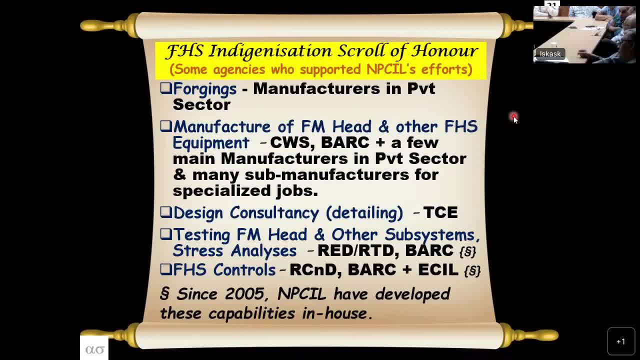 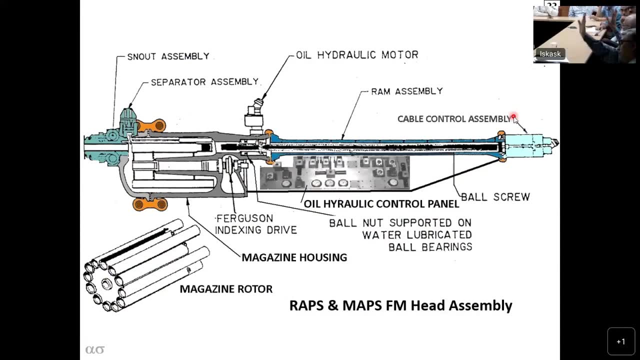 technology established. so this is the uh really scroll of. i think a lot of people in die have contributed to this. now this is the anatomy of the fuel emission. i'm just taking it very briefly. anatomy of the fueling machine as designed by acl. it has got the three major parts here. this is part. 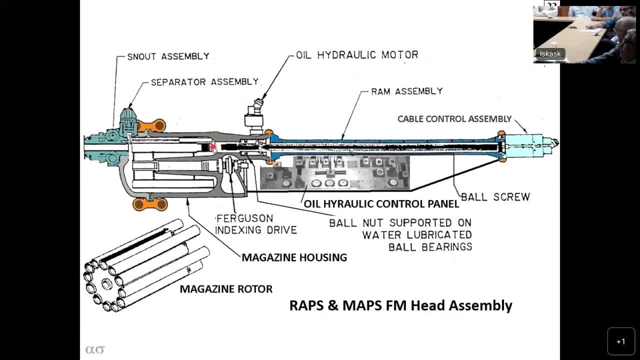 this note assembly. i will miss it. this is called the magazine assembly. in between, that is the forging that was required for it. this is the ram assembly. i have already talked about it, so these are three parts. so, uh, this is the uh ram control panel for the ram assembly. i put it here. 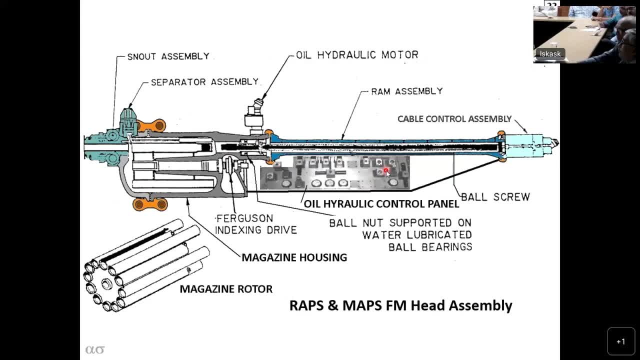 to show that it has got so many more parts here now. this is the uh magazine housing that is. you need to take fuel, spend fuel bundles in the machine, so you have a rotary magazine. it's got 10 cubes. so we will come to that in a minute if time permits. 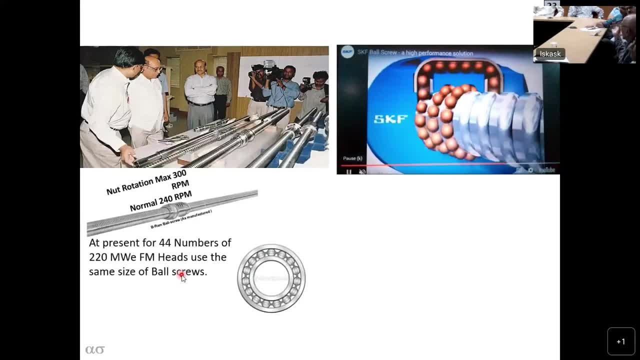 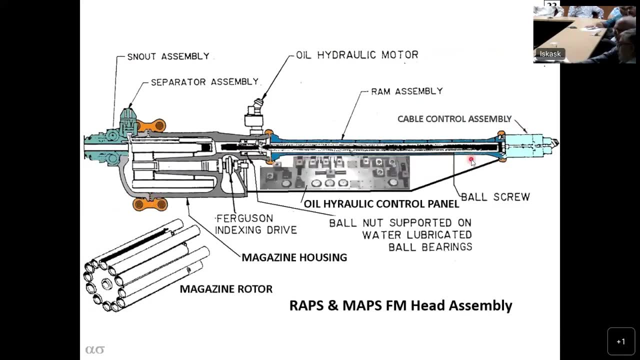 will do, otherwise we'll miss it. now we talked about that, we talked about the ram. so in this here you see this, uh, wiggly, wiggly black thing, here that is a ball screw actually with you see the threads there, ball screw. then inside it there are two more. 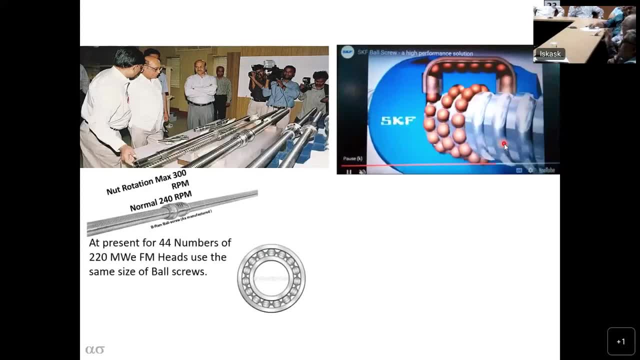 telescopic channels. so this ball screw is very important. it is water lubricated ball screw. even today, water lubricated ball screw in india only one fellow is making. at that time nobody was making anyway. we were getting. we were not able, we were not able to get it from canada. then we tried. 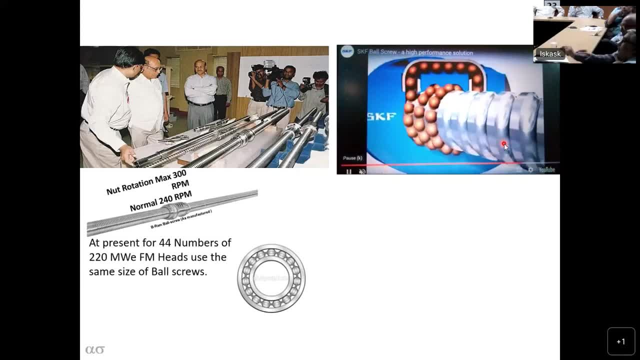 other people, europe, etc. etc. this is the way it works. but this, this video there, is not very accurate because it is only a teaching video. it is only an educational video. it doesn't show that thing correctly at all. there are errors in this, but this is the company which has made balls. what is the problem here? if you? 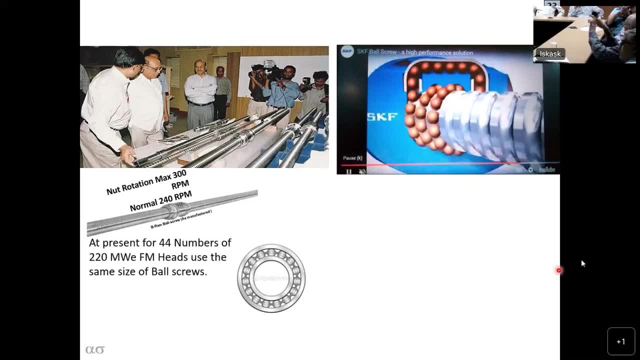 think of a ball bearing. the race is a cloth race, so ball can go around and round and round. it will not go anywhere in a ball screw. it has to go on a thread so ultimately it will fall down somewhere. so you have to collect the ball that is falling down and put it back again here. so that is called. 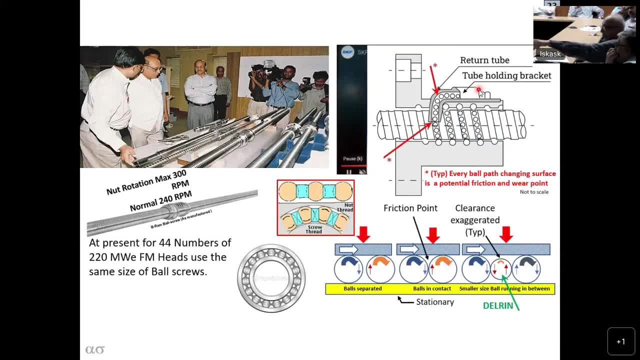 the return tube, next one you should here. so this is the ball bearing. and then this is the ball bearing, the return tube. that is there now. you, anybody knows problem for us, right from wrap on this and until we were testing in thing also, and it used to be a. 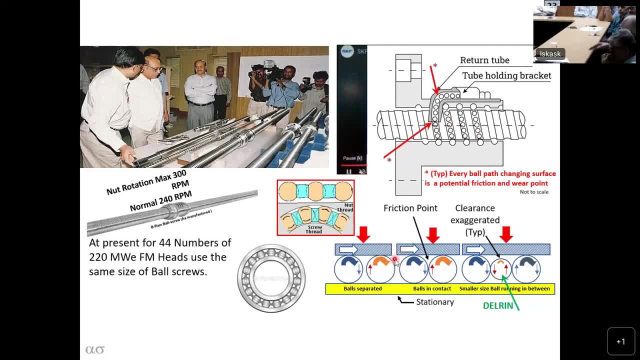 problem, even for icl. then they had changed the design when they went in for pickering and other things. douglas point at some point of them stopped, then went in for pickering. they changed the design but we were not able to do that. so this is the return tube that is there now. you anybody knows. 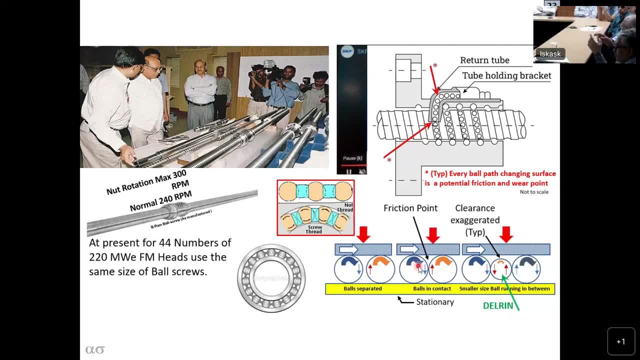 one of the points was ball bearing. a ball screw manufacturer says don't rotate the nut because when they're rotating the nut at high speed it has got centrifugal forces, it pushes the ball outside and it spoils the issue totally. so our design has the ball nut rotating at 300 rpm. 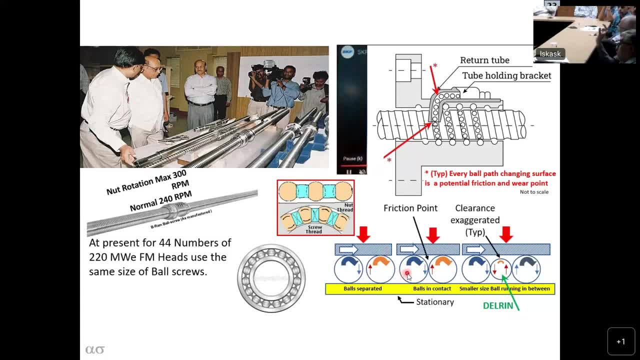 the icl have changed it to have walnut traveling screw rotating. that they have done, which we have not done so far, and they have also installed. see, two load bearing balls are there. you put a non-load bearing ball building so the ball will not jam against one another to cause friction. so these are the things that they have done and 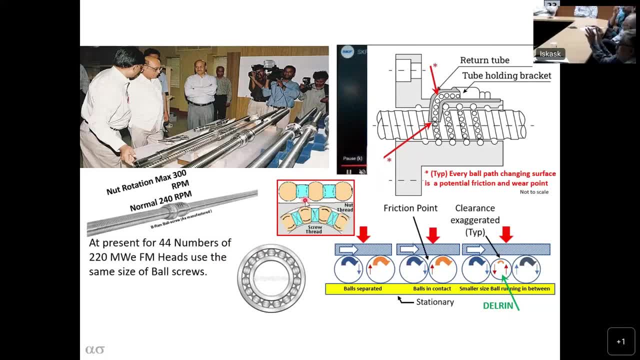 germany they have even found out spacer between two balls. they have done it, we will be doing. ultimately, these ball screws. we have to make it work come what may. we have to make it work because there are already 44 fueling machines using this ball screw: 220 megawatt and then 500, 700 megawatt. 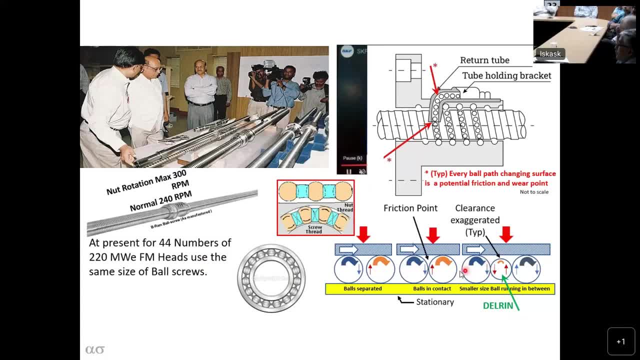 are also having ball screws so we got to make it work. so work, development work on these ball screws will happen. uh, one of my colleagues late, mr mathur, has actually improved earlier. this ball screw used to come only every 200 channels. they used to change. now it has become 700 channels so that 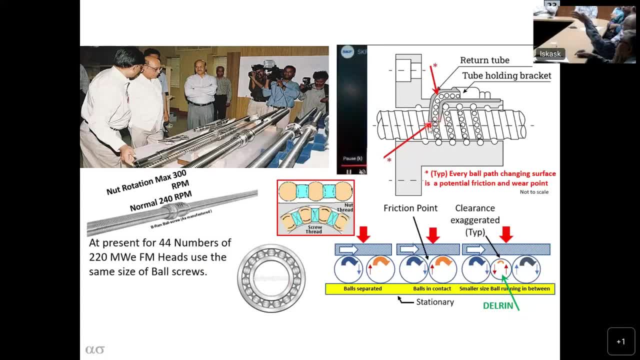 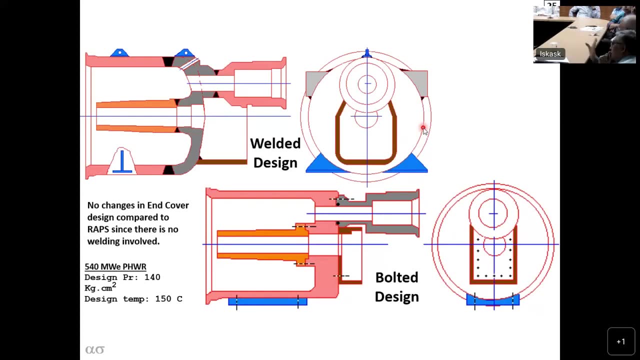 is because he has made some changes in the pickup tube in such a way that doesn't cause so much friction, so it has life increases like. so it is now 700, not too bad, now this. you will miss this now. this is the i would consider in this seminar if i were to say this is the most. 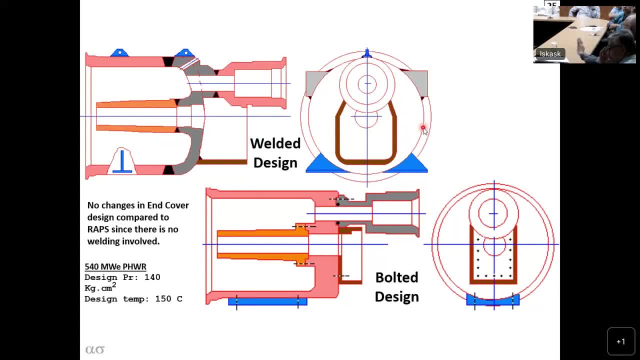 important innovation that we have done. this is my theory here. the real reason is the top one. you see the magazine housing. it is a welded uh thing given by asia. even canada did not have this equipment for the manufacture of this. they went to a company called taylor force in houston, texas. they 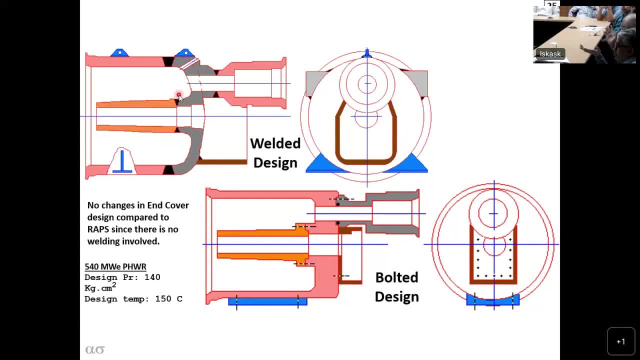 made before, why it is 403 material, which is p6, 403 material. they made this, uh, one, two, three, four, five separate forgings and they welded it. now if you have p6 material welded is about 30 millimeters wall thickness. there are two pressure weldings. this is this is one pressure welding and this is the. 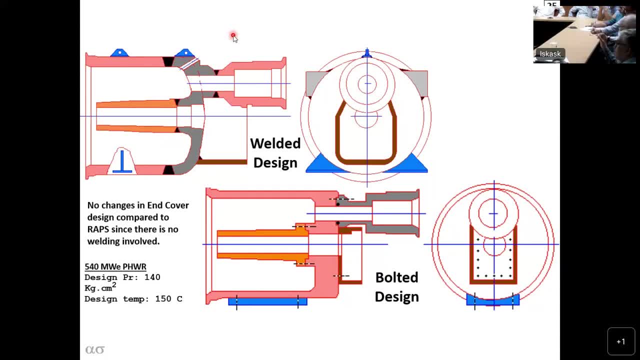 other pressure welding, welding capable of standing internal pressure, the others are mechanical strength is required. so this 403 uh thing you have to finish weld off all of this and then you have to do post heat treatment. that means the entire housing, entire vessel has to be put in a furnace and then it has to be taken to 1800 degree fahrenheit or something. 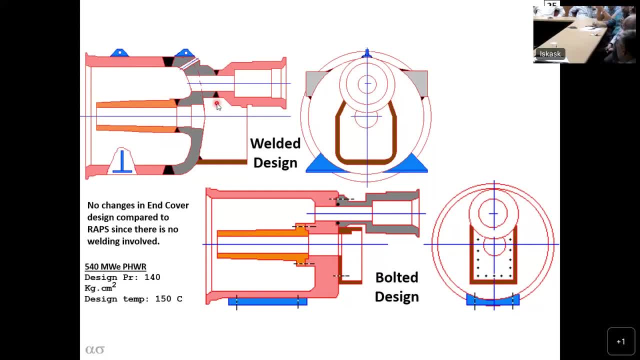 and quenched in oil, then heat treated. so that means a coil bar. just no way we could get this in india. just no way, absolutely no way. i don't think even now we can get it. this one, it's a welded design. so, uh, for madras also, we had a problem, but we were able to import it from europe. 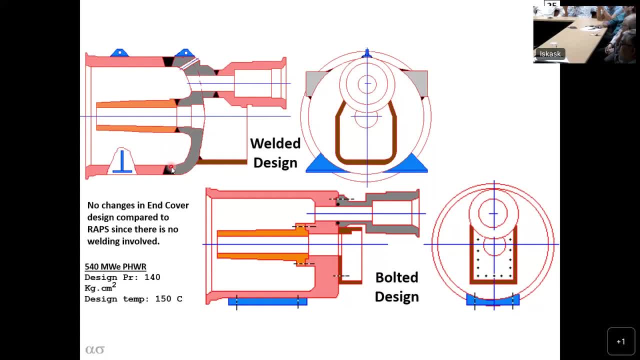 obliged to redesign. then my metallurgy guru, mr balramurthy, suggested sanat: why don't you change this? welding this? avoid this. welding. you make a flat head. you make a flat head, then it is possible to forge it. the person will forge it semi-diforce and then punch it on the center, so you will get. 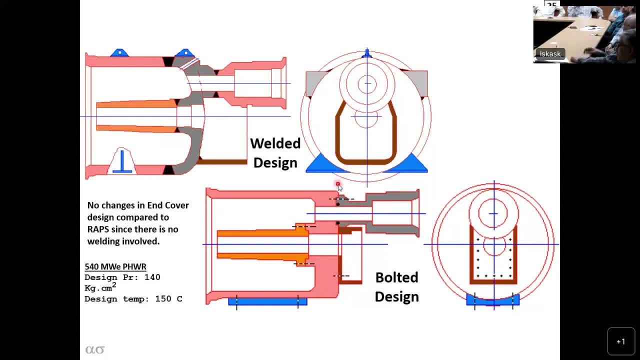 the grain flow also correctly, you will forge it now. the problem was this kind of forging. at that time in aurora time it was not available in india. it requires a six, some six thousand ton brush, which is now available for 700 watts, but it was not available for us. so we got the forging now. 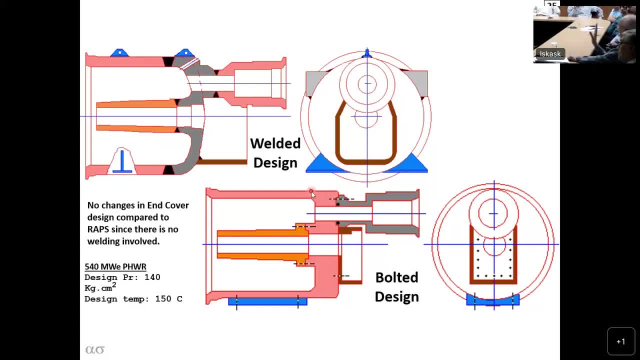 point about this is that if you remove the welding, the forging is, anybody can do anybody with the equipment. it is the welding that is a problem and the machining. so we were able to get the forging and this is what, ultimately, we designed it. so all this, all the this, this, this is a 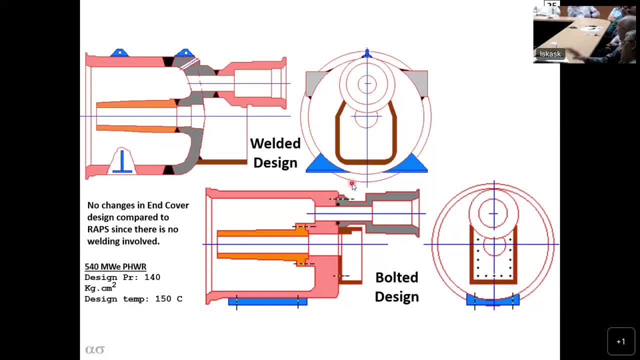 see this weld is avoided. this joint, pressure joint, is done with bolt, bolted, assembly with a metallic seal, finished. everything else is only bolted there. we don't go with a 10 foot long pole with a welding rod near this it. everything is done. all the parts are heated at first, finished machine and assembled. that is the way it goes. 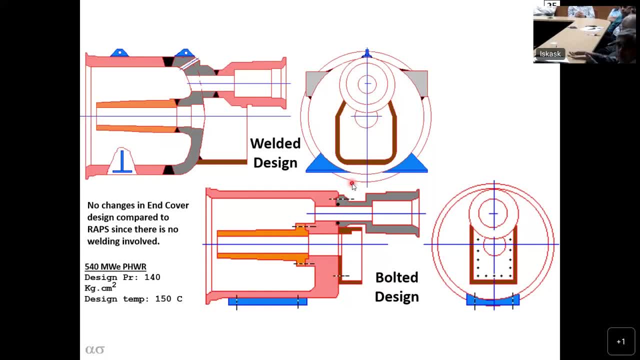 so now this has been uh done very successfully from aurora narora one onwards to 500 megawatts to 700 megawatts. this is the design that is going, only thing is with slight changes. without this narrow one would not have come, we would not have been able to get a mass fueling machine. 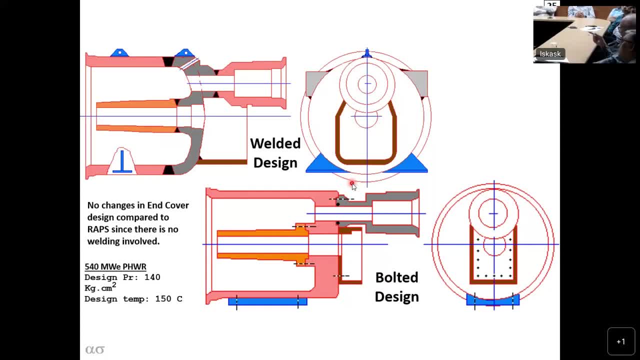 in there. anyway, that is what is, and, uh, this, uh, what are these materials? 403 stainless steel, both, yeah, all the same material, same material: 403 stainless steel. and dr singh was talking about pressure testing. this is the machine that we pressure tested in central workshop. he did that, so we wanted to put strain gauges in the water. we, in order to 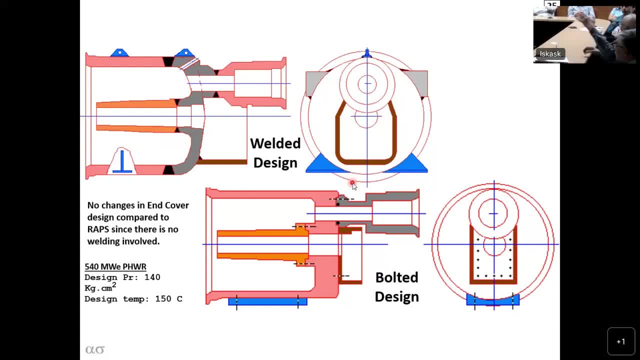 pressure test you have to put. the mating component is coming here, so they have to put everything together. and the strain gauges somebody wanted on the inner surface, because 30 millimeter thick. you need to know what is radial stress, so 10 gauges have to be put and then he has touched. 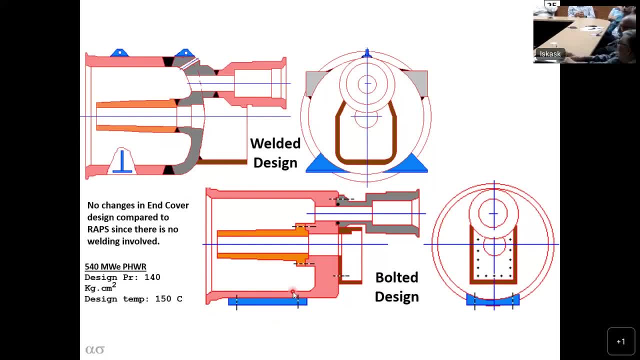 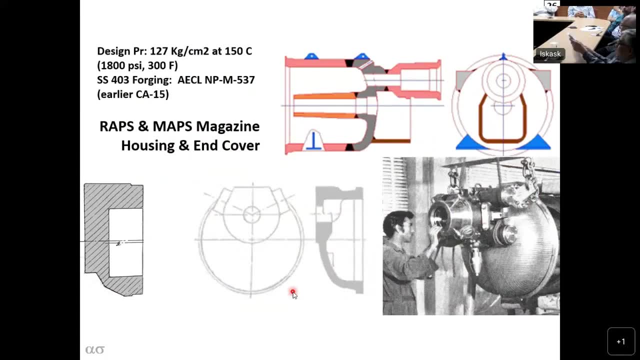 the nose this way and got the strain gauges for working. you know, very, very interesting job in central workshop. that was done. once the pressure test was done, then it means of course it is meeting all of that, not only present. ultimately they did kushwaha and dr singh did the stress. 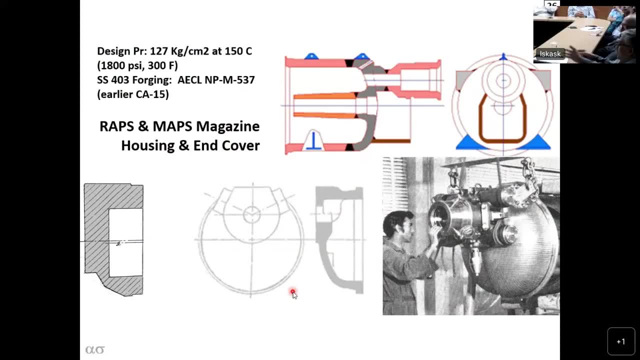 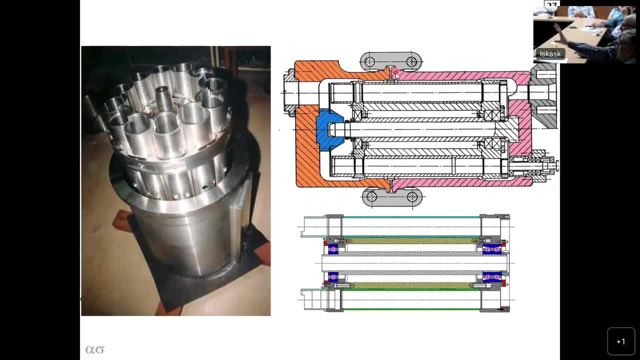 analysis, finite element analysis. it became all right. this we will miss. now you can see here the same housing, same design for 500 megawatts, slightly bigger dimension, but the same same thing. but what is important is that these two parts are joined by a class which is called the graylock class. it is come made by a company called. 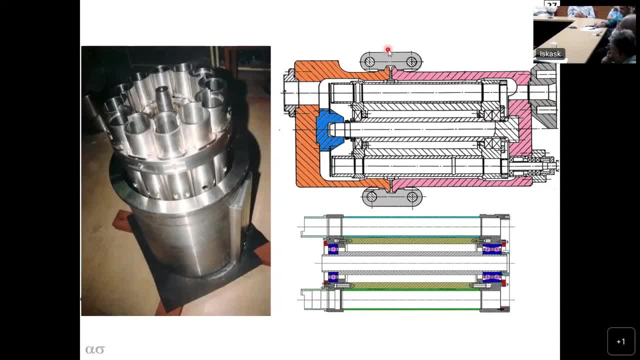 the gray tool company in houston, texas. they were having it and at some point of time they said we will not give you this. so this needed to be indigenized. there are three such clamps needed to be indigenized, so this has been indigenized by 500. 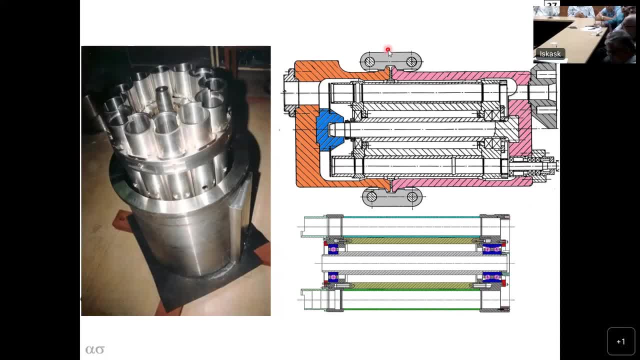 700 megawatt people now- uh, terrific indigenization. the thing here is 220 megawatts has got that 13 inch clamp. we have made sure that the 500 megawatt magazine housing meets the same graylock plan. we don't have to buy another graylock. so this is, this is the thing we did. and then the magazine. 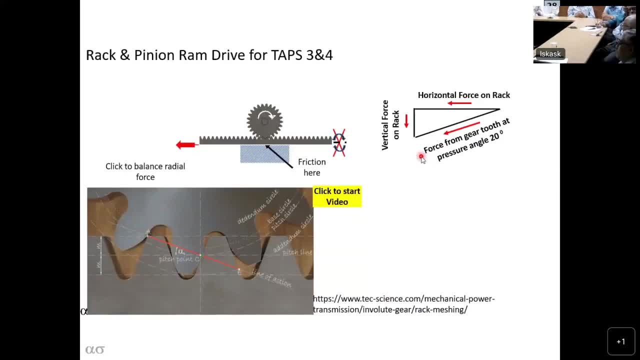 now we come back to this: uh, 500 megawatts for lower money. we could not get ball screws for the ramp. so what to do? and then, when we were testing the ram, the ball screw ram was getting stuck up, stuck up, suck up. we have tested up to 12 o'clock in the night, etc. etc. hall 7, hall 3, nothing doing. so he again, here is a do or. 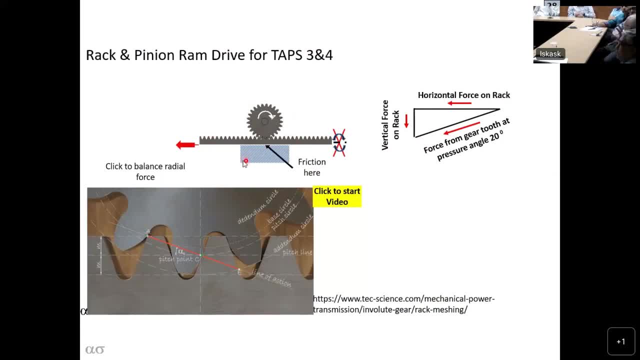 die situation. so we thought: after all, a rotary motion has to be made linear motion somewhere. you've got a motor, hydraulic motor, re. it needed to be made linear motion somewhere. how do you do that? there are several ways. we cannot use hydraulic cylinder because you cannot position it. you need a mechanical drive. 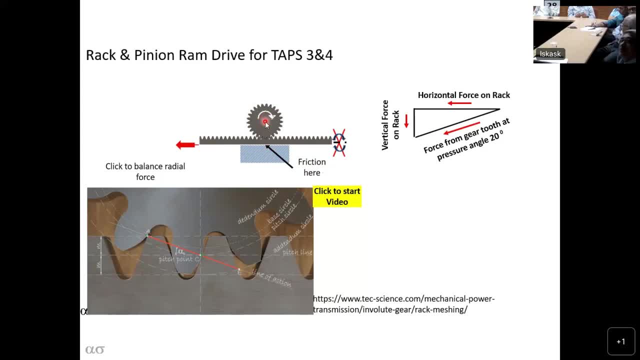 to do this. so if you have a ball screw, ball screw is not there, you use a rack and pinion rack companion. if you use first, objection is that it is friction. too much friction is there, which we solved saying that if you have invalid tooth working on a rack, it 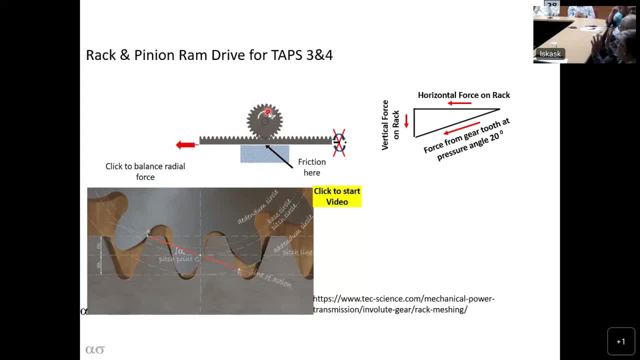 is pure rolling, at least theoretically it is pure rolling, it will roll. so there is no friction. it is because of the rack and pinion that is coming, so we put in value to. then there is still an amount of friction because if the at 20 degree pressure angle, when 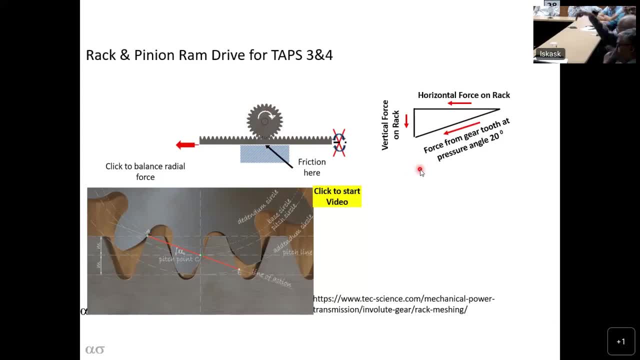 you put 20 degree pressure angle, it gives you the horizontal force which we need, but it also gives a vertical reaction. that vertical reaction will give a friction with the support of the rack. so how to do this? we said, okay, we will put another. see very often rolling mills. you have to roll mills and 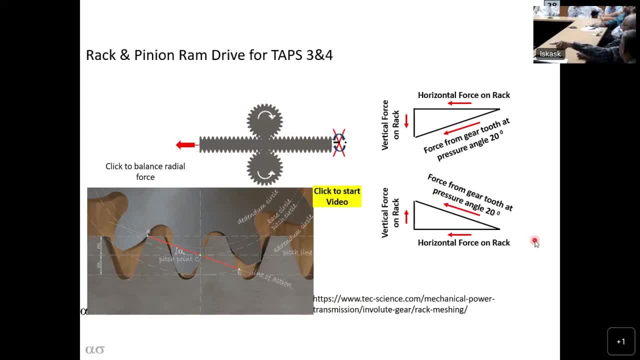 then it goes. so we put it on that, so the vertical reaction is cancelled out. the advantage with this is that if you put the two rack and provide the same, then the rack, the pinion, the motor torque, everything can be halved, really speaking, but we made it 60% just in order to that. even one is not there, it will still work. 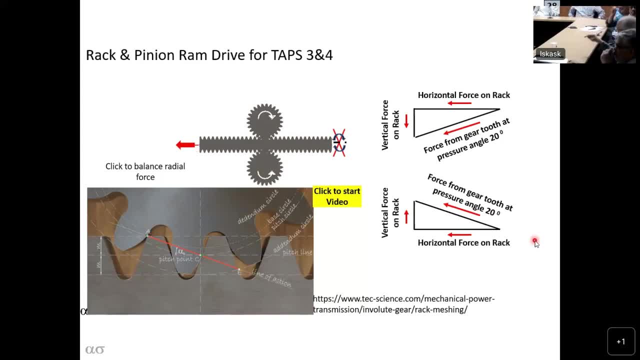 so the gear teeth is smaller, the shaft is smaller, the ball bearing is smaller, but the problem is that still the RAM became bigger because we wanted to put this another coaxial RAM is there? no, that, we wanted to put that also rack and pinion. so that is why the RAM became that rack support become a bit bigger. so this is. 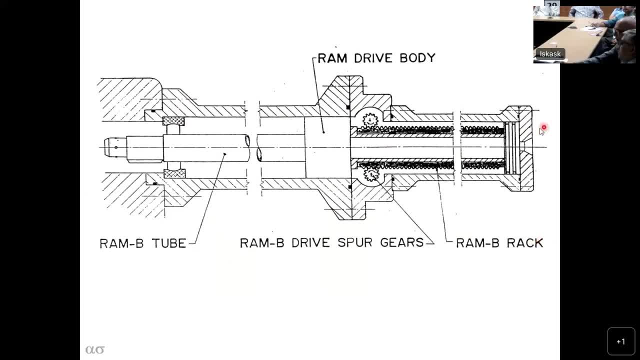 the how it is implemented. you see here, this is the. this is a rack support. this is the pinion that is driving. it is driving the thing here. now this is- you can call it- a traveling gear box. this gear box has got gears so that, whatever the RAM is, that gear box can make some gears run, so that the 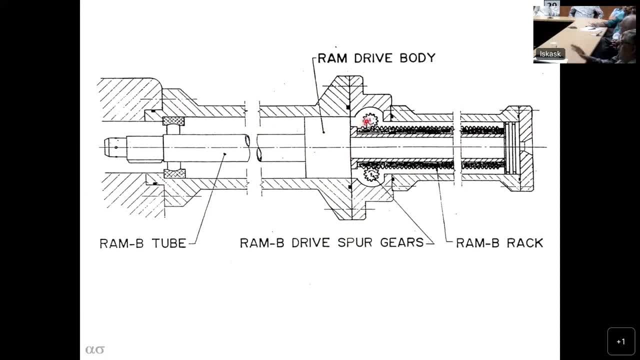 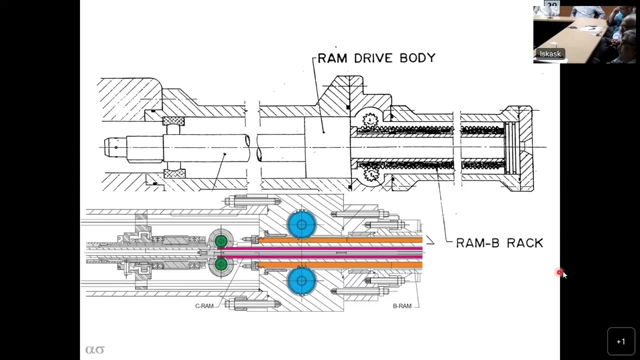 inner rack can work on this. so, ultimately, this is the you know, very easy to tell, that is what I want. but ultimately, by the time you prepare, by the time you come, this is how it is implemented. all very complicated thing. so this is how this is cross section. this is the cross section, this is. 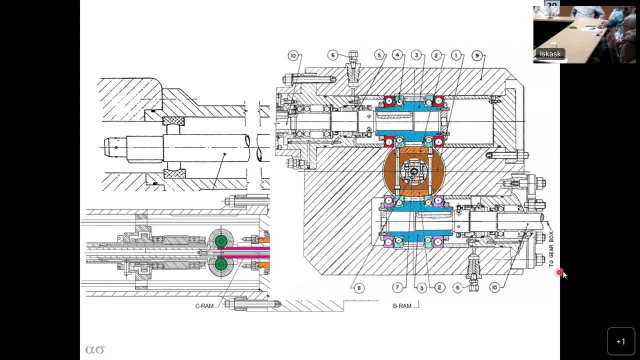 elevation. this rack and the rack support it to time. but one thing is very important is this: which is not there, to my knowledge, in any of the acl machines is that this ball bearing assembly is modular. you can simply take it, put it and then test it somewhere. 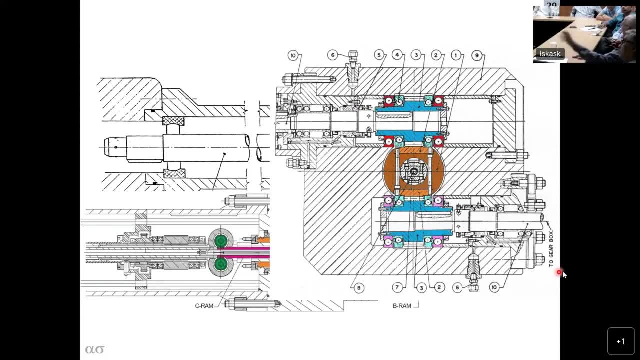 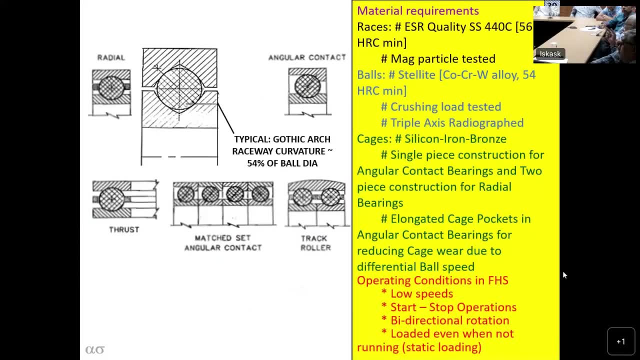 else and put it back. the whole thing is modular. all ball bearing assemblies, all seal assemblies are modular. they can be removed. okay, so now we come to ball bearings. ball bearings: everybody knows ball bearing, but everybody knows only oil lubricated ball bearing. water lubricated ball bearing is a problem because oil lubricated ball bearings use carbon steel. they use carbon steel. 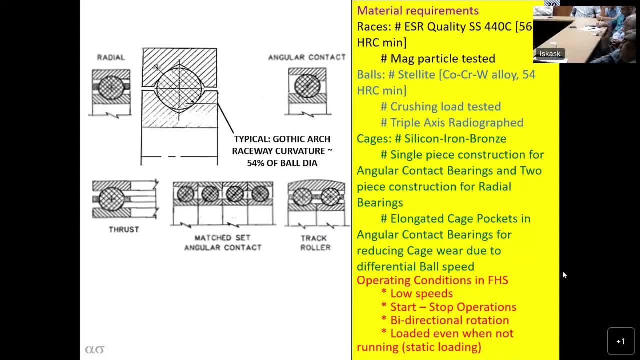 balls. we cannot use that in here because of corrosion, and stainless steel does not have inadequate hardness, so the ball bearings have to be terribly derated in order to be working. so this is what we found, that in all three they did a test. we said: if you want, 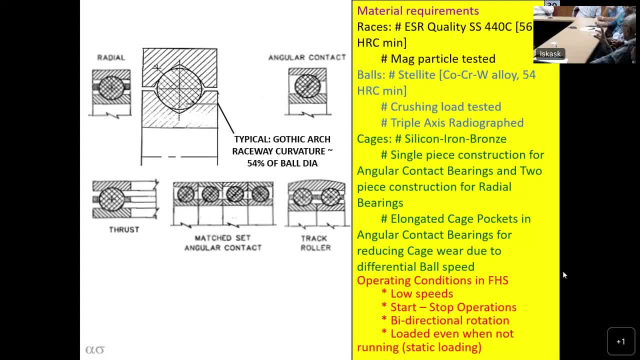 your load p to be taken by a ball bearing, then you must select an oil lubricated ball bearing which is eight times speed capable, so it has to be taken eight times. so that is what it. but we have different types of uh ball bearings. not all these are used in 220, but 500 megawatt uses this. 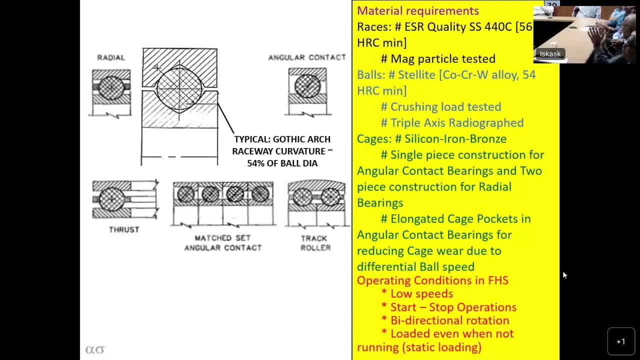 and the in a water lubricated bearing the raceway does not have full compliance. normally in oil lubricated bearing the raceway is 50 percent of the radius of the ball. here it is 54 because where particles are there and they have to go through the bottom. so that is the reason why. 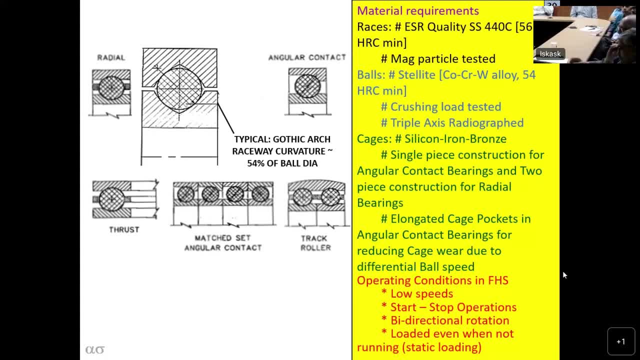 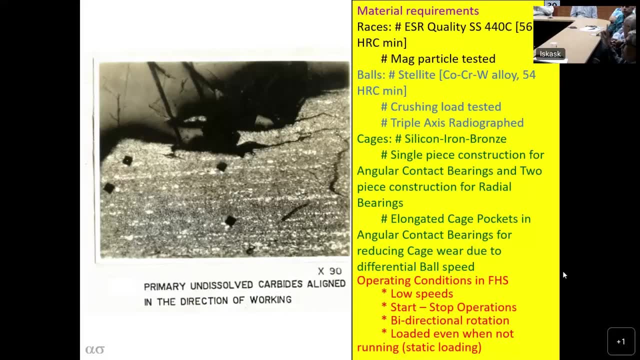 ultimately, we got this. then we tested when we tested- see, we got all this here. we tested when we tested this, what happened at least with one bearing? we tested the bearing with the highest load rating and you can see that it is failing. the raceway is failing, not the ball, the raceway. 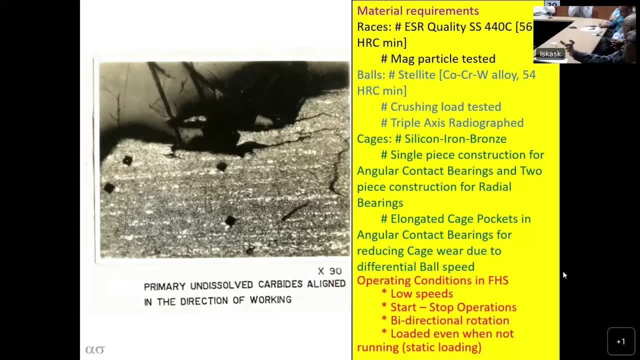 is failing. why is it failing? that is because the 440 is the 440c material. 440c material was neither superfluous as it was because the 440c material was not very good. it was made very easy to replace ESR quality, nor CVIR, It is normal quality. So the carbides had precipitated along the 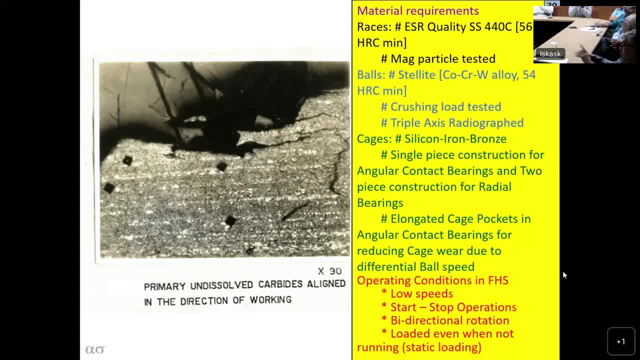 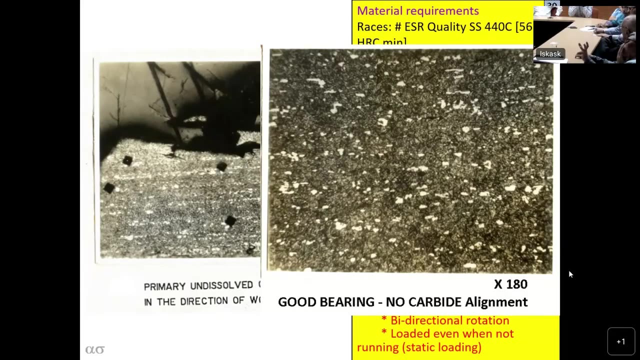 line here and they were weak spots. So we said no, no, no, no, not possible. So we are now dating either ESR quality or CVIR quality, so that any precipitates there are finely divided. So that is what we are now having here. So now, with this we have, I think we 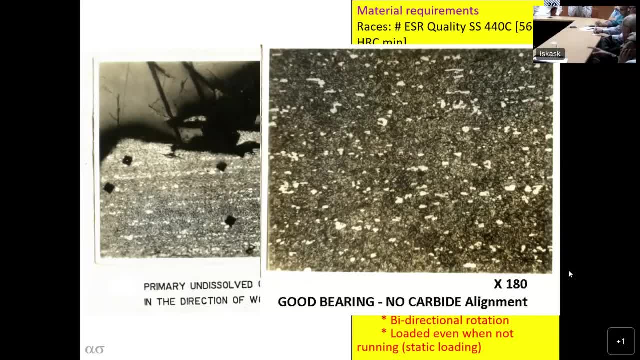 have solved Now, at least as far as 500 megawatts is concerned. this water lubricated wiring was also not indigenous. Now these people have indigenized that also. They are making it in India. This is a terrific job they have done So now these are the last. 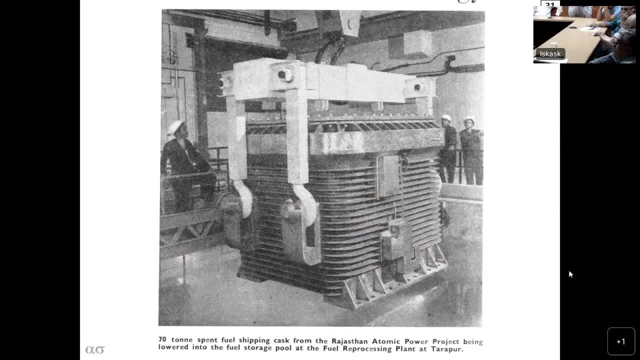 two slides. After all, after you take the bundles into the bay, our job is to send it to the plutonium plant. We have to ultimately give it for reprocessing. That is our policy. So a flask was designed. This is 1974.. In those days, 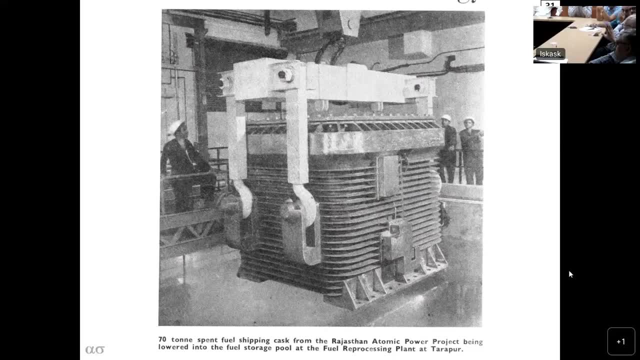 the bundle was kept in the bay, It had a cooling of only 180.. It is producing a lot of heat, So even though it is out of the reactor, it is producing heat, So it needed to be cooled. So we needed a designed flask which will have fins and it will cool 180 days. Then 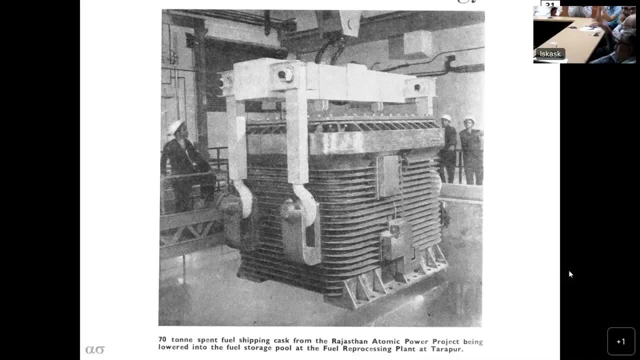 later on we found decontamination of this problem because it goes into the pool, The flask. the only important thing is this flask has to be compatible with the pool in the reactor as well as the pool in the reactor. In fact, Mr A N Prasad and Sita Ramaiah, they have the one who ultimately approved. 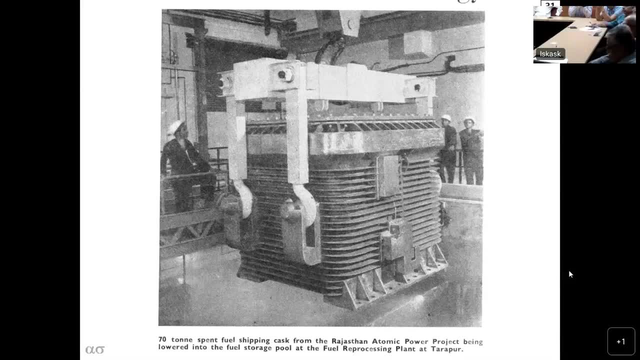 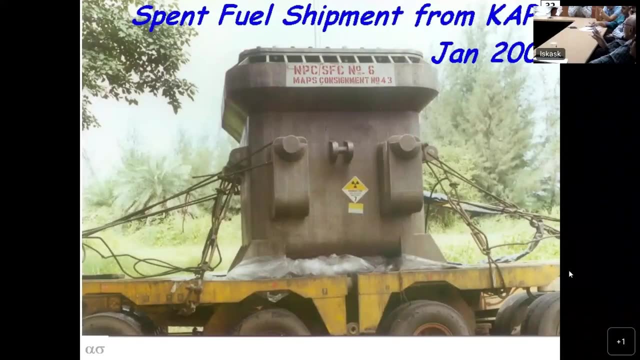 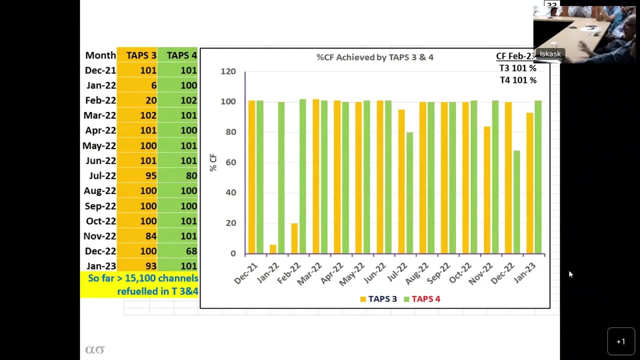 this design okay to work in their pool. So that is what it is. Then later on we redesigned it to have a smooth surface so that decontamination will be possible. Now comes the last slide, See Tarapur 3 and 4, in the last 15 months. any operator should be very proud of this. 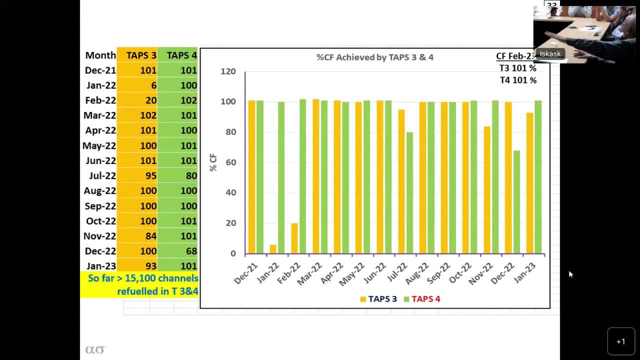 output. In the last 15 months it has been consistently holding 100% capacity factor. Now I am not saying that this capacity factor of 100% all the while it is here, December 21 to January 23,. at the time I prepared the slide, the February data was not available. Now it is. 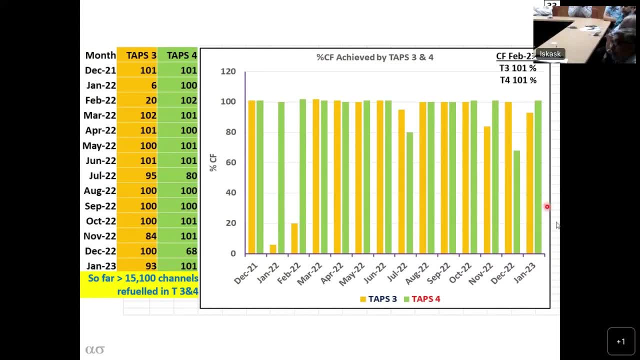 available there. I have put it down, So I am not saying here that this is only because of on-pour refilling. On-pour refilling is one, but several other things also have to be. Tarapur 3 and 4, at the moment, heaven forbid- is working very nicely As a matter. 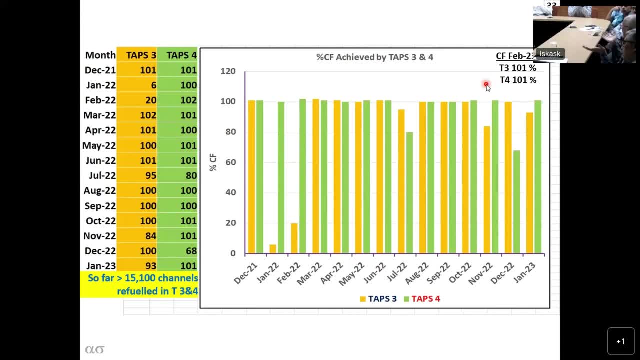 of fact, I would like to even suggest that, if late Mr Kati was here, he should be very happy with this performance, because he was the chief designer for 500 megawatts. Everything was his, Everything was his. So that is what he did. Now I am not sure I will leave this. 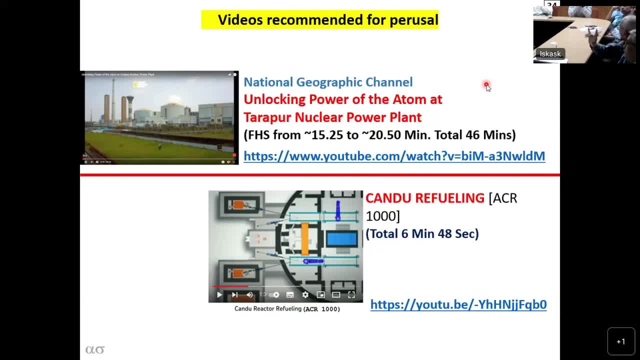 on for some time. This is the end. I have come to the end. I will leave this slide on. I would very strongly recommend. Okay, So I would like to say that you please see these two videos to the links that I have. 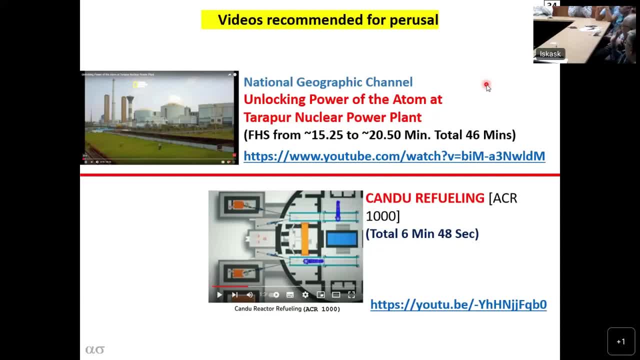 given. If it is not there, I will give it to Dr Singh. you can take it from him later or you can take your mobile camera and capture it. So these two. the first top video is provided is done by National Geographic and it is about Tarapur, And I have said here. 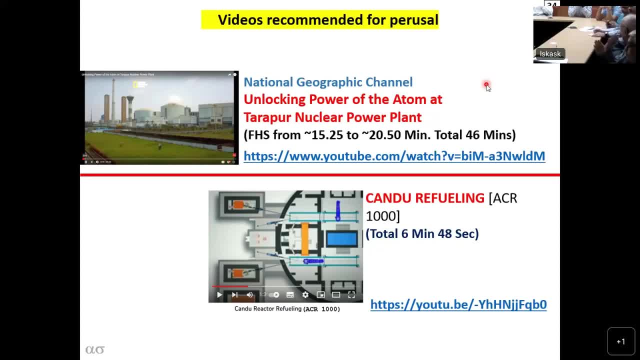 from about 15 minutes to 20 minutes. it talks about fuel and if you talk about the entire reactor, but 15 minutes to 20 minutes, 21 minutes, it talks about the fuel handling. Okay, exclusively by a very, very dear friend of mine, mr uh. um, actually he is the man who got this. 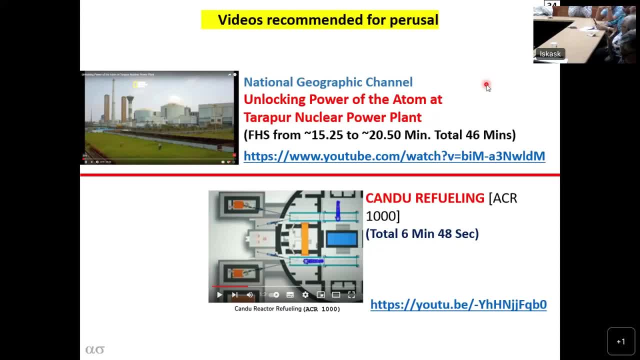 commissioned in tarapu. three and four these machines. he owned the machine. this is very important. the operator has to own your design. if it doesn't do that, it won't work. so this is what he won't do, that, and that is how it got. and then the next one is also by acl. 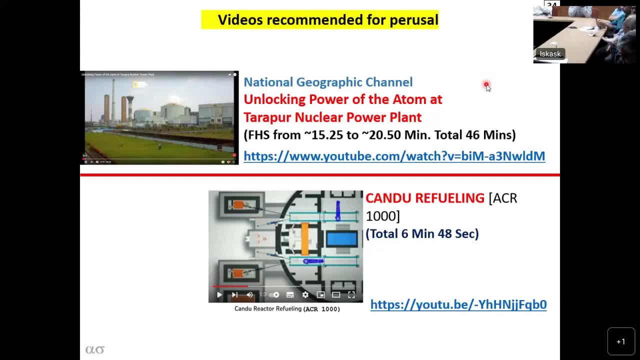 they are. uh, they had a acr prop, a proposal for making a thousand megawatt phwr. i think they were cheating a little bit. they were trying to put some industry into this, not to get so. anyway, this is the one. but this is a fuel handling system. 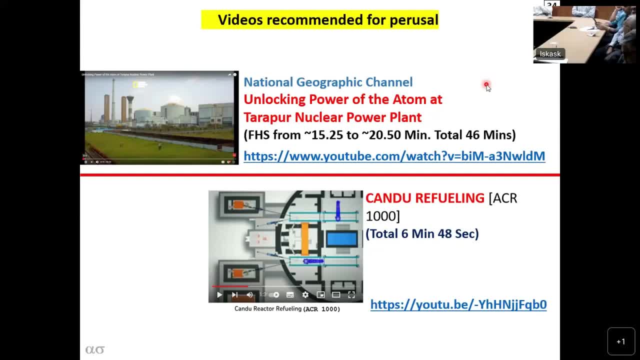 of that acr they have put. this entire video is on that purpose, so you can see it. our 700 megawatts does not actually completely follow this, but it has got some principle of that implemented in there. okay, so i come to the end of that. i don't know whether i'm on time. 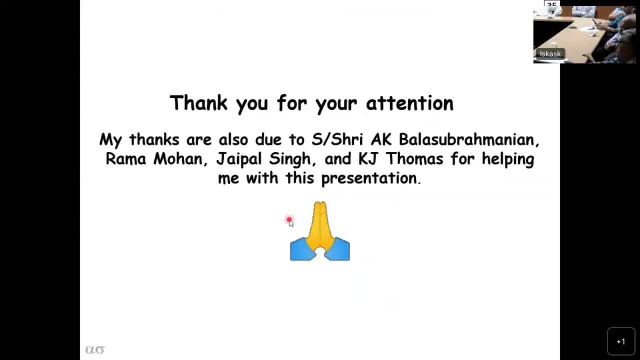 thank you. thank you very much for the patience. say, one more is there. that is important. so thank you very much for your patience. i hope you will not ask any questions anyway. uh, yes, sir, thank you. so thank you for your illustrious lecture, and it was just, like you know, carrying forward with your journey, and i 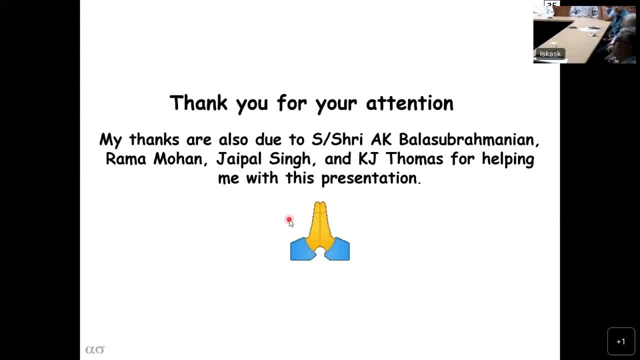 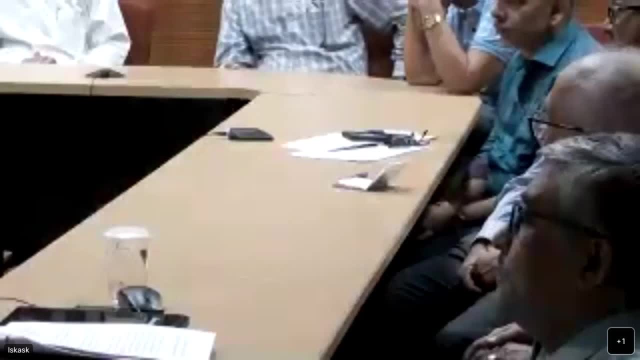 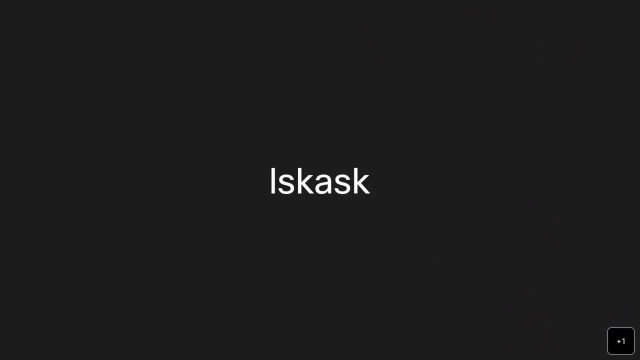 think it was just like a refresher course for all of us in mechanical, electrical, electronics and control engineering and on top of it, the nuclear engineering. so i thank you for your lecture and i am sure many people will have questions, so few questions may be addressed by you. 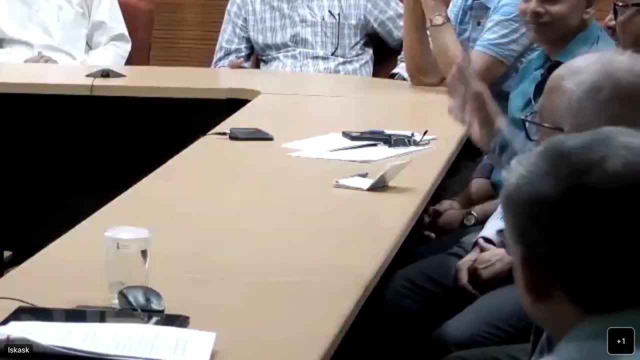 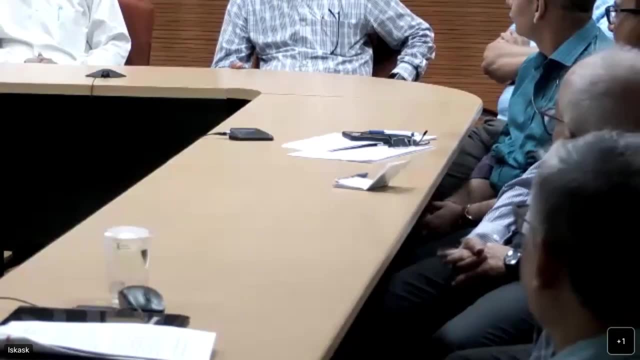 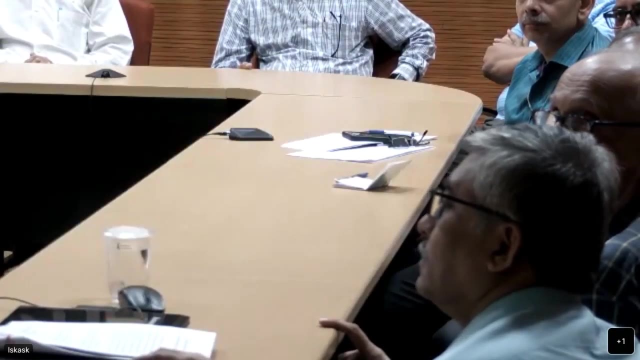 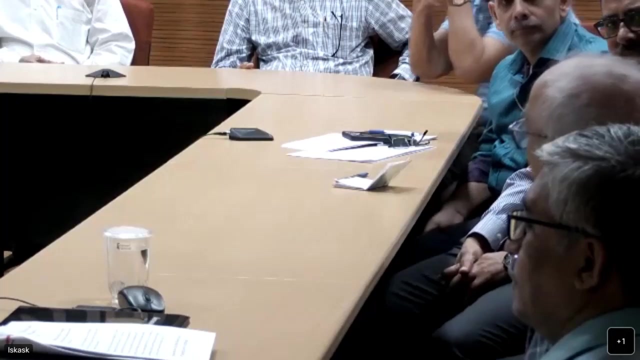 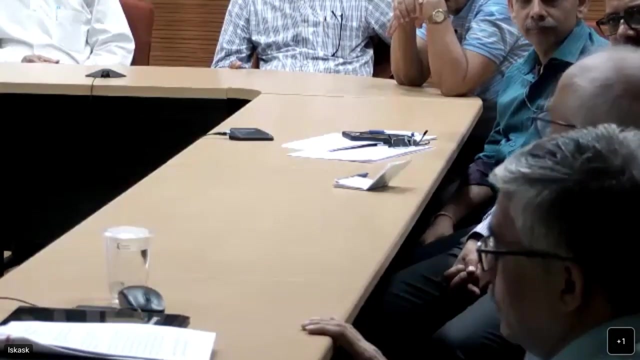 from here. so let's see chat box. if there are any questions, yeah, chat at the right hand bottom. no, not as yet. see the fuel handling. i will tell you. uh, apart from that, we used to have a very illustrious senior senior to me one, mr jayabarga. he was trained in canada and he used to work in 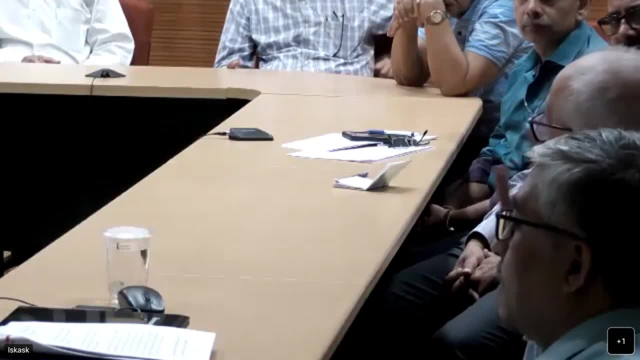 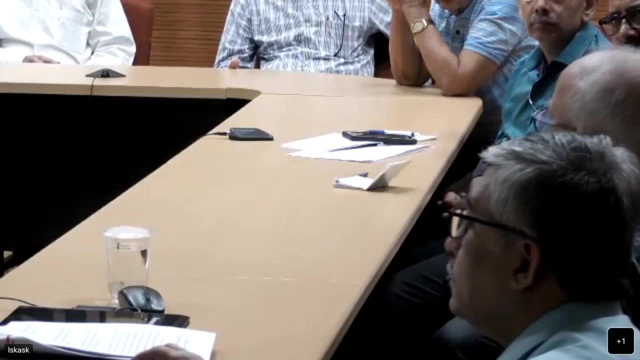 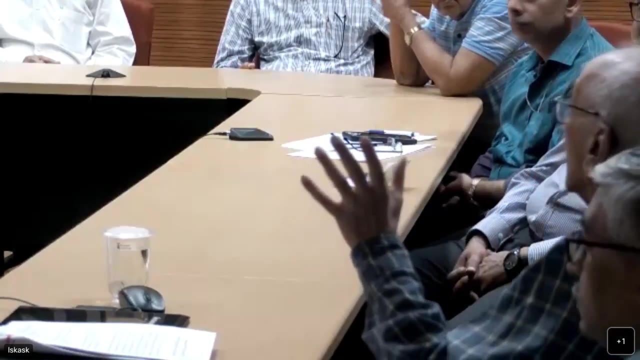 rap one and he was in charge of the fuel handling system in rap 1 and rap 2.. he was getting frustrated because you know, when you commission a system, nothing works. you have to be. then he was saying: normally what happens is the project manager is saying: when are you going? 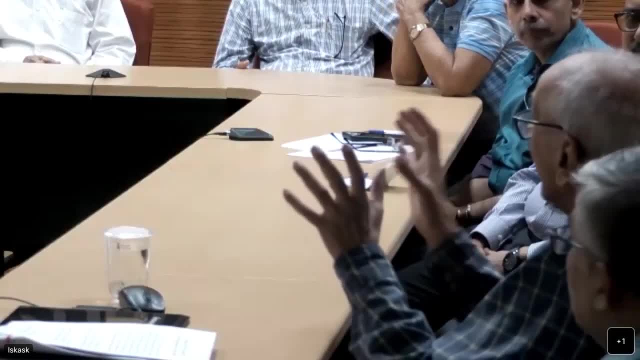 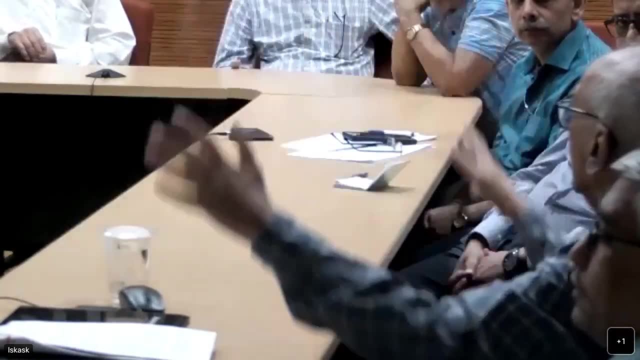 critical. when are you going critical? when you do that, he says there's always a pressure for you. so he got frustrated and then said this fueling machine is a black box. it's a black box that the terminology brought in- black box terminology for the fueling army. 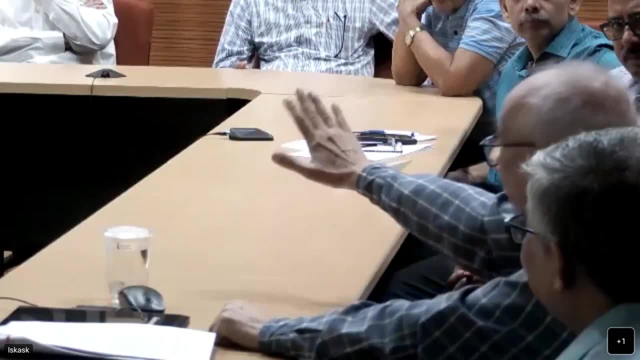 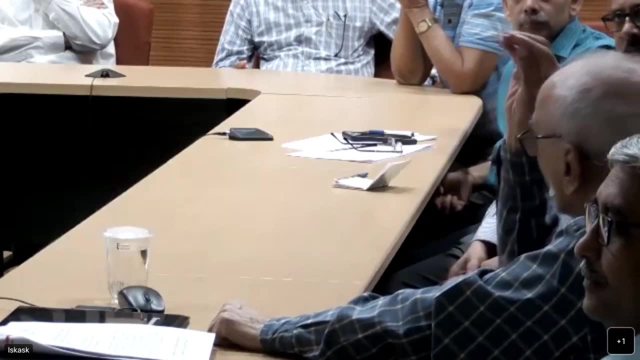 since then, everybody has treated this fueling machine as a black i. i don't want to know about fueling machine, so this is a black box. so i used to tell that it is not a black box. you come to me, sit with me for half a day. i will simply explain to you everything. but that was not the case. 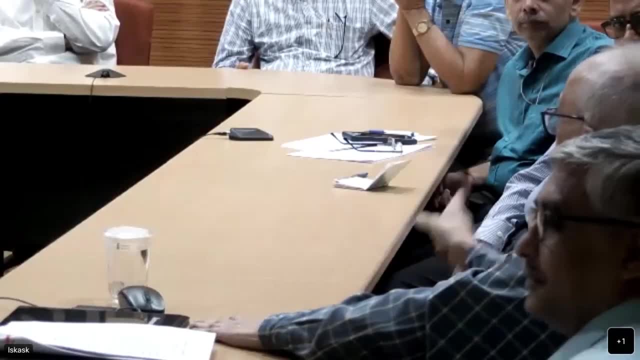 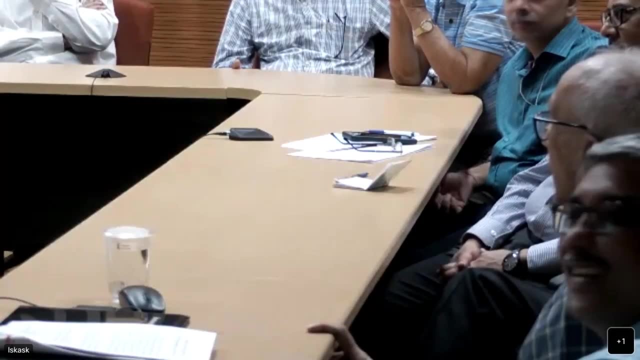 because it was easier for everybody to say that it's a black box and forget about it. so. so maybe that is, the black box theory is working here. so how did you take care of alignment of fuel machine to the channel? yes, yes, yes, very important, very good, good question, uh, if you see. 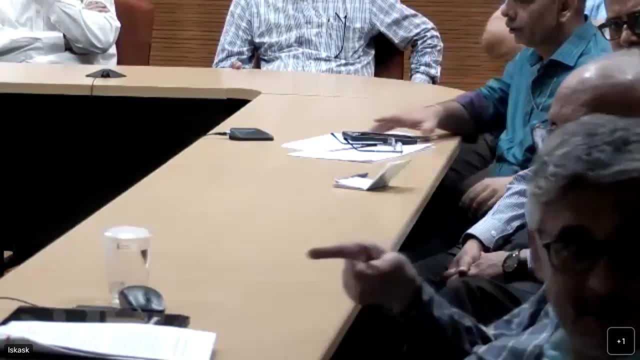 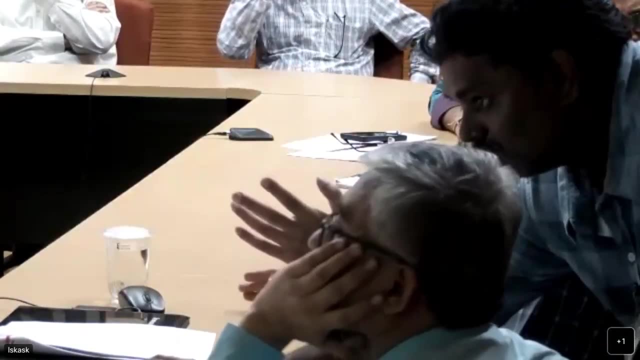 here. can you go back to the? can you go back to the? it's okay, no, no, no, i'll tell you the fueling machine. i know, i'll show you the slide. oh, you know, it's okay. it's okay now i'll go, i'll go. 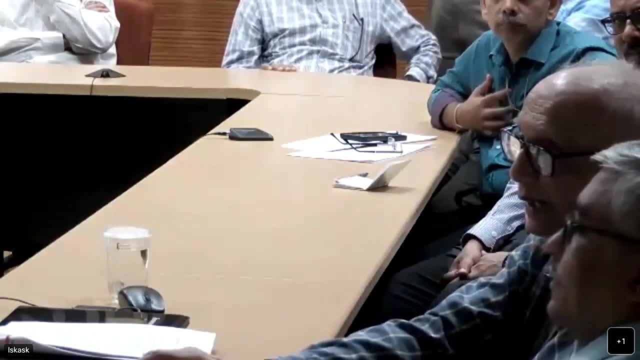 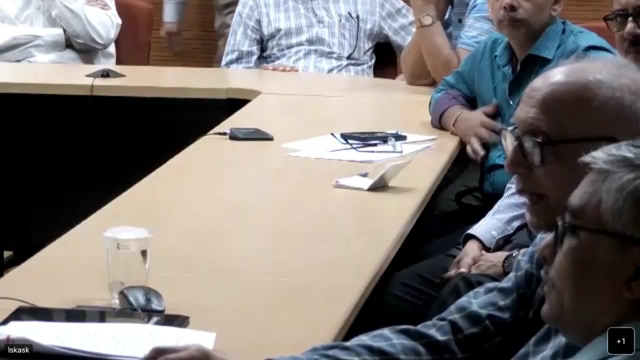 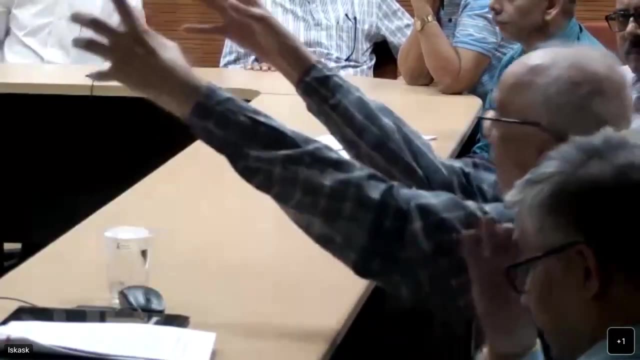 see here, you asked a question here correctly that. so i have just put the xyz, that is the machine, has to be one channel, you have done. you have to move it to the other channel. you have to move to the channel up and down, you have to. it is very. 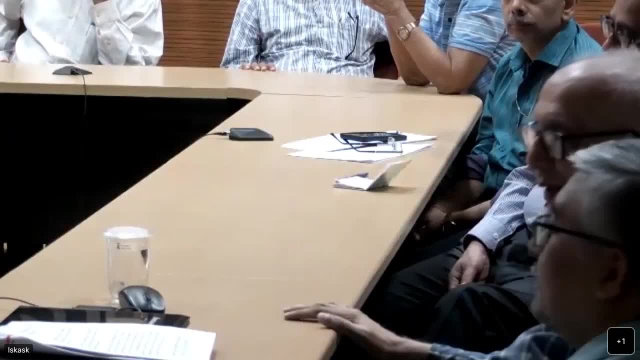 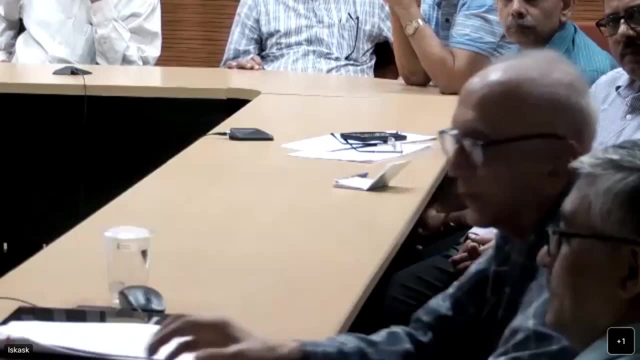 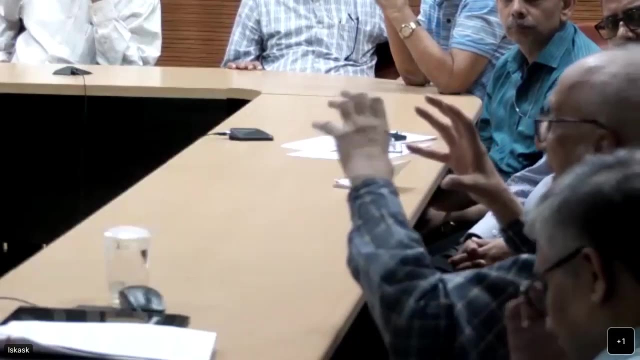 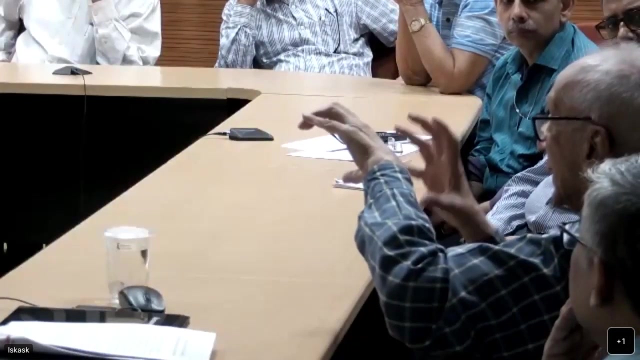 easy to put xyz but quite difficult to come and do it. and that is exactly what is being done by this in the case of aecl. this is called the carriage. the machine is kept on it with gimbals, with gimbals. so the uh, exactly like uh, refueling in the media, refueling the fueling machine comes. 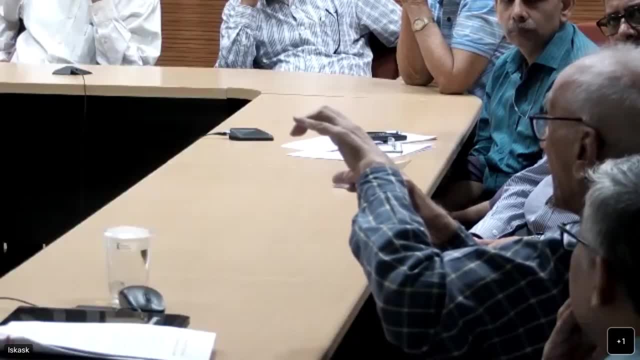 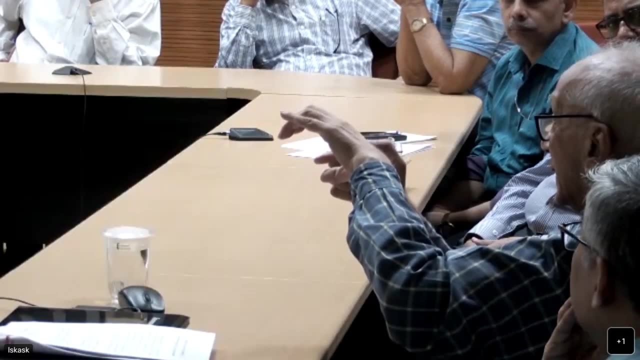 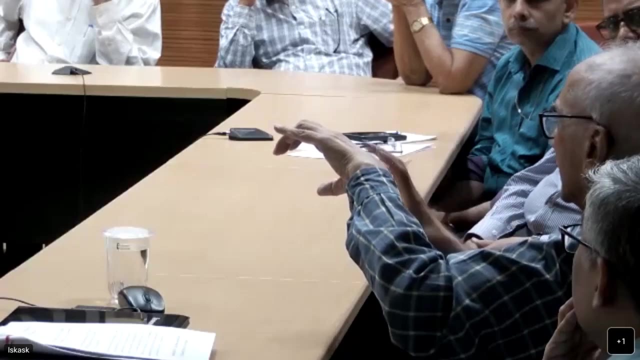 and you know the position of the channel within a tolerance of 10 millimeters- actually much, much more, much better, 10 millimeter. you know where the center line of the channel is, so you position the fueling machine y and z with the potentiometer lvd. it is potentiometer, fine drive you have. and then you come. the error band allowed is 10 millimeters, but actually much, much better than so. then the channel end fitting and the machine have got papers. so when you advance in the z direction the machine tilts. you sense that tilt and then try to correct it because it will tilt in y. 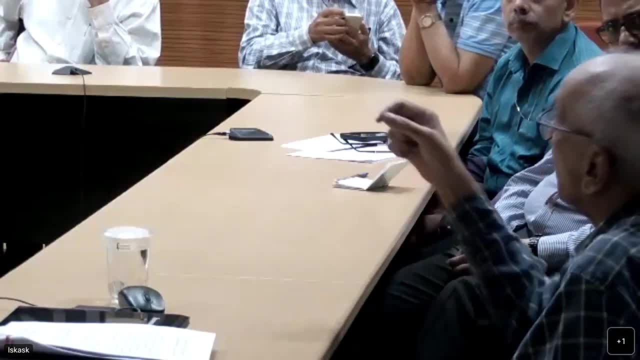 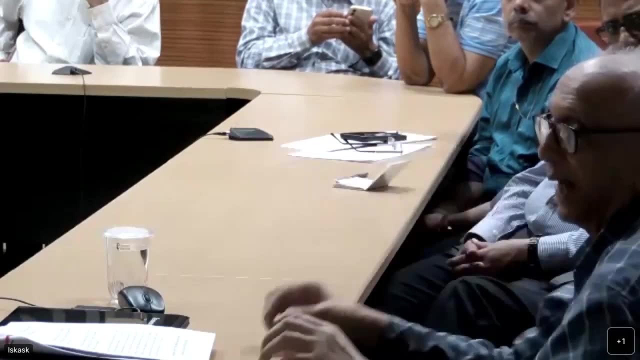 direction, or it will tilt in x direction. so you make a correction by finding the z direction, and so you make a correction by fine y and fine x. ultimately, the point is you need to get the machine in line with the channel. as a matter of fact, if you see here, my drawing has not been very. 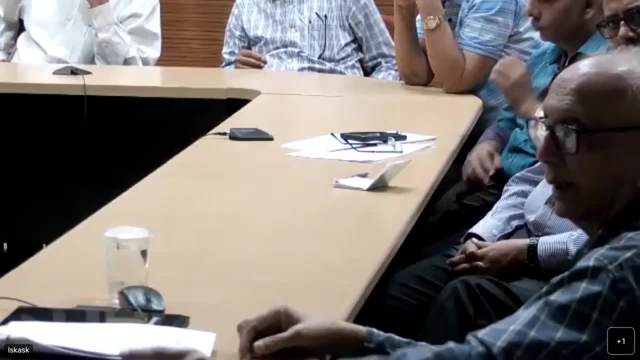 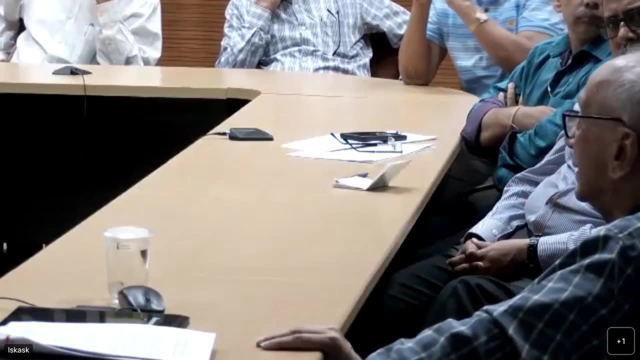 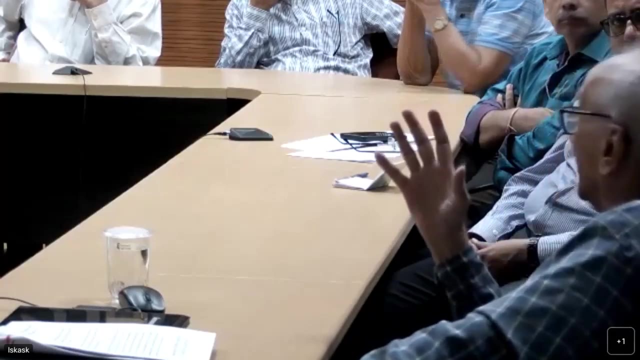 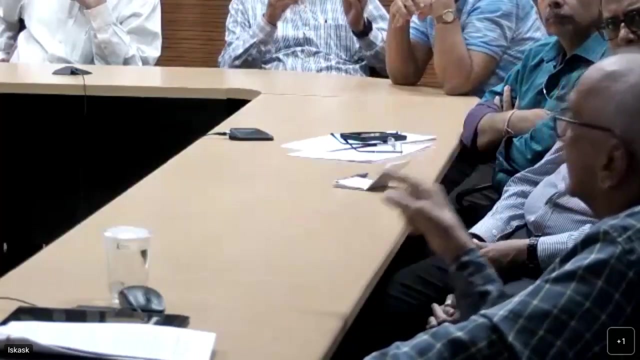 good if you see carefully. see, this machine is not very well aligned with the channel there. it is sorry for that, but i didn't have autocad or anything else, so, uh, drawn only with powerpoint. so it is required. so this is done. there is a error correction system available. gimbal driven error system system is available. 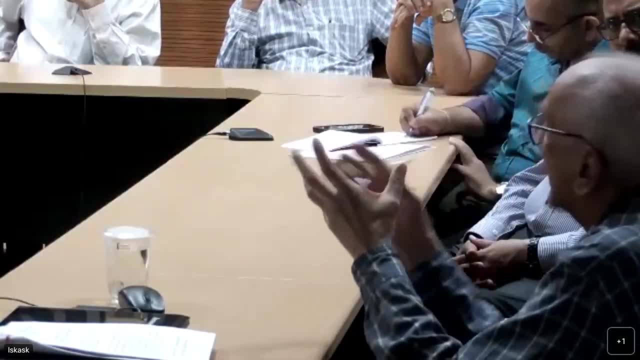 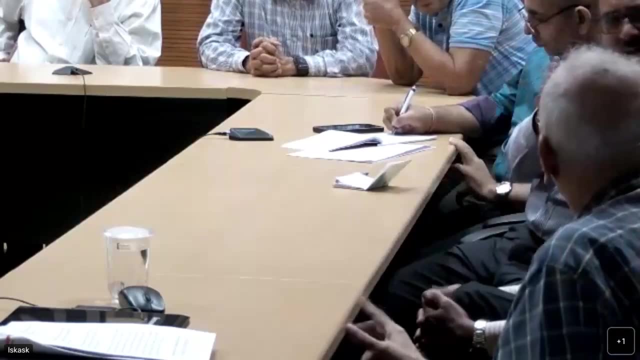 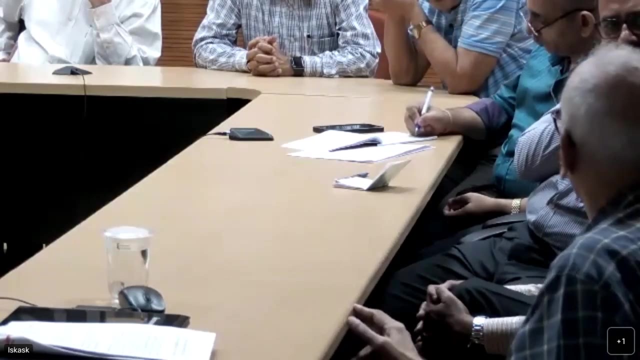 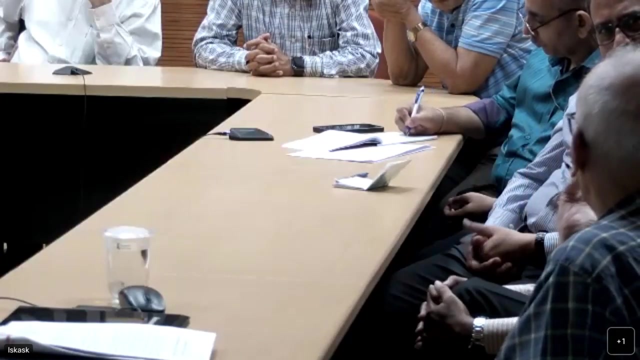 for the machine to align, and once it aligns it clamps, then ceiling plugs, shielding all that. oh sorry, i don't know too much about pfr, but they tell me that pfbr refueling has to. once they have a, they have got sodium first of all, and 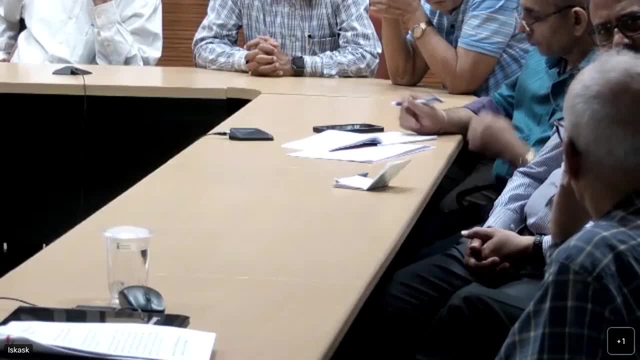 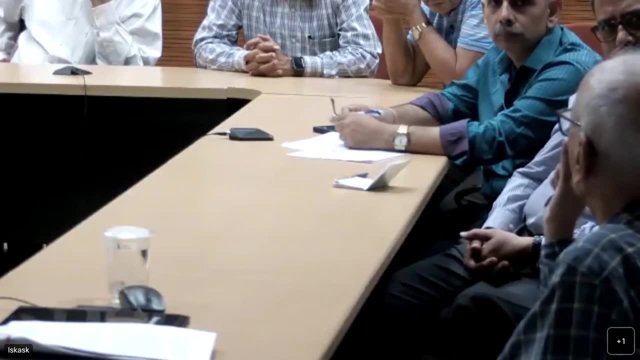 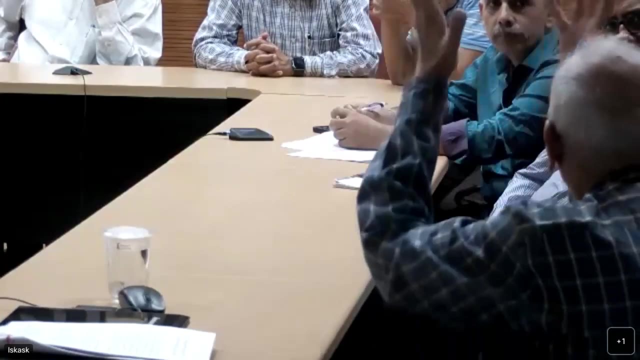 a quite complex. uh, they have to refuel up with that fast reactor once in six months or eight months like that. they have to do that and that is because it's a very heavy duty reactor as it is so very in a very small core. you are producing five members, so it requires that. 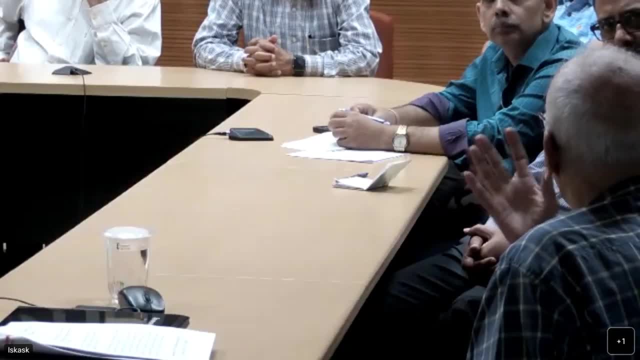 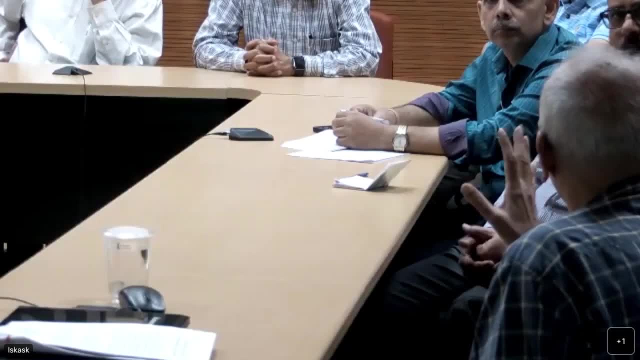 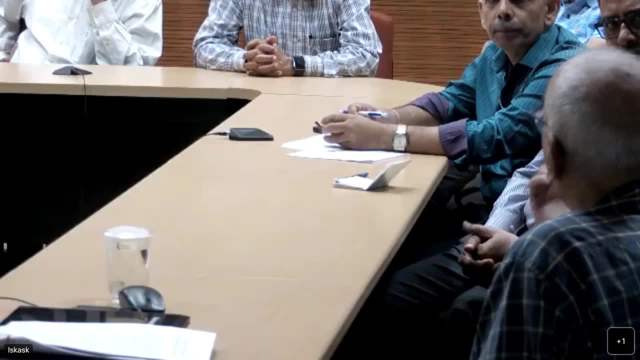 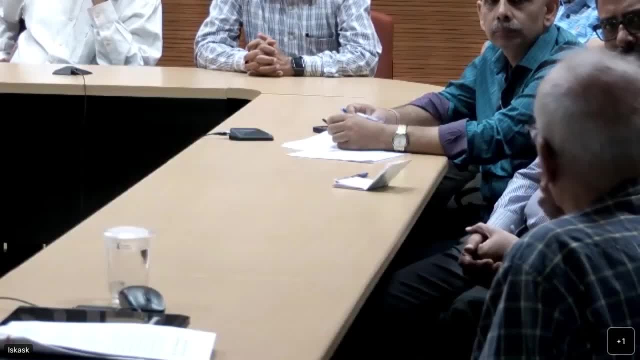 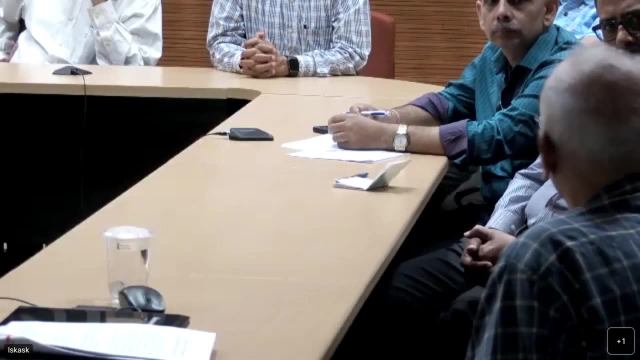 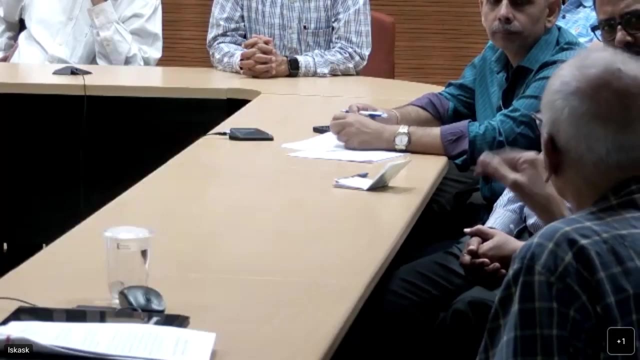 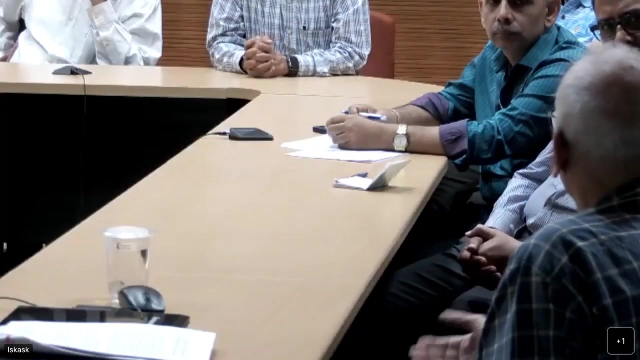 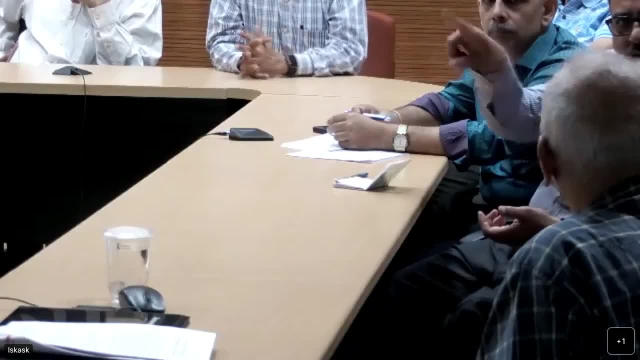 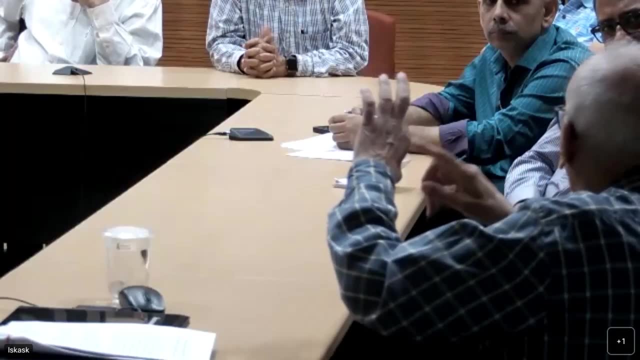 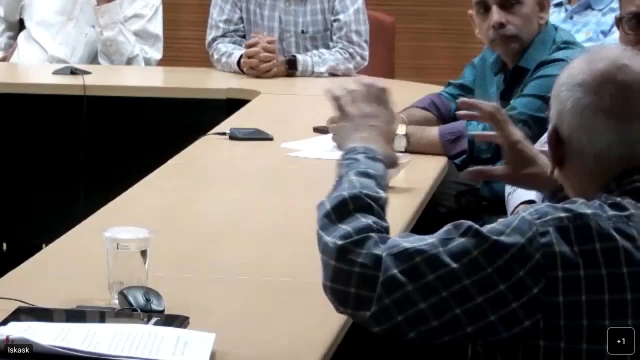 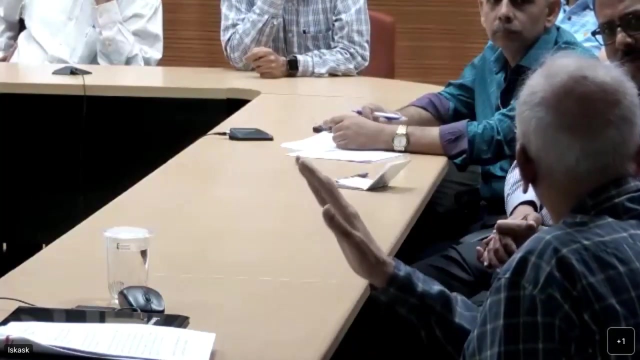 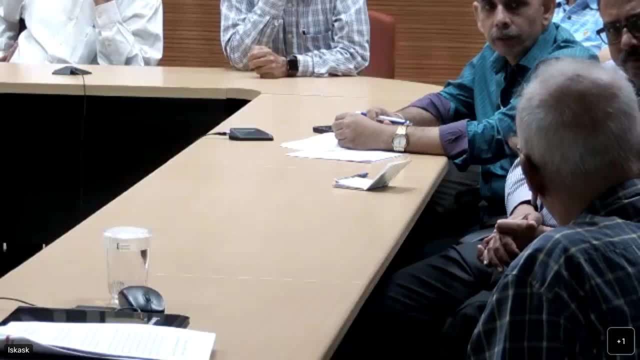 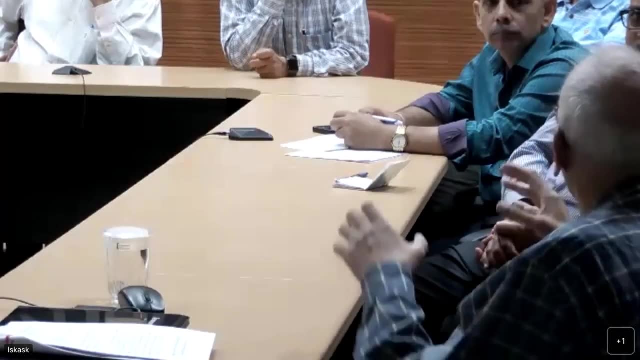 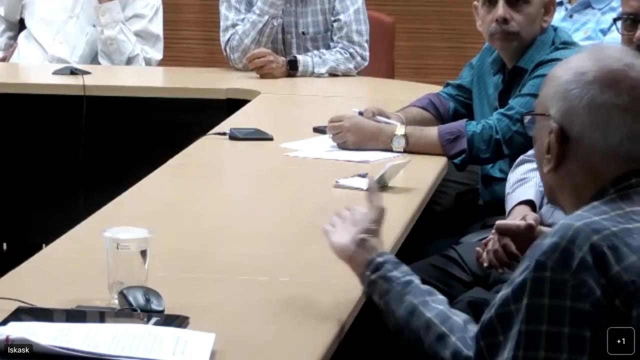 So even if there is a small, small bend, it will negotiate it, but it will. it is not necessary that it should have perfectly right, because it is like a train: you have links in between two carriages and you can take some amount up and down, not only curve, but up and down. 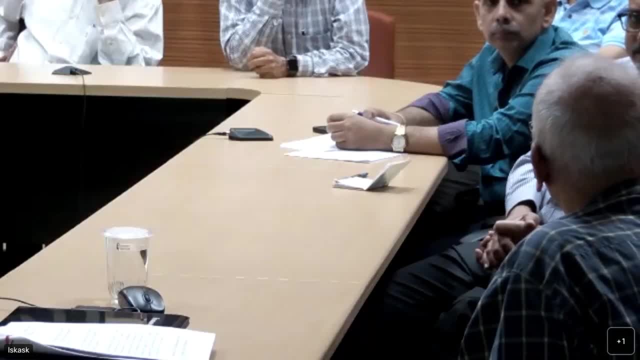 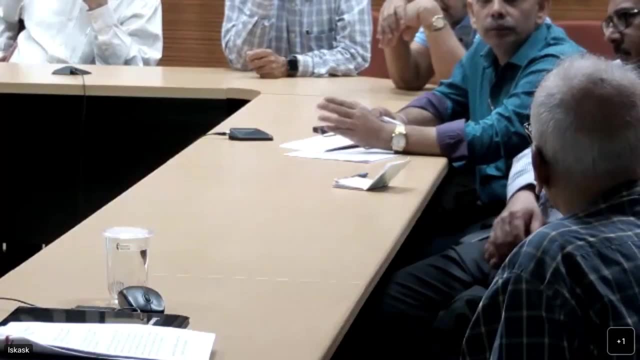 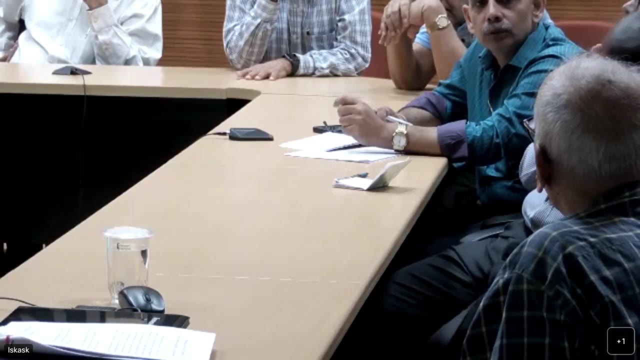 also it can take. So similarly it is here also. We were talking about the water lubricated ball bearing, oil lubricated ball bearing, but nowadays requirement has reached for there is no lubricant should be allowed because we want to have cavities in the vacuum here. ball screw should not have any lubricant. 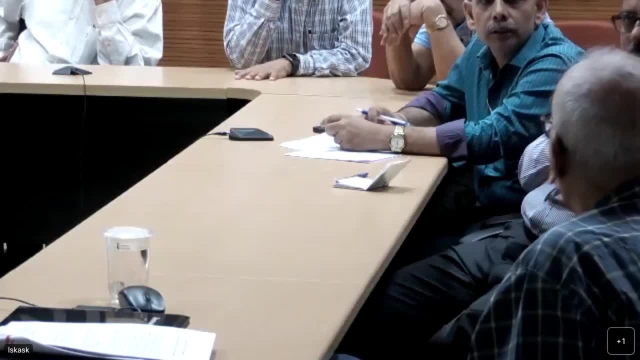 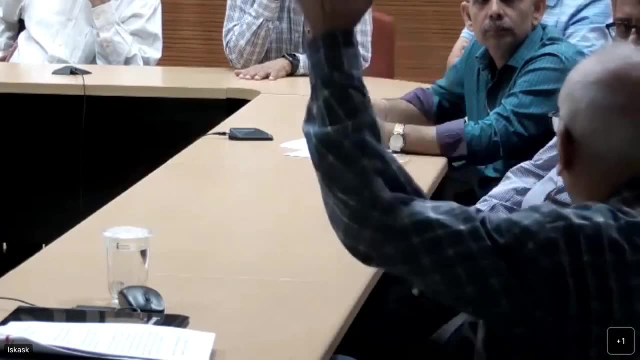 Vacuum means you cannot even have water. that is what you are saying. Actually, there is a material called molybdenum sulphide. I am just telling off the hat because you asked a question. I have to answer, right or wrong? 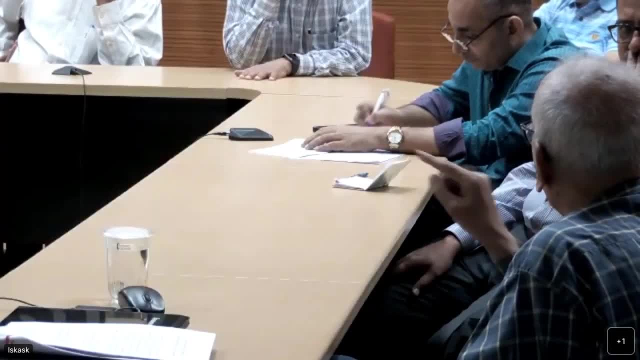 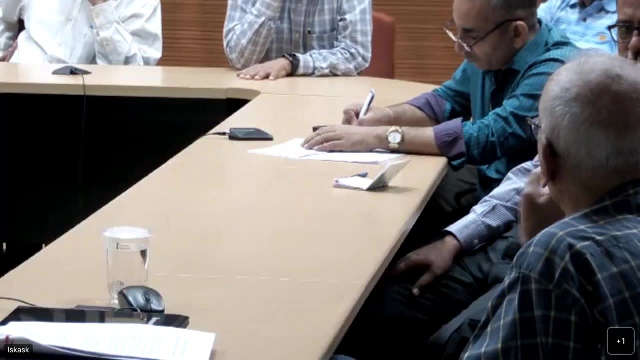 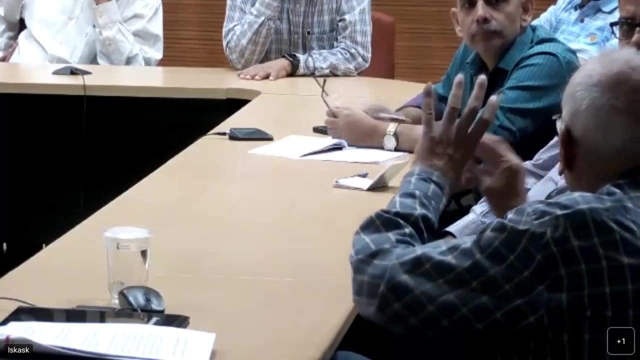 There is a material called molybdenum sulphide. that molybdenum sulphide can be coated. molybdenum sulphide is very good for low friction but ultimately any such bearing if you do not have lubrication and if you have not over designed- see where takes place because of 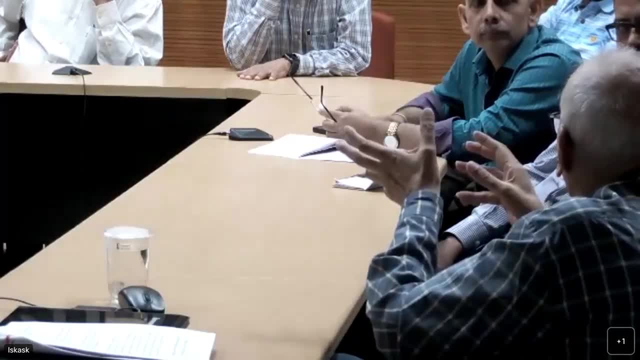 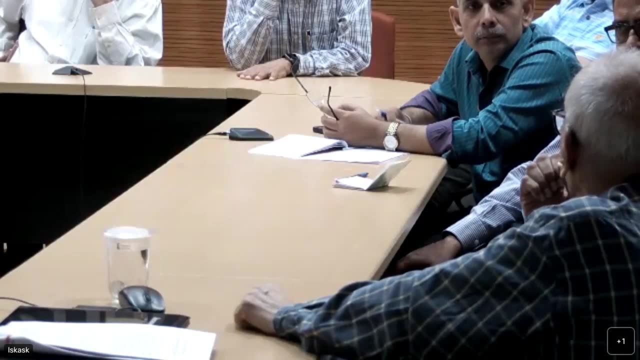 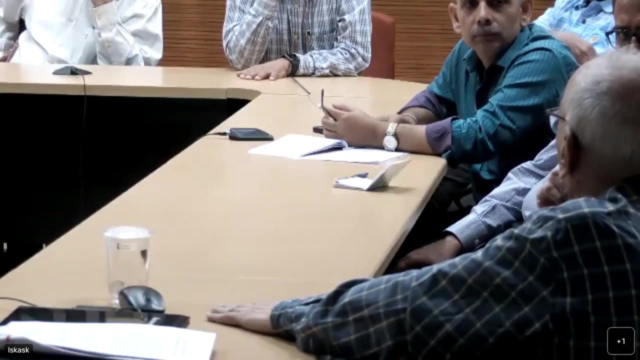 contactless. Okay, so if you have this ball bearing- and I do not know what it is, But if you do not have ball screw length per minute, okay, anyway, not. what is the ball nut? that ball nut that is rotating now. what is the speed of that? 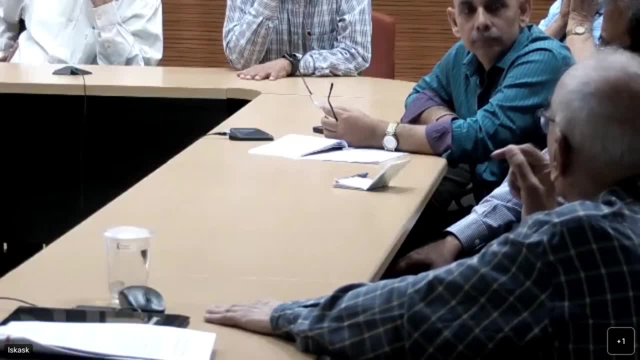 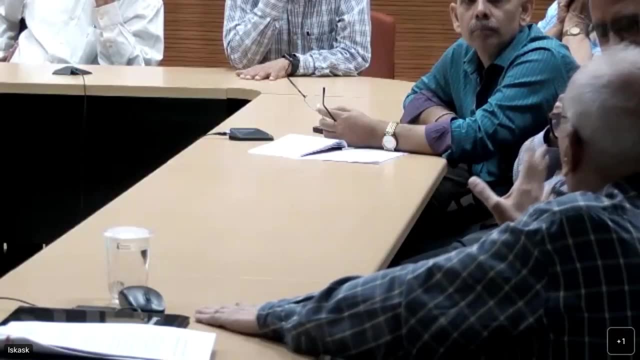 That is, that is what is important. speed of that RPM is important. Now we put molybdenum sulphide coating on that you can reduce wear. But I would say that in vacuums, That in vacuum system, if you are going to have drive like this, ball bearing, ball bearing. 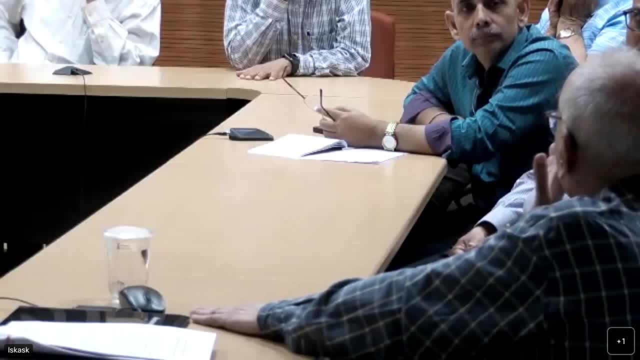 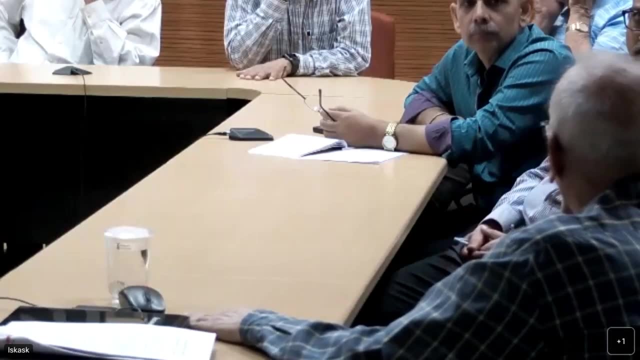 or ball screw or small screw you're having. you make it in such a way that it easily replaceable. one dot, that is what is important. Don't put it somewhere and then say 30 years I will not touch it. That is not a good idea. 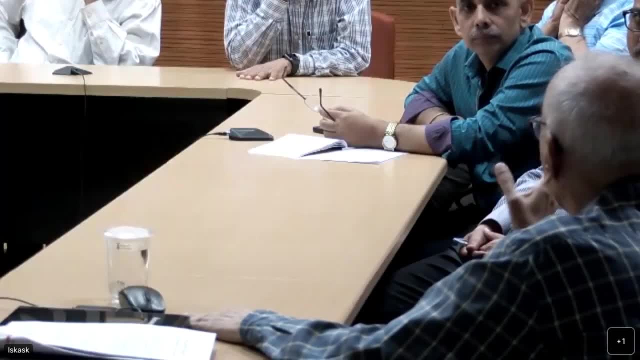 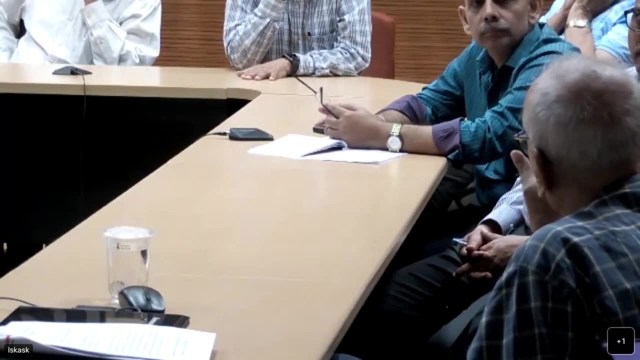 Anything should be maintainable. maintenance, you must take care of it. I think molybdenum sulphide, sulphide will do. then yeah, I don't know how loading is that? there is something called a delrin material ball. So if you put that that is a phenolic material. 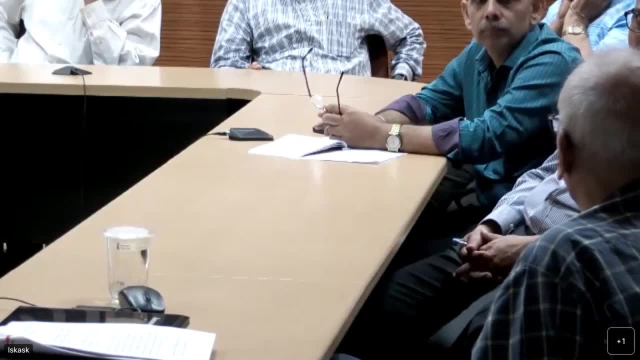 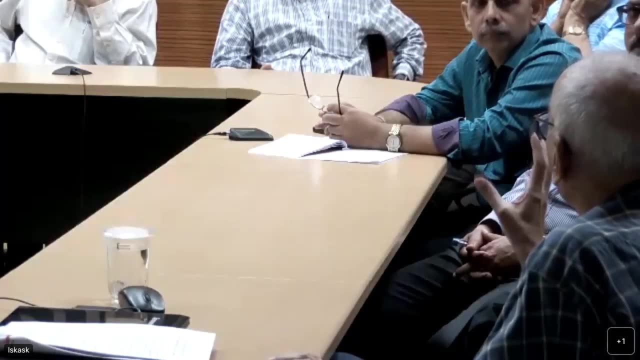 It will not take too much load, but it will not give you friction. So you can use that. and then the other method I told you: between two balls you put the delrin ball. that will reduce also. So there are methods available for reducing friction. 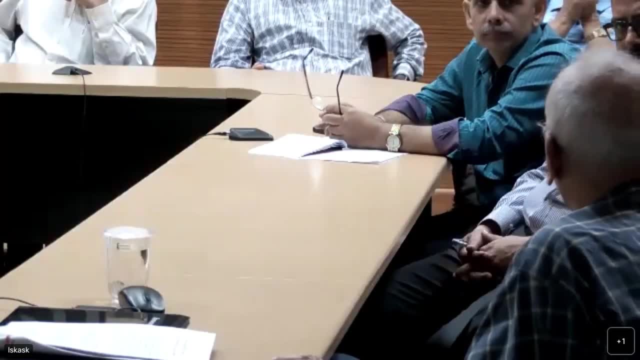 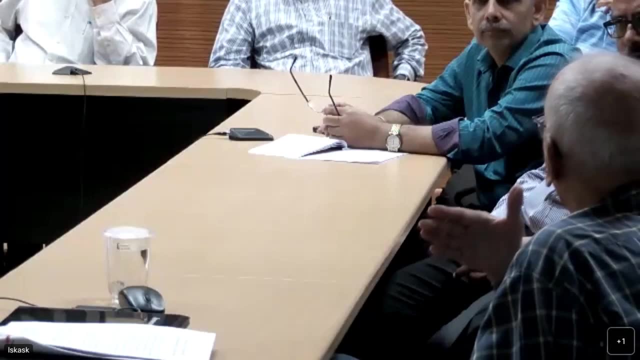 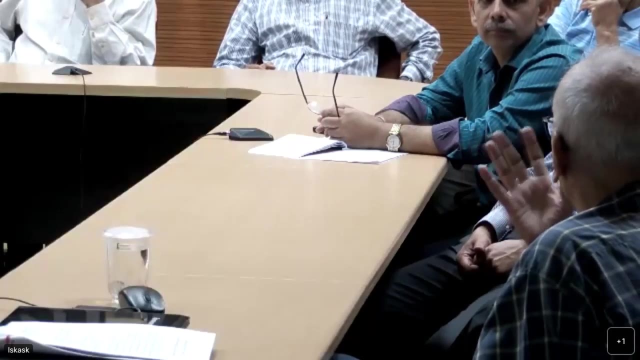 Ultimately you have to make one and test it, Otherwise there is no very important. you have to test it. ACL have done it. tremendous amount of testing. the ball screw originally they had for BRAM was in fact made by a rolling process By Saginaw steering here, which is no good. 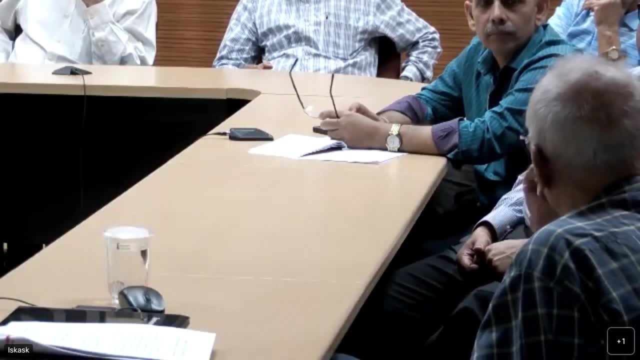 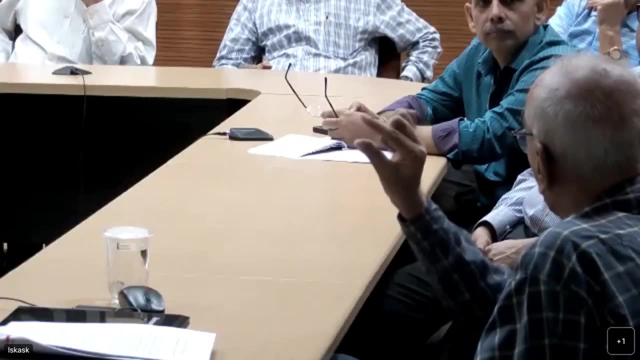 We are now grinding, which is for much better finish, much better accuracy, much better tolerance. in India, all the ball screws, And in other words the ball screw is also hollow. So we this experience I will tell you once we got the ball screw from Saginaw steering. 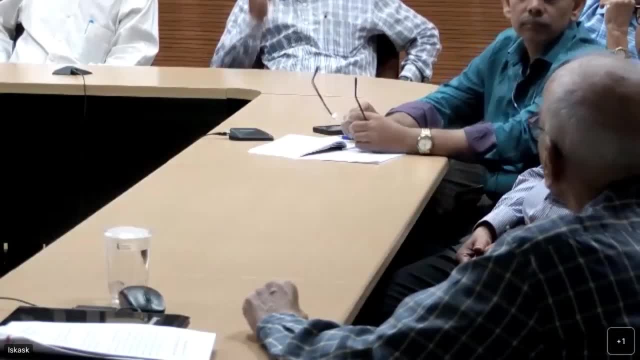 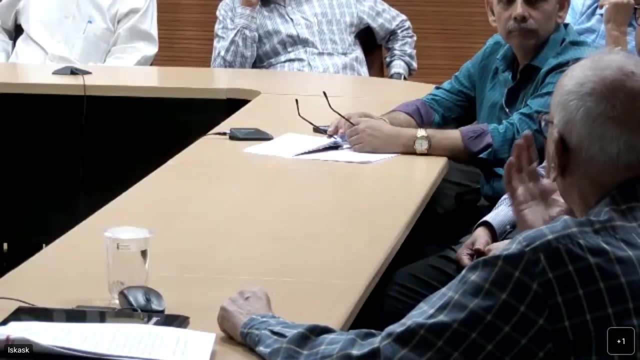 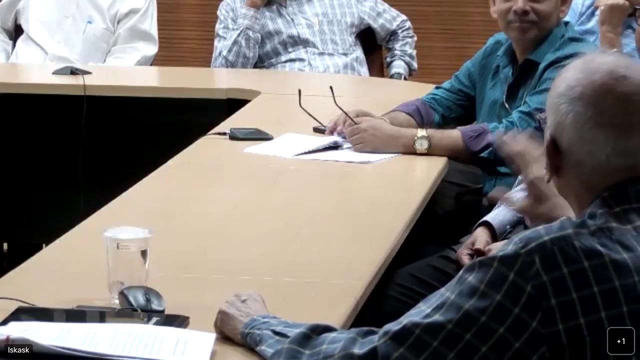 gear. earlier then Central Road shops started machining. they started putting the inside tube. You know how, How machine, how manufacturers are. they're always very happy to pounce on the designer, and I was the designer, Central Road shop manufacturing. is that why your ball screw is all no good? 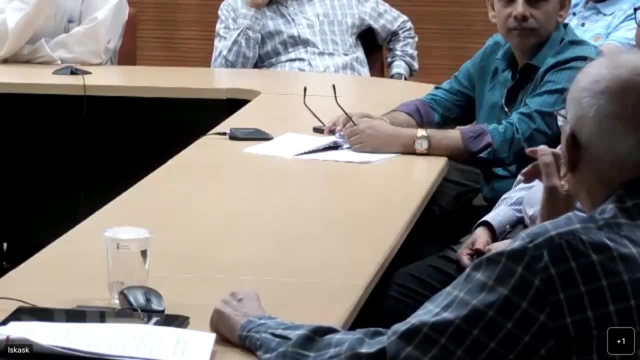 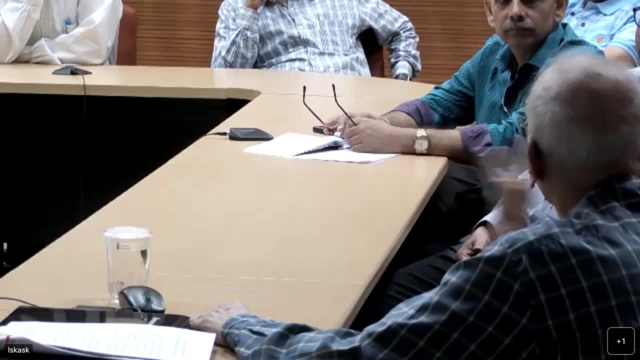 My cube is not going. I'm not able to put the cube inside. Then we thought, we thought of thought we've got to troubleshoot. we started measuring and finding out. I was saying you will let us hone that tube and then the errors will go away. 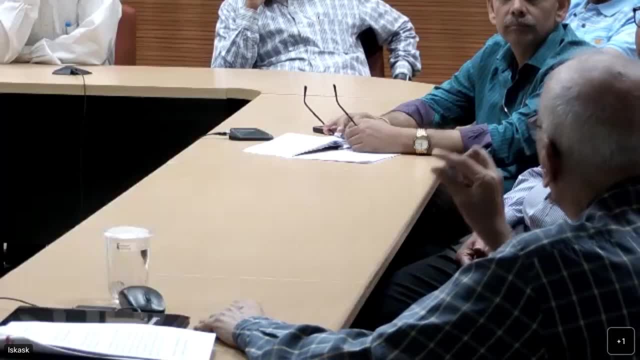 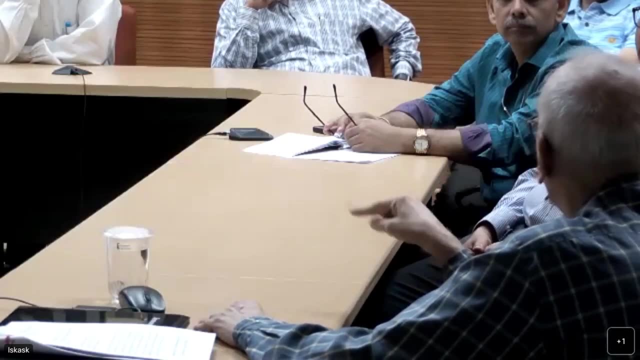 Ultimately, what had happened is The manufacturer of the ball screw had taken a tube and then rolled the thread. So the rolled thread, when he rolled the outside of the thread, it produces a ridge on the inside, which was stopping this fellow from going. 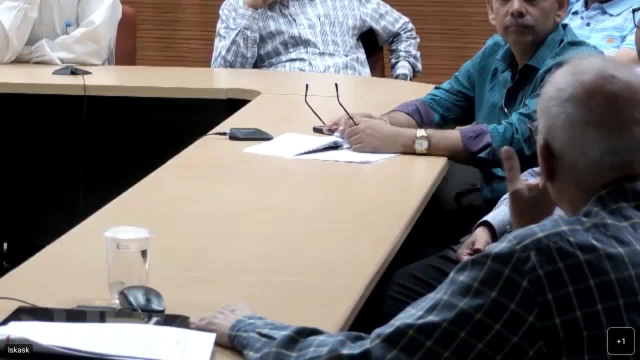 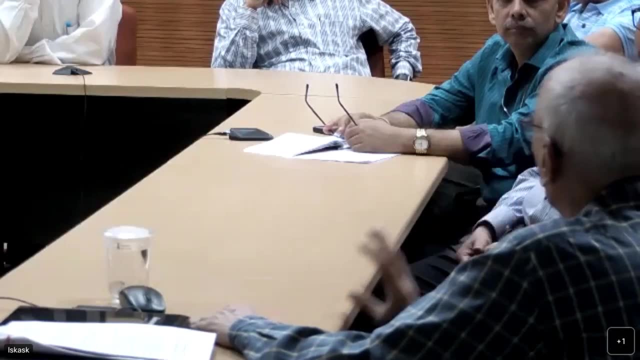 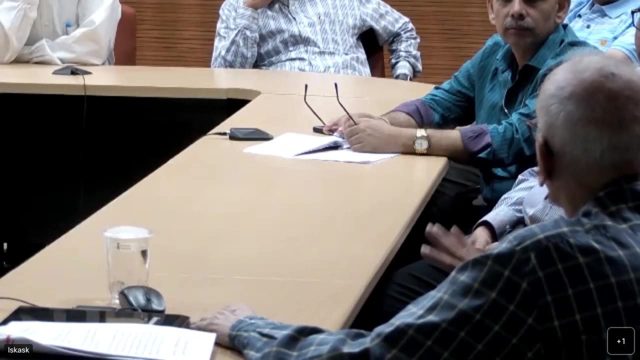 So now I what our people are doing. they're grinding. grinding means you're not putting so much force on the thread machine. So our, to some extent, that 200 channels refueling to changing to 700 channels is a good progress. I hope it will come, incidentally, 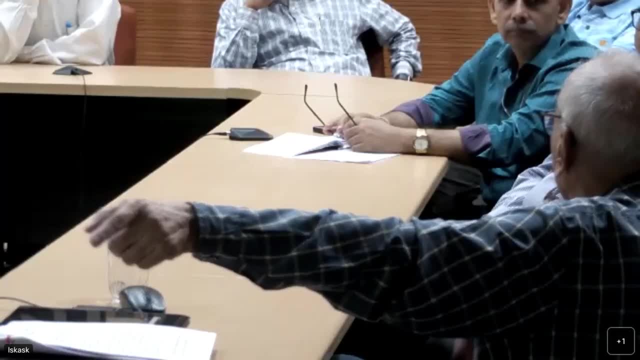 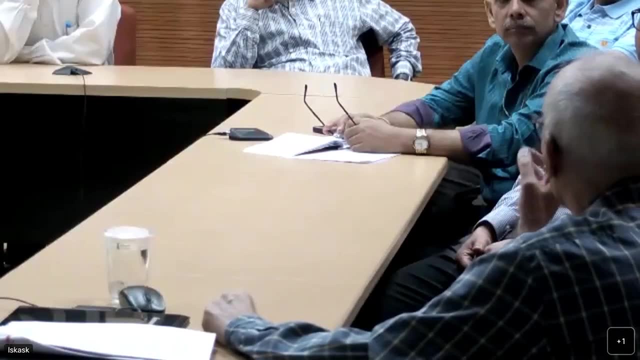 I wanted to tell you they forgot this- Tarapore 3 and 4 fueling machines, as of today, as of yesterday that is, have done more than Tarapore 3 and 4 put together, have done more than 15,100 channels refueling on power. 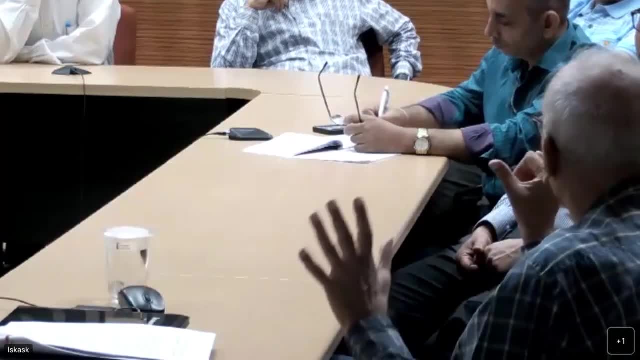 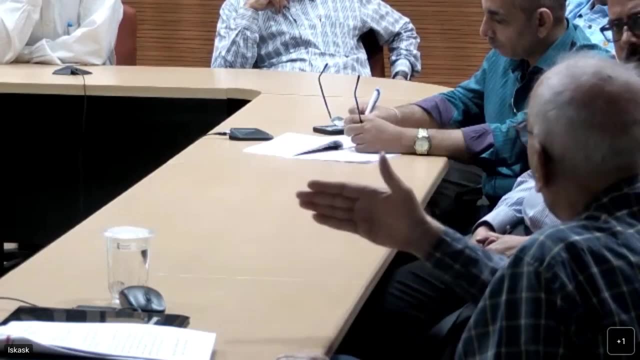 So each reactor, 7500 channels. they have done. it is rack and pinion. I am told they have not changed the rack and pinion at all. If you take rack and pinion as an equivalent of that, As an equivalent of the ball screw. 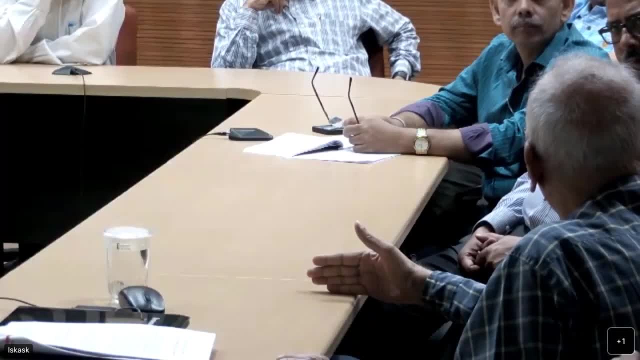 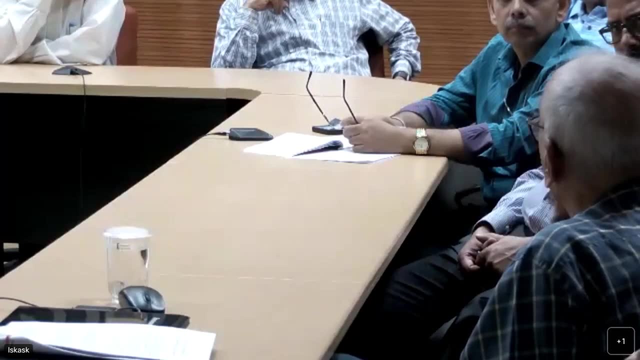 They have said that they are not reaching. They have not replaced the rack and pinion. The reason is the rack and pinion is over designed. We have. we did not know what is the stress that should be under time 1985, when we were. 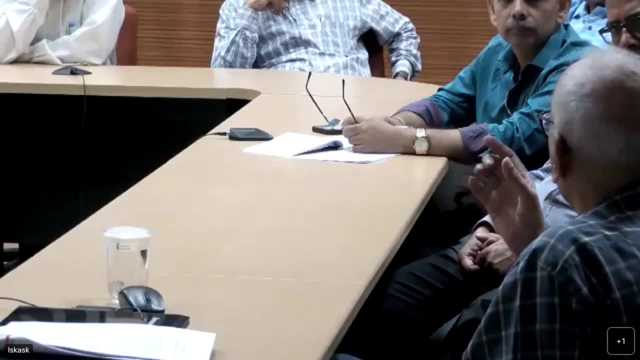 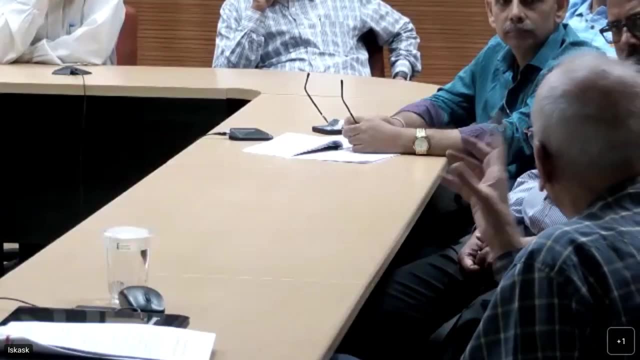 doing. We did not know, So we were very conservative in the design. The width of the pinion is very wide, It is hard and the speeds are low. The contact stresses are very low. We have kept it like that And therefore. 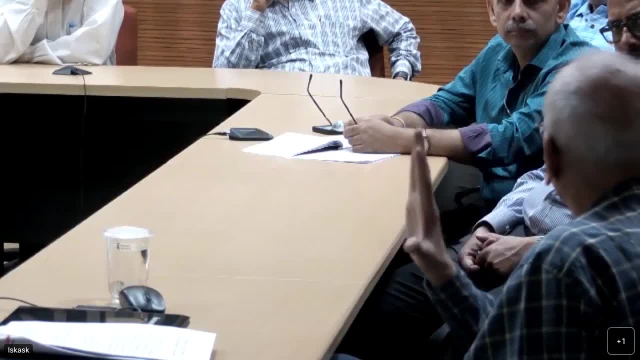 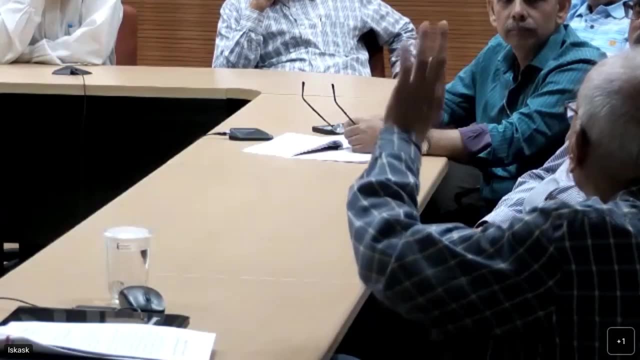 Up to now We cannot change. And one more very interesting point about that rack and pinion design is that in the whole system, The entire ram has to give the maximum force, which is 3000 kg maximum force, at only one point, that is, to operate the ceiling. 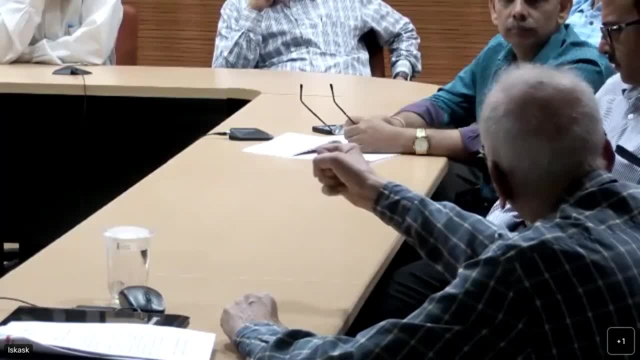 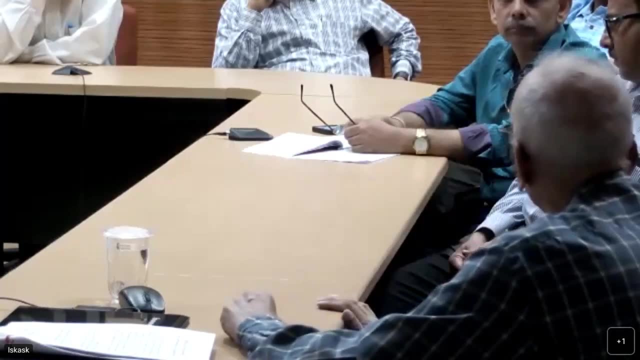 It is only one point. Ultimately, if you see, it is only one tooth, Only one tooth in the entire system that is taking that maximum load. Otherwise, it is all fair enough. Everything is plenty. So the rack and pinion design has been made. 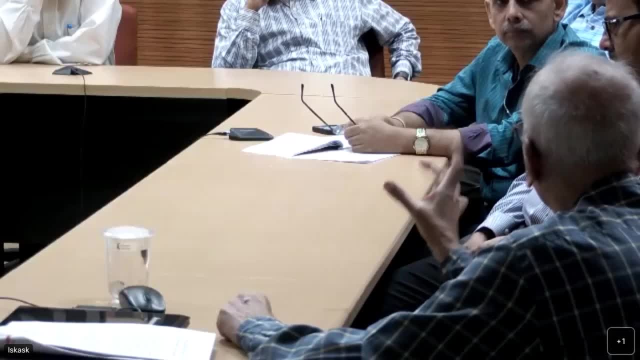 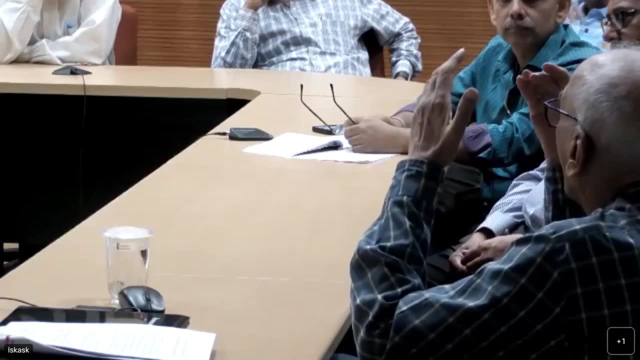 And that individual sections can be replaced. If it becomes one that it is can be replaced ground, put it into work. So that is the design that we have done, But see what we have to sacrifice on account of these design. changes in the machine has. 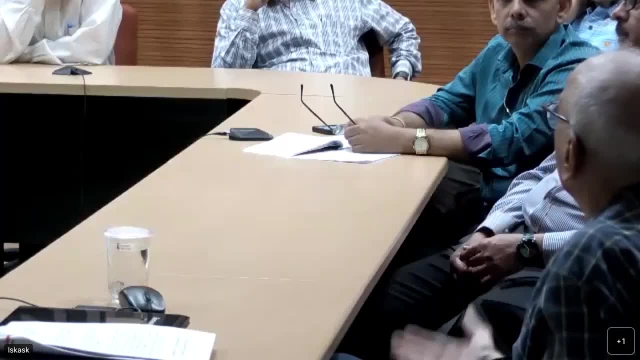 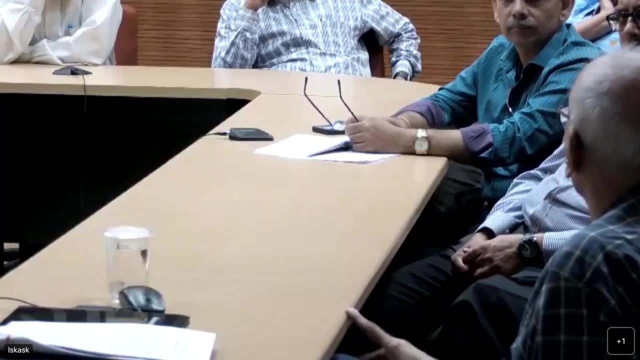 become very long. It has become a little bit more long, But the site have accepted it. So to that extent I am thankful, because that is what it is: The rack and pinion. that is what is the story. It is what it is. 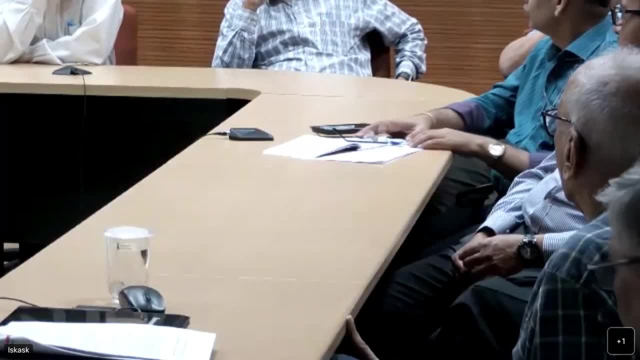 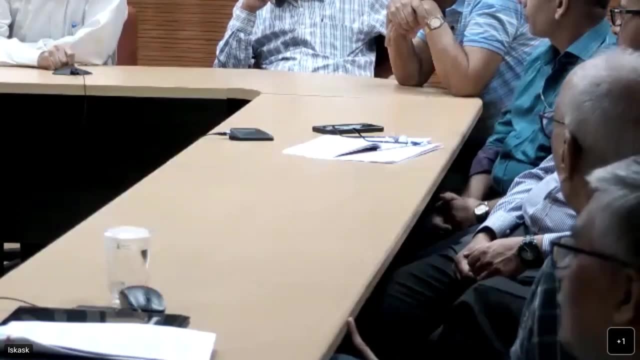 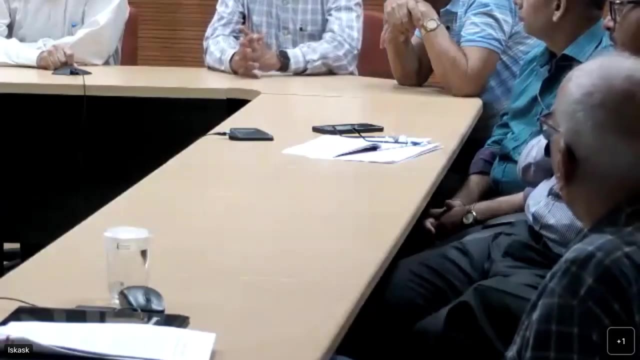 It is what it is. So it is what it is. It is what it is. It is what it is. Well, we come to the end of the lectures and discussions And I must say this was something which tells us how all practical things are interdisciplinary. 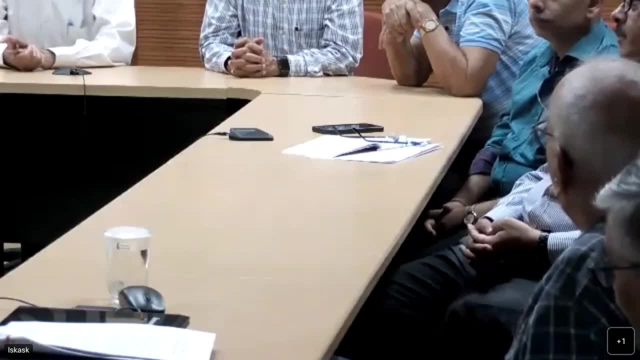 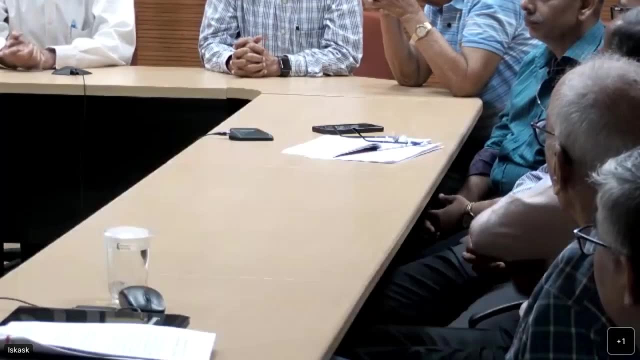 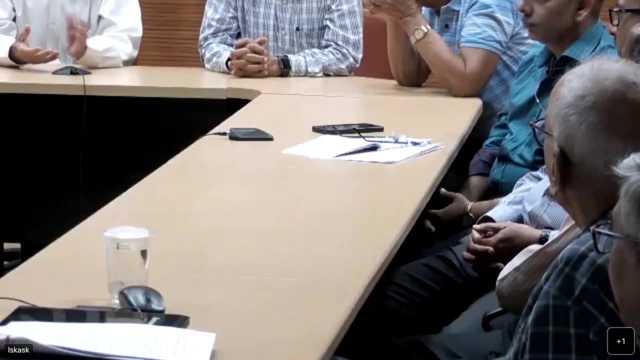 and knowledge of all the subjects goes into a machine of this kind, And that also makes us feel that how pioneer Pioneers in the Department of Public Energy have brought the total program to this level, based on which now, I think, the 700 megawatt is working at 60% and very soon we'll go to 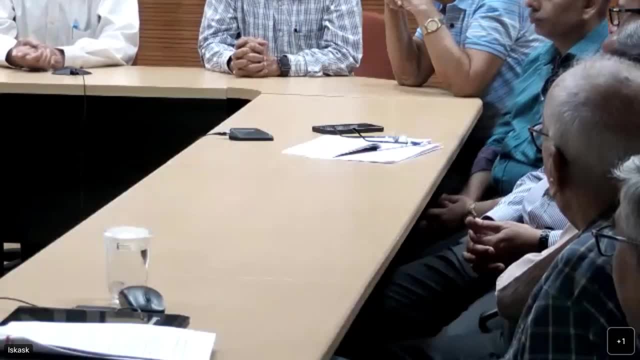 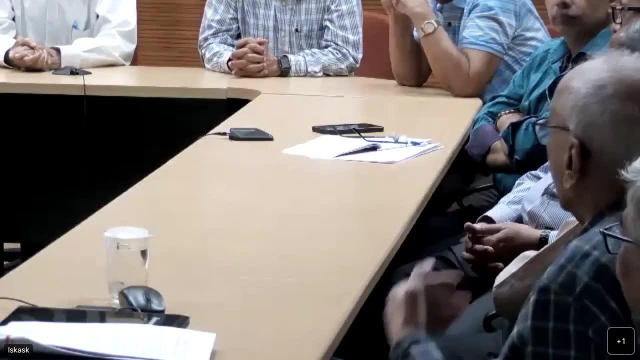 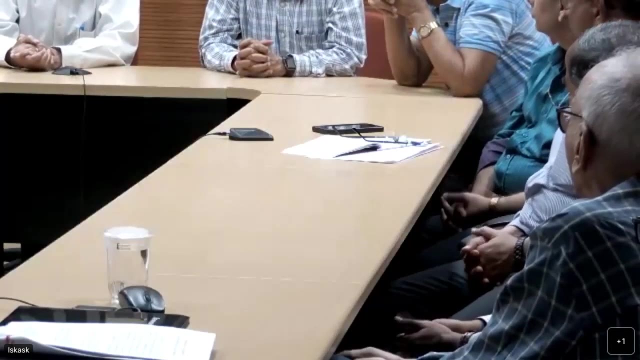 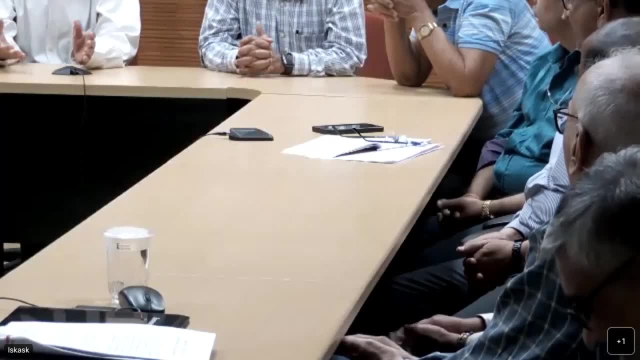 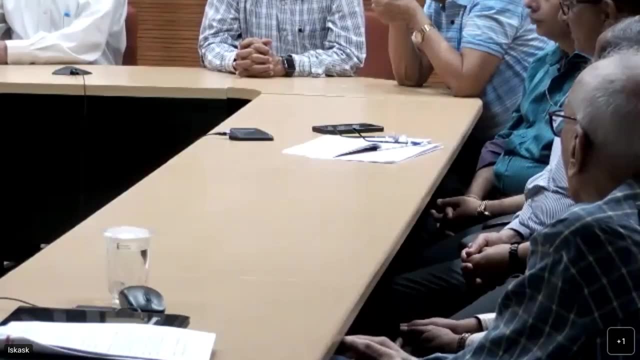 Thank you. Thank you, Sanath Kumar. Sir said that anything is possible. That is something which should motivate all the youngsters to carry on the program further And, on behalf of the local chapter of INAE, would you like to Thank you?